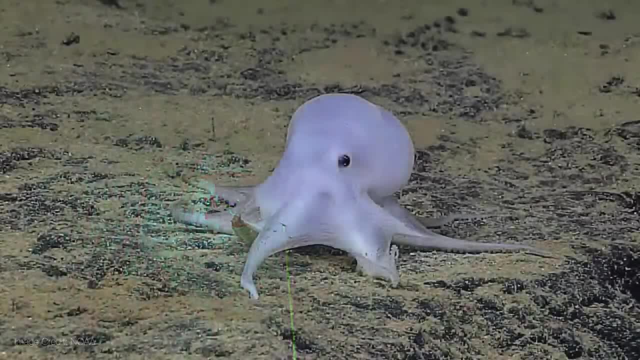 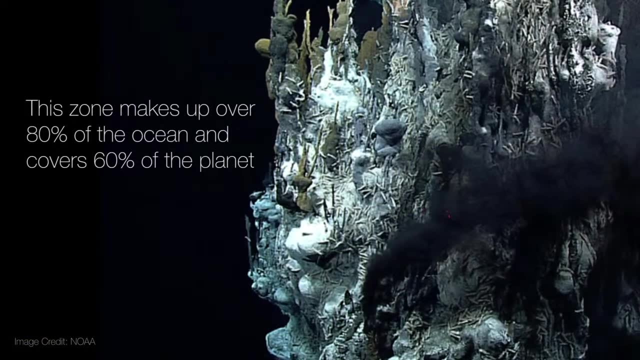 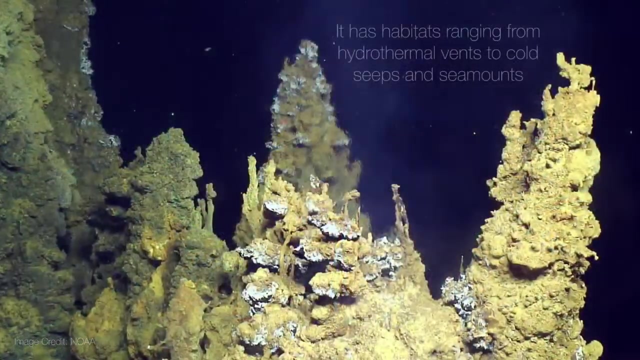 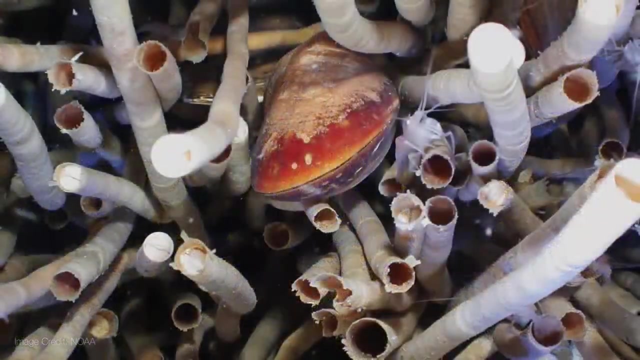 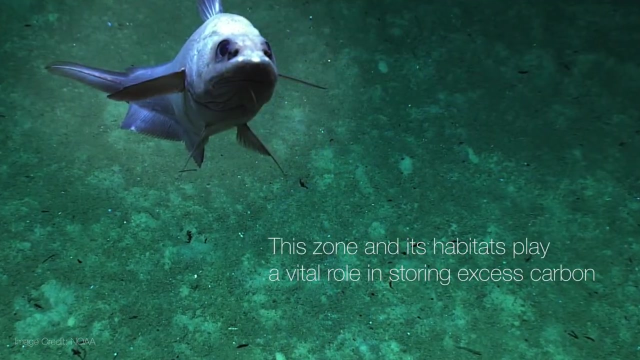 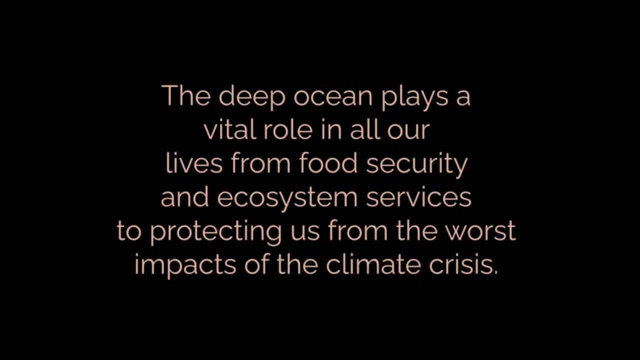 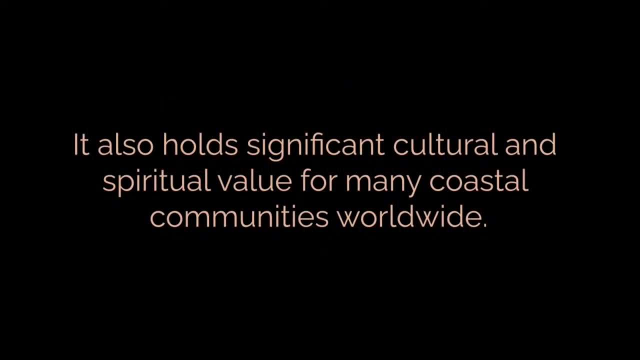 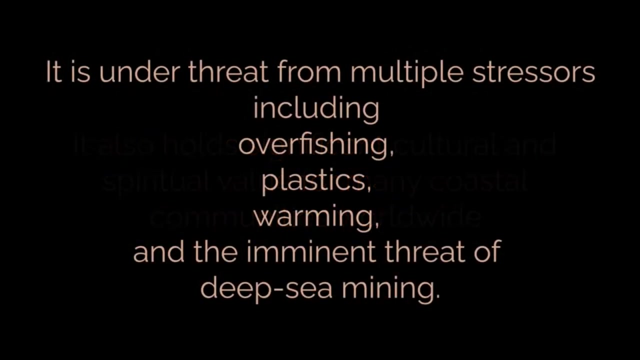 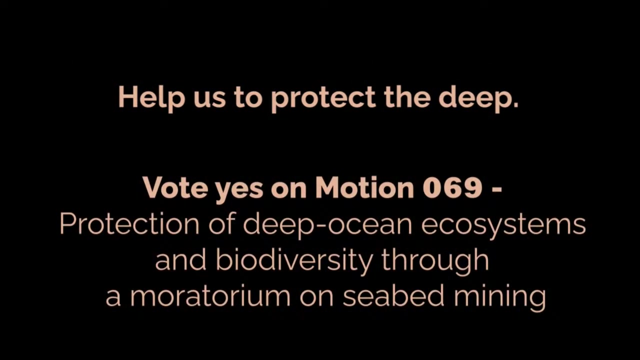 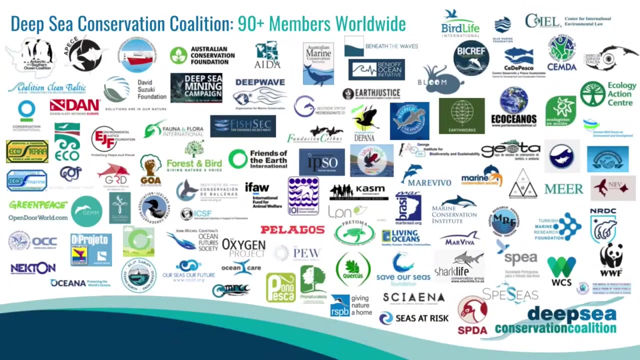 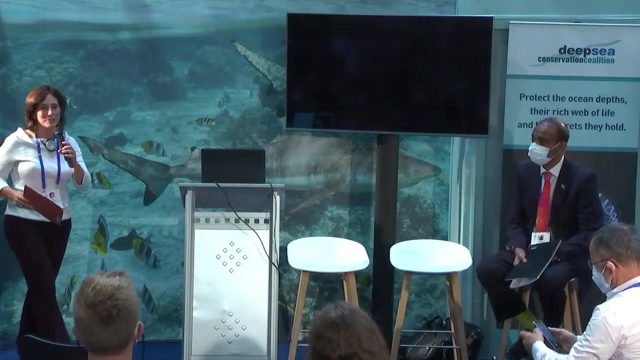 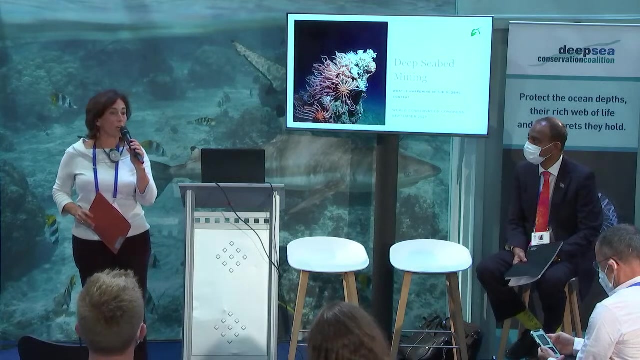 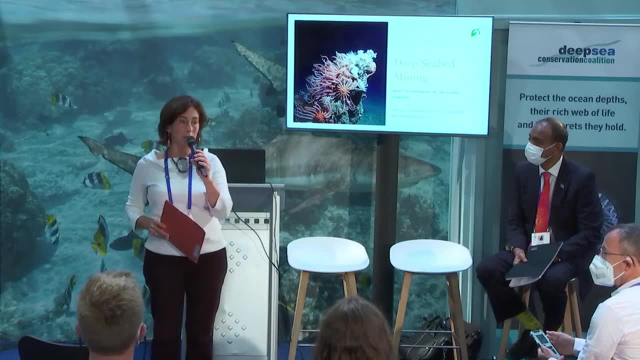 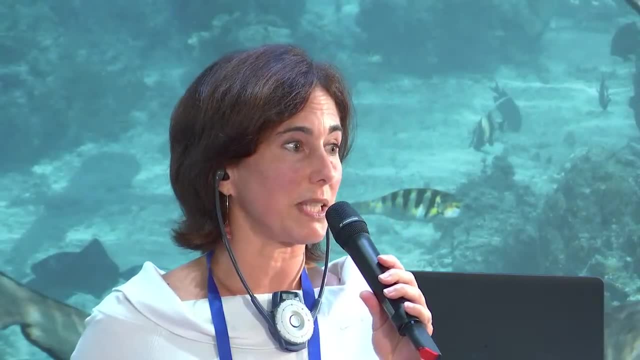 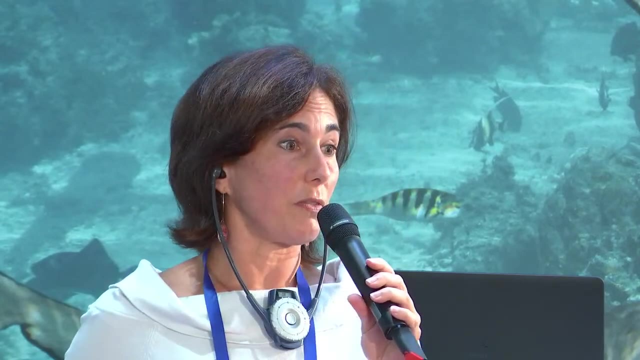 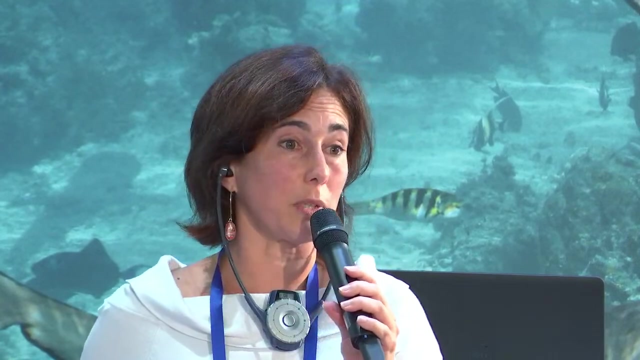 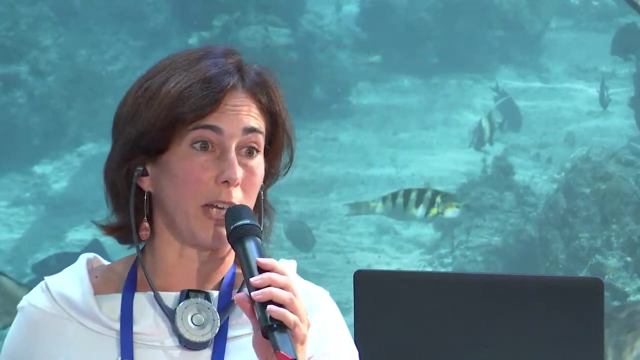 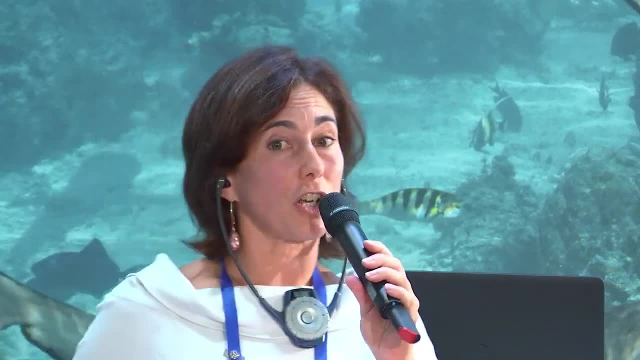 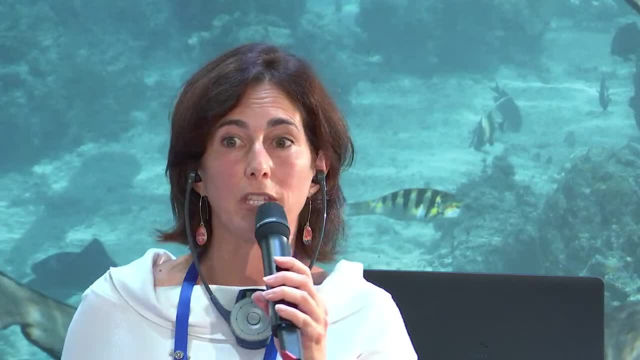 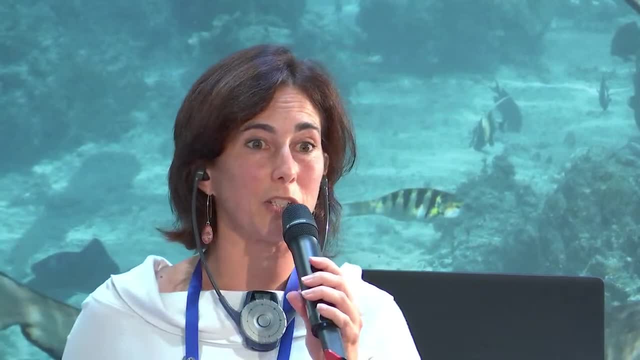 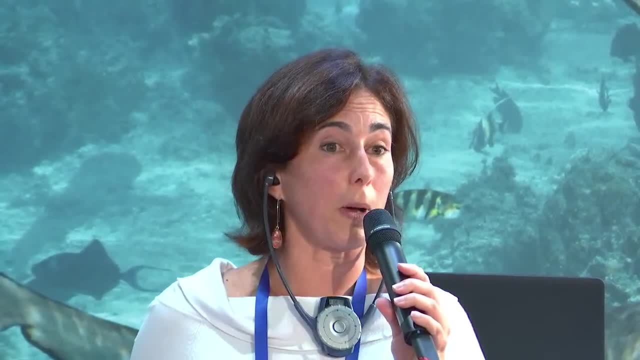 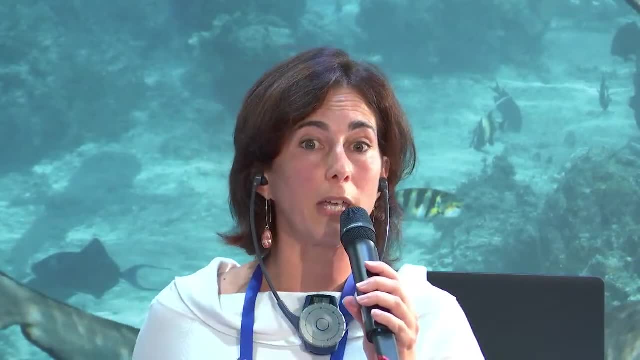 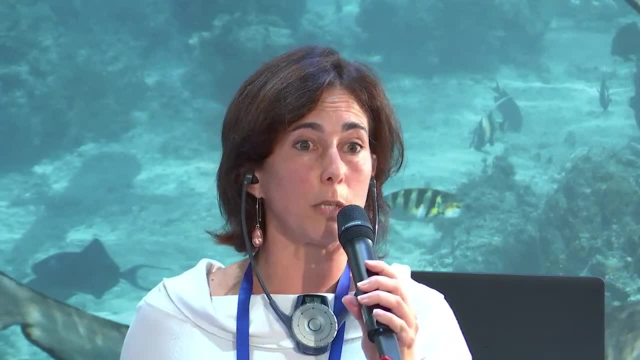 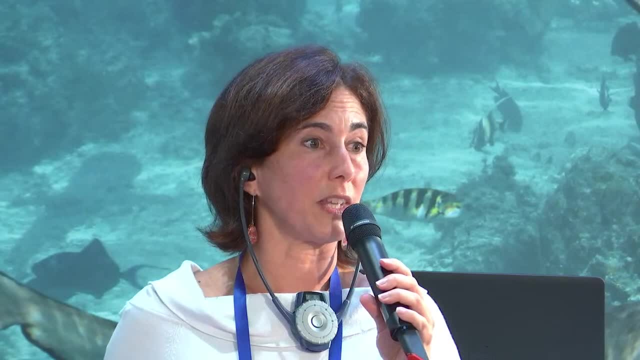 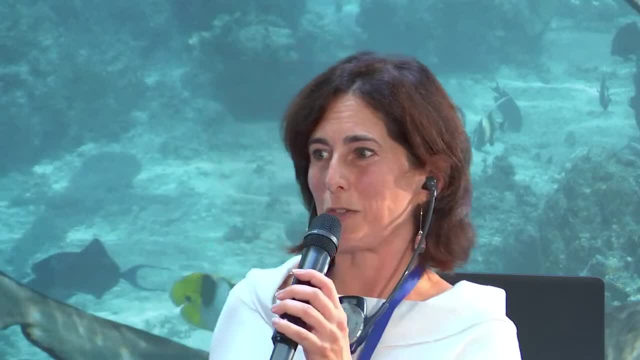 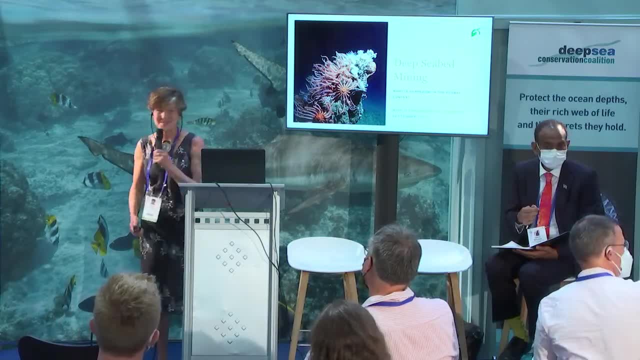 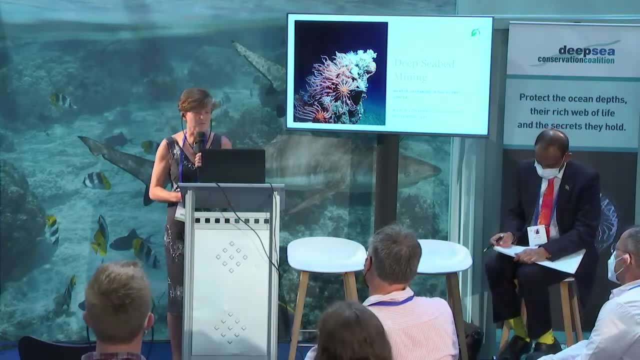 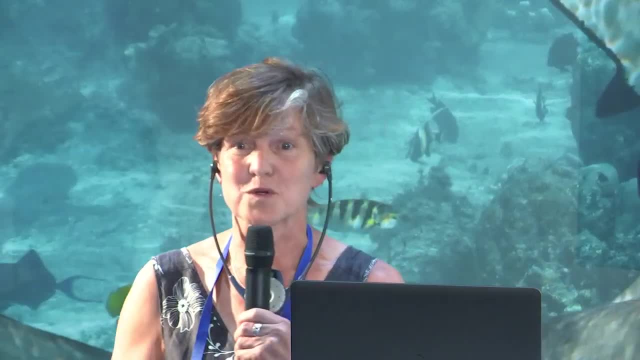 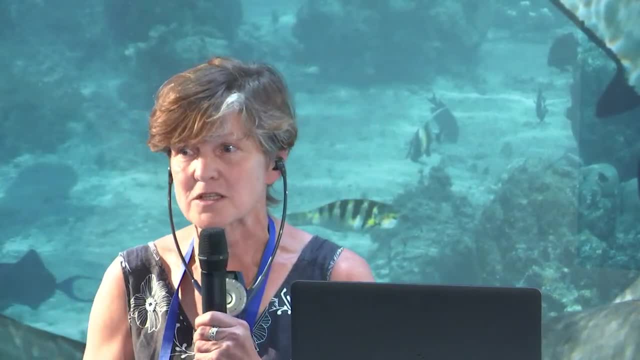 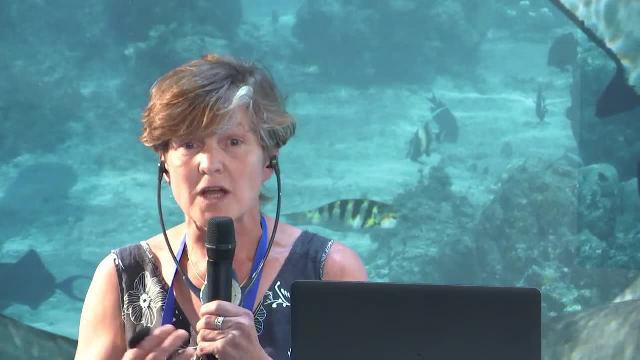 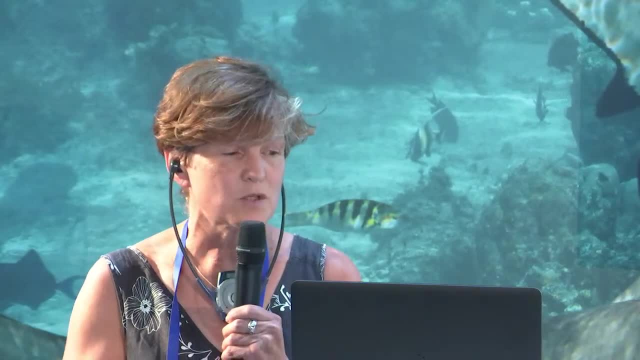 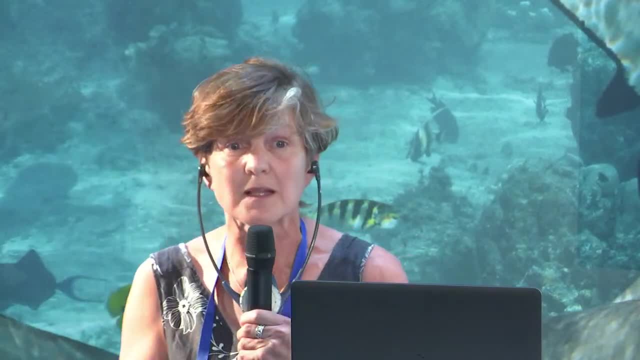 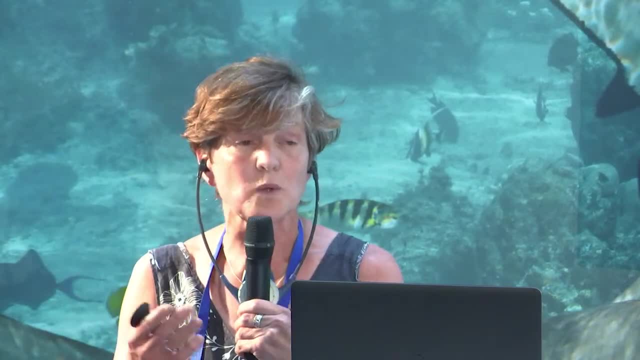 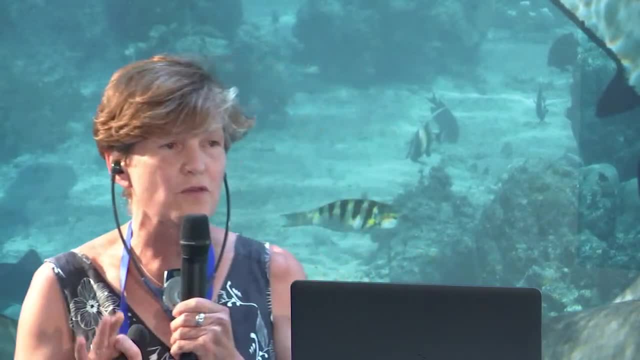 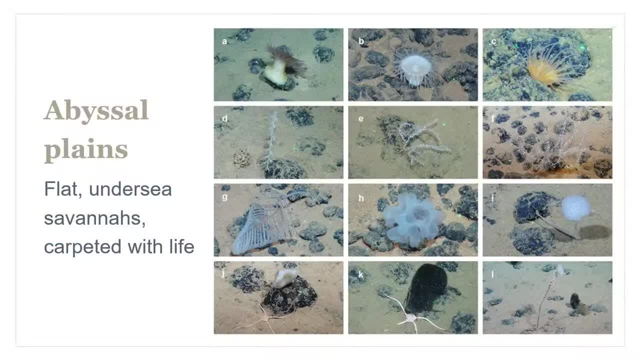 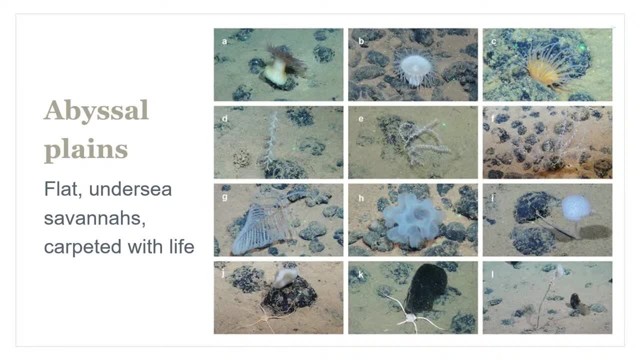 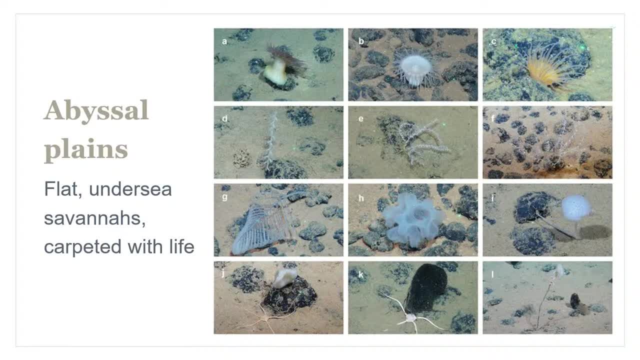 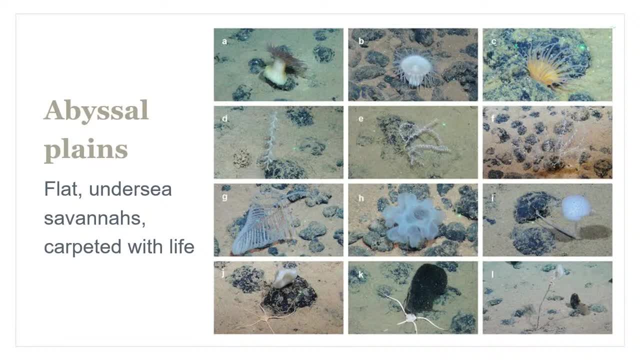 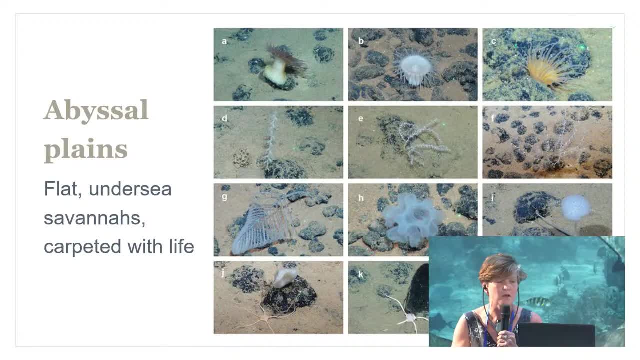 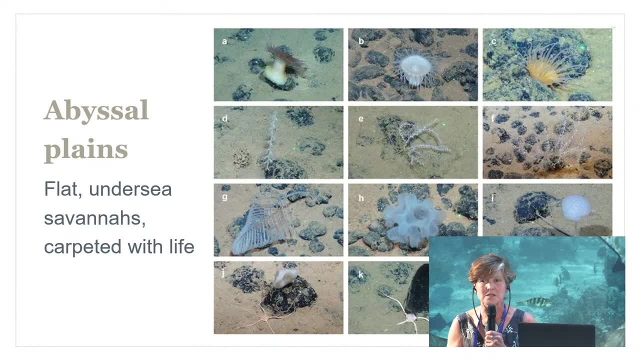 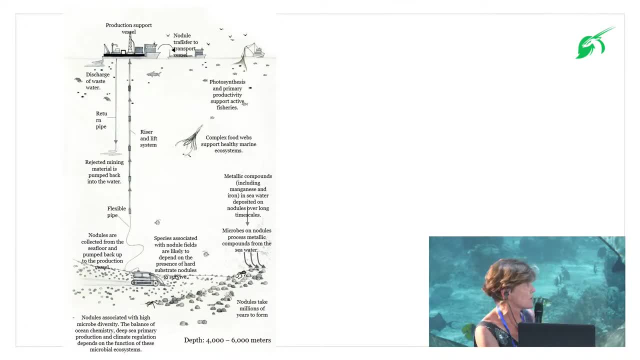 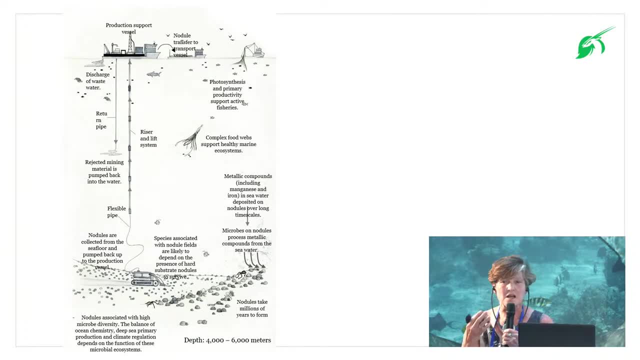 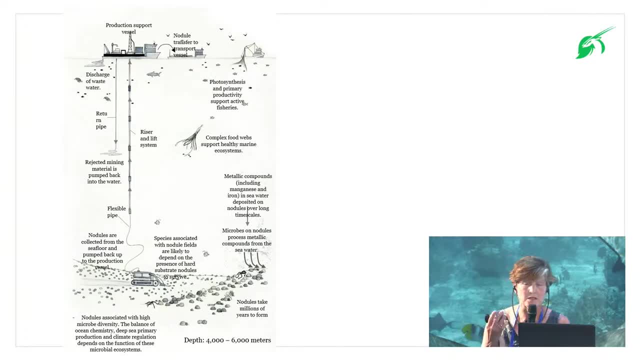 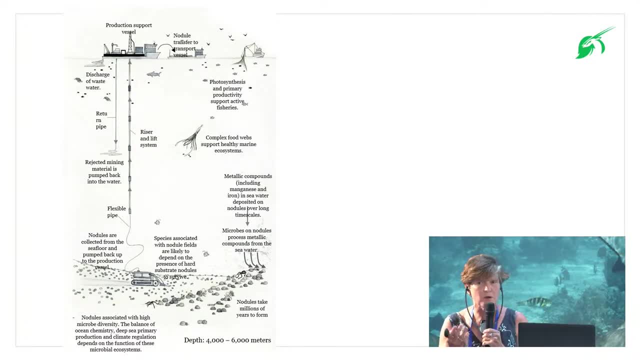 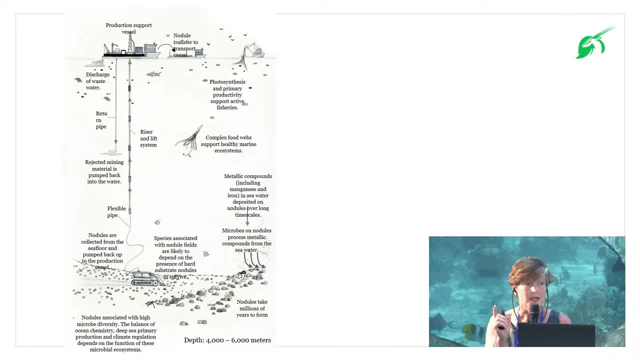 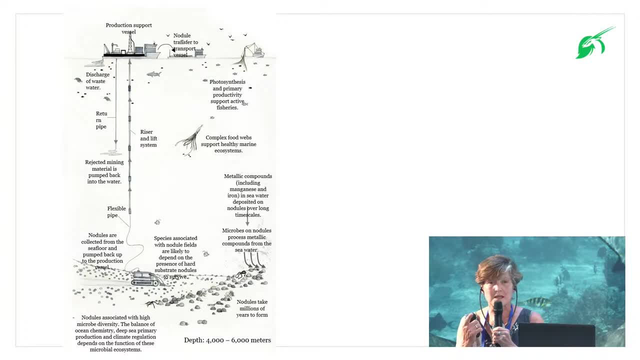 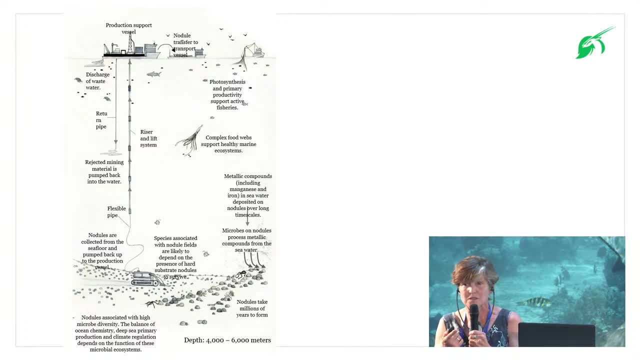 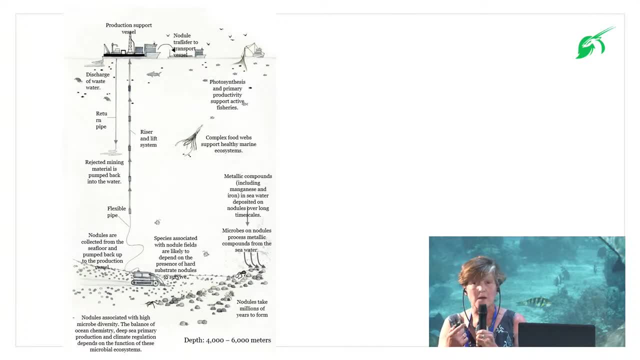 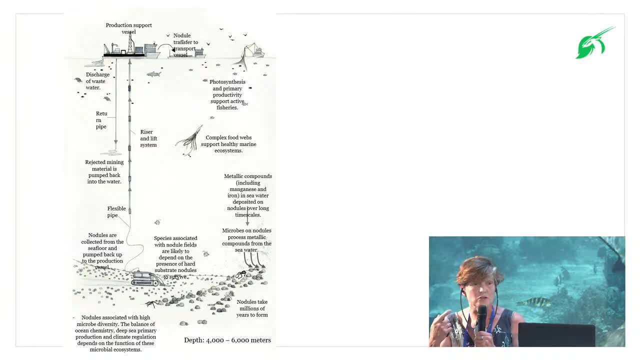 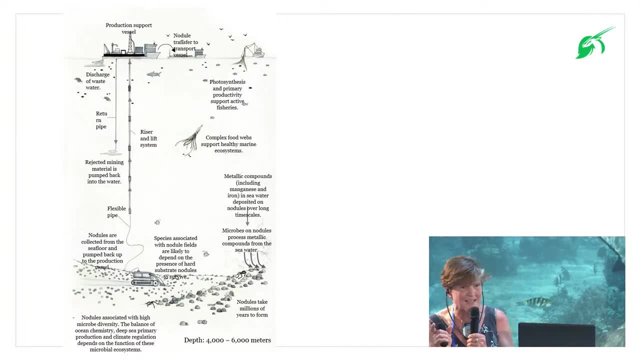 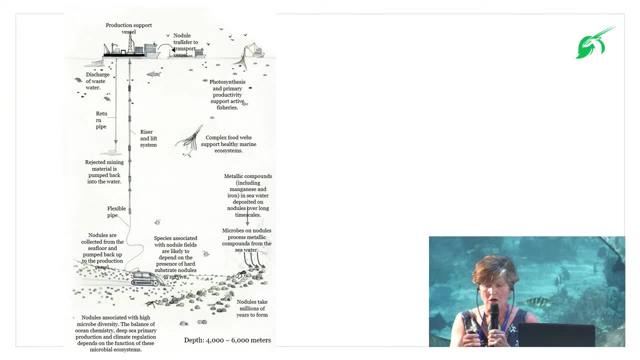 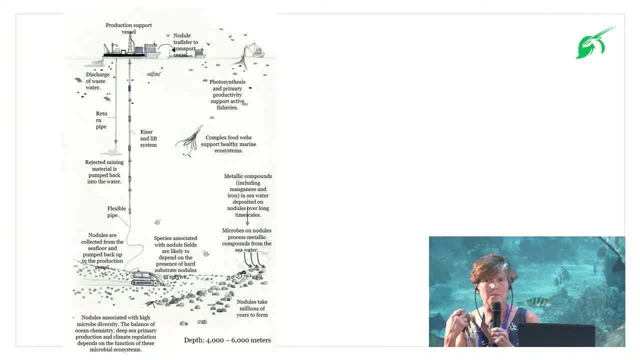 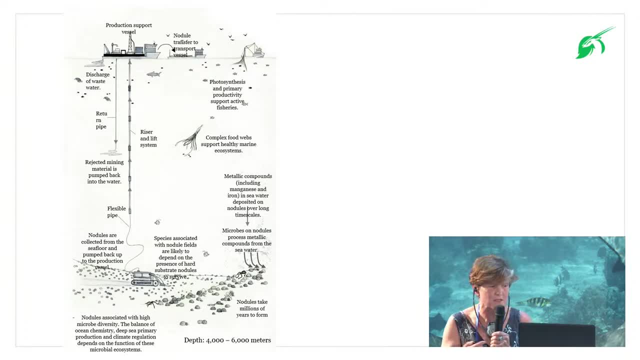 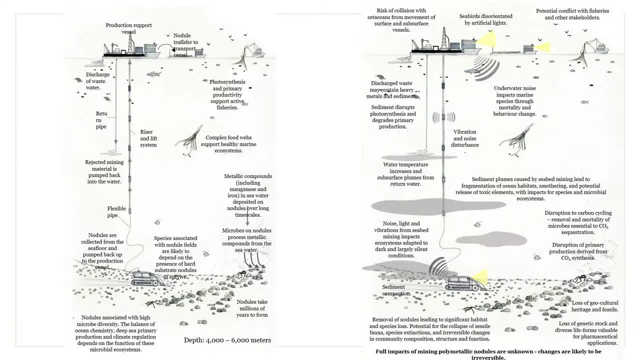 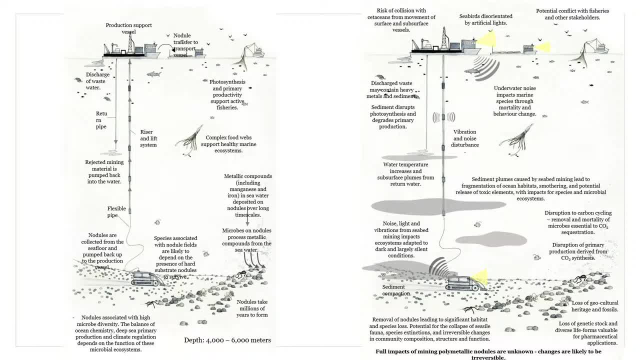 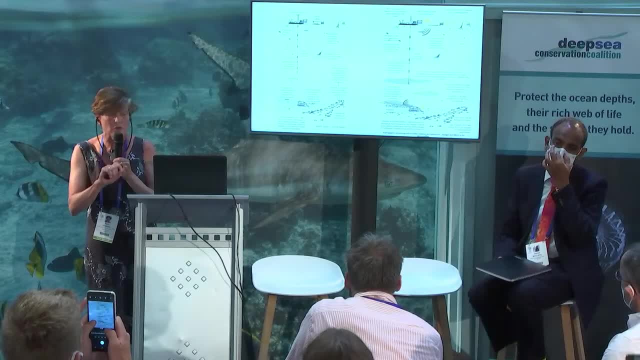 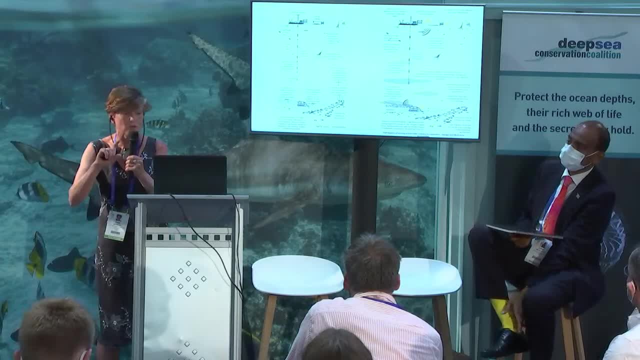 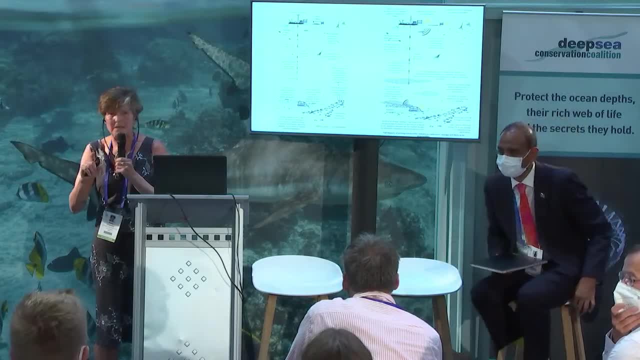 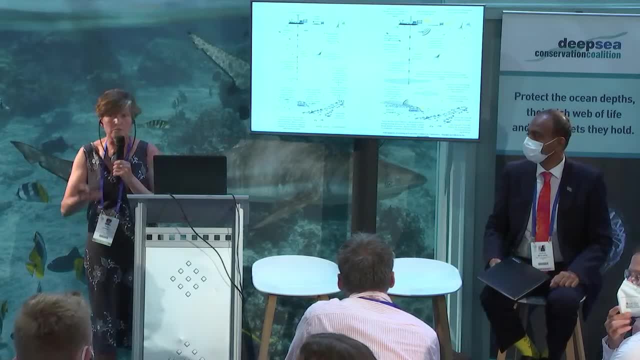 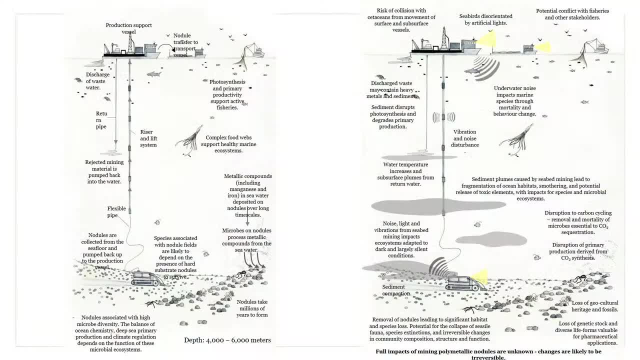 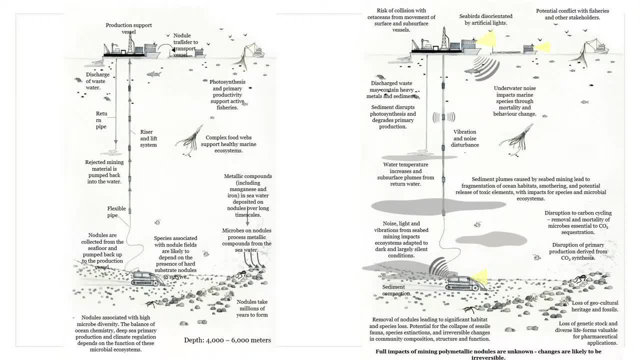 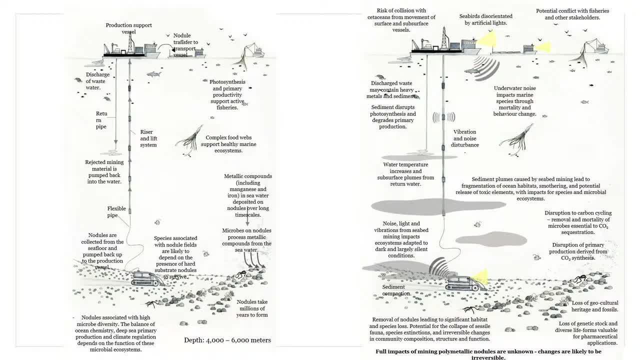 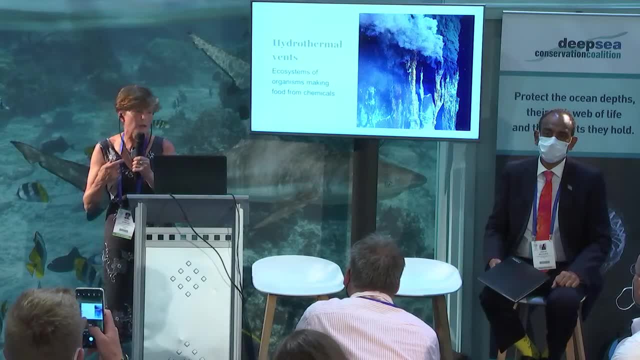 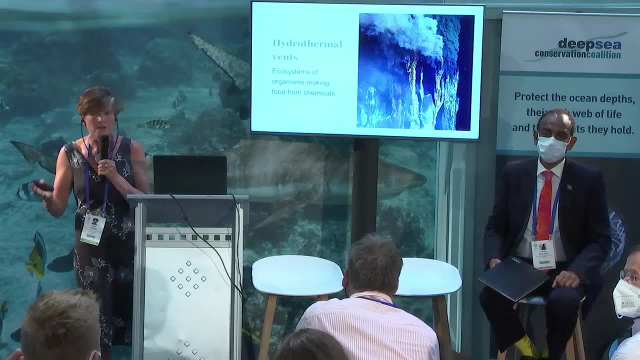 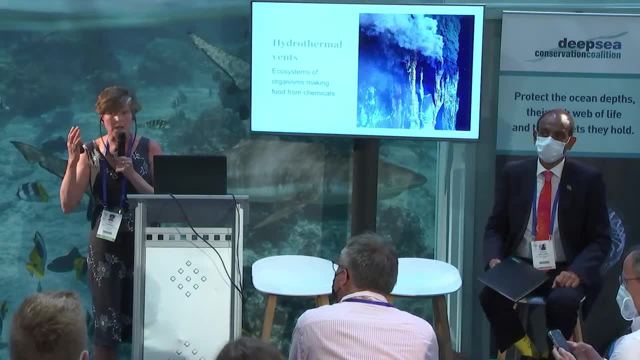 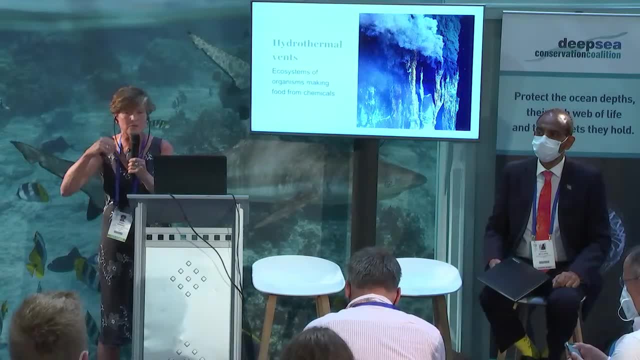 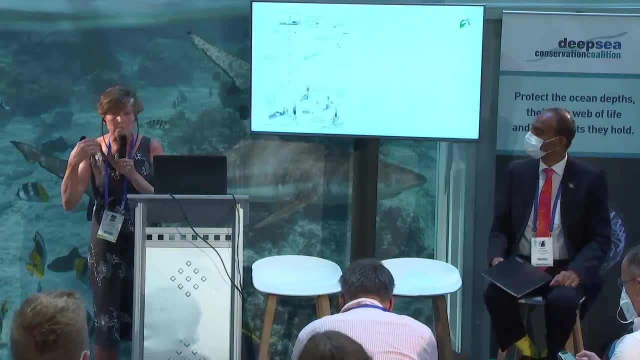 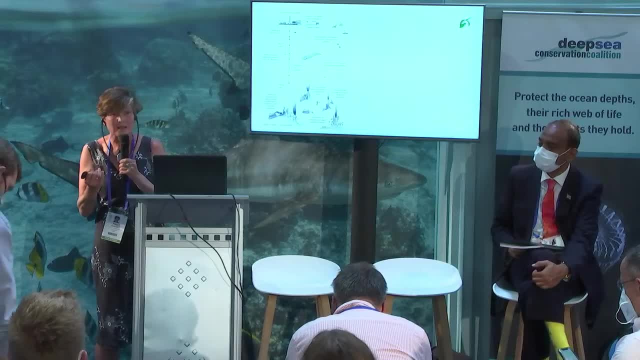 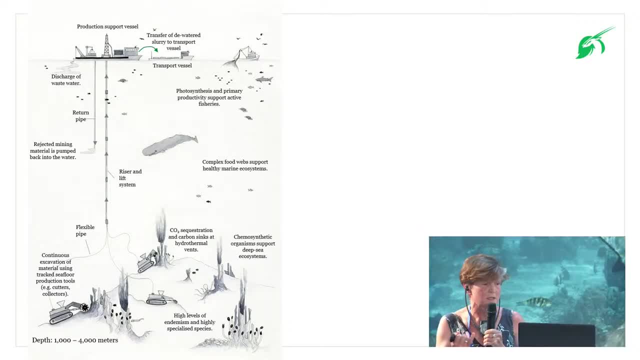 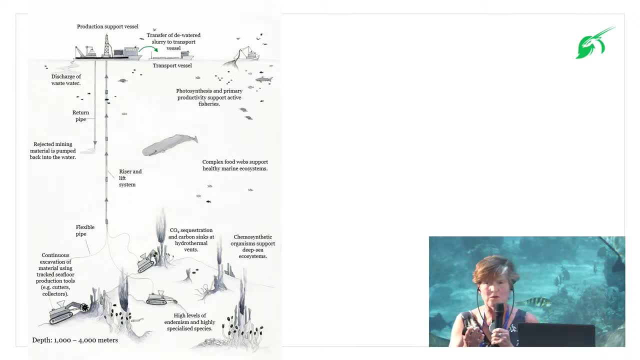 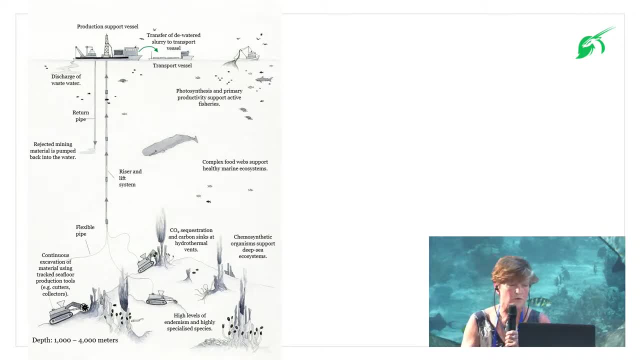 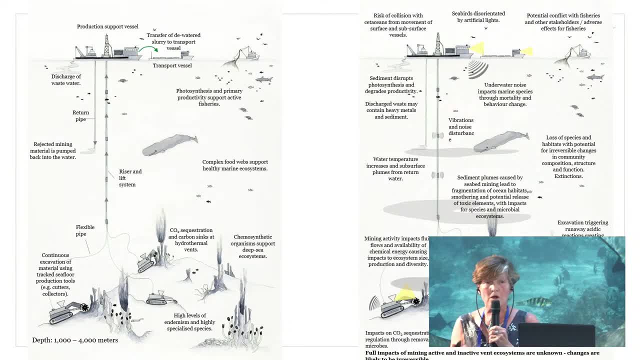 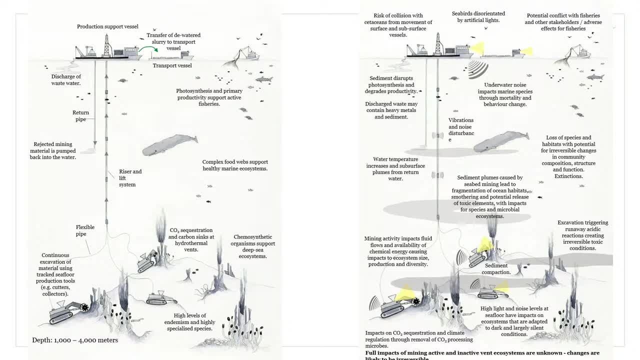 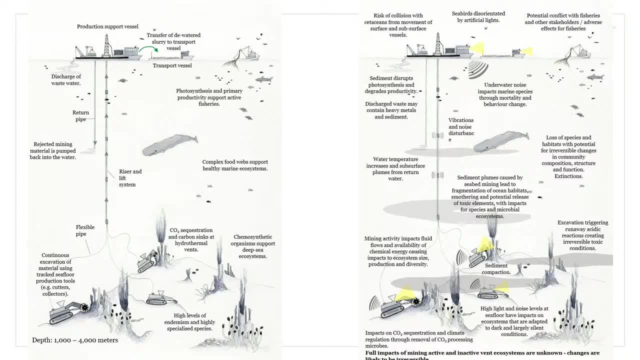 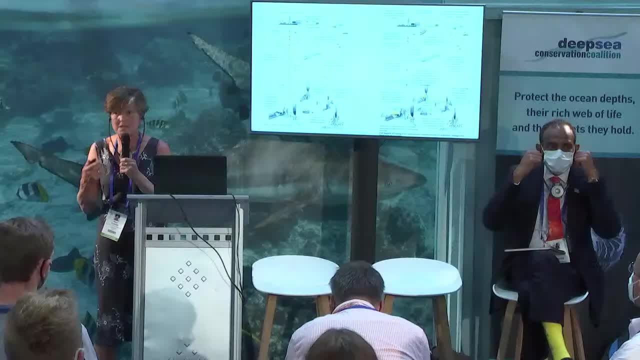 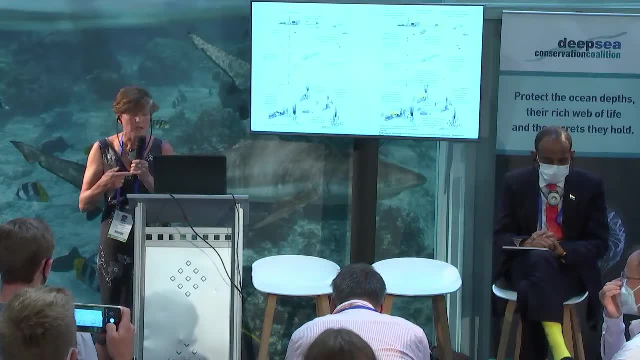 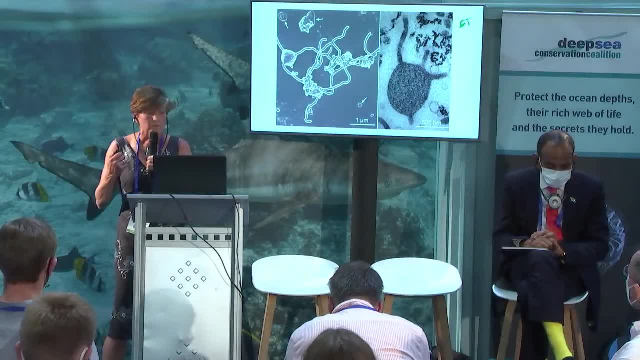 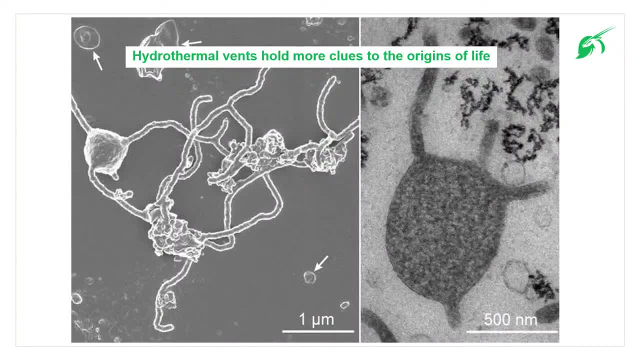 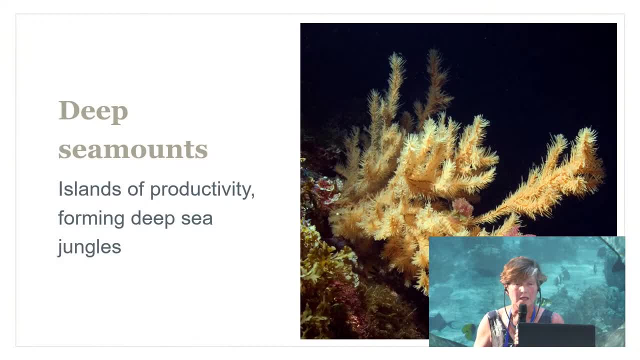 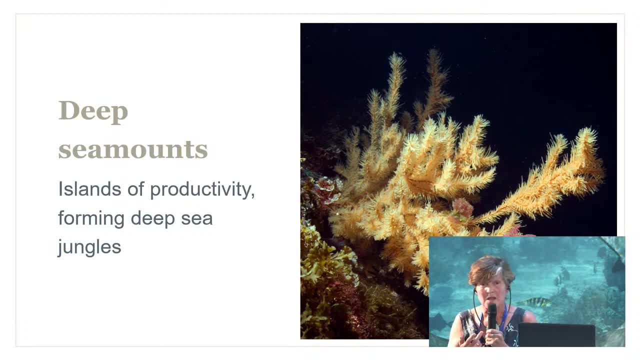 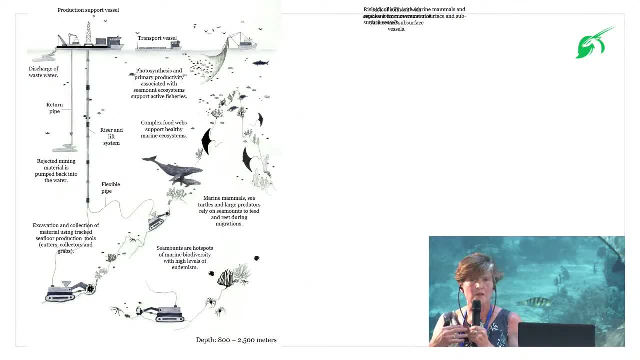 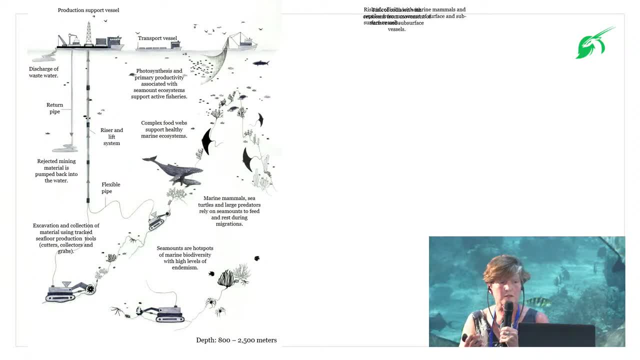 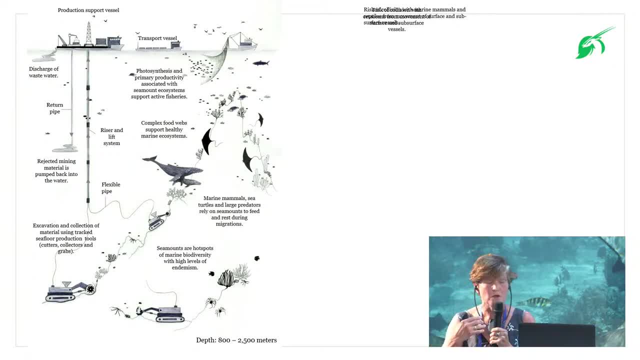 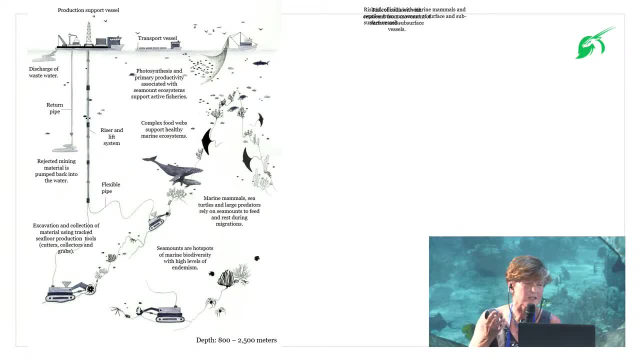 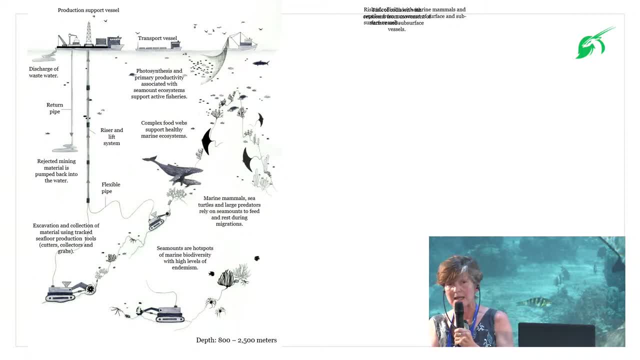 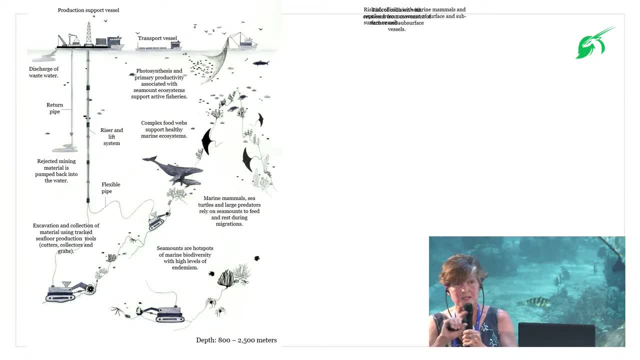 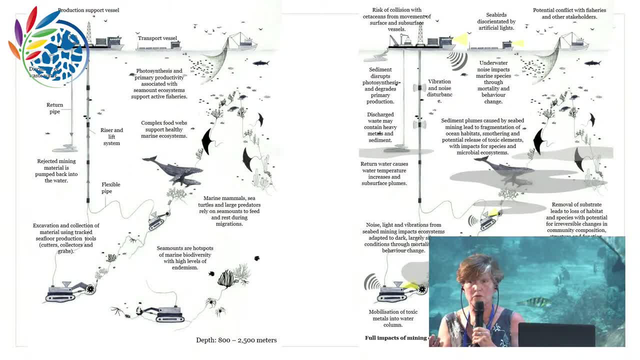 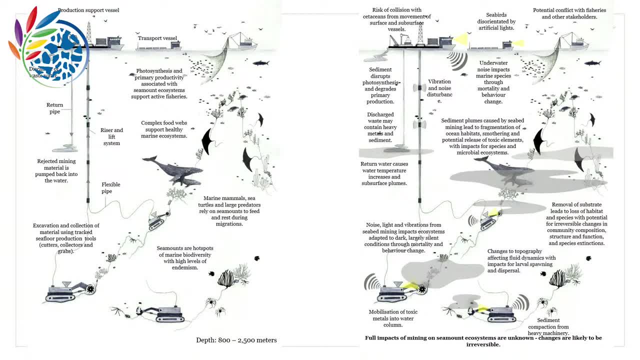 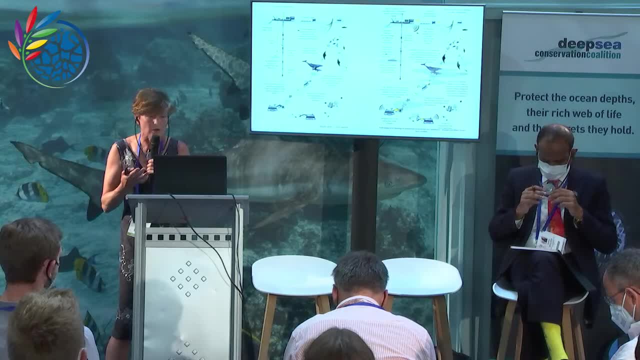 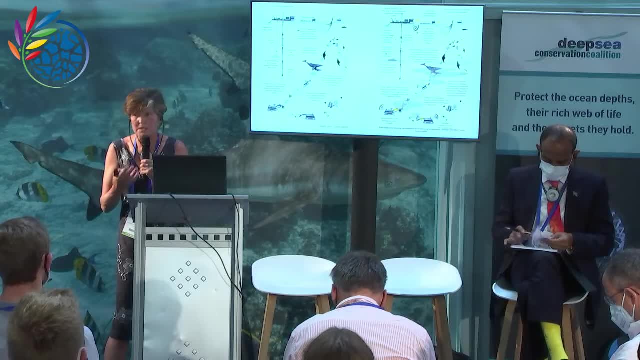 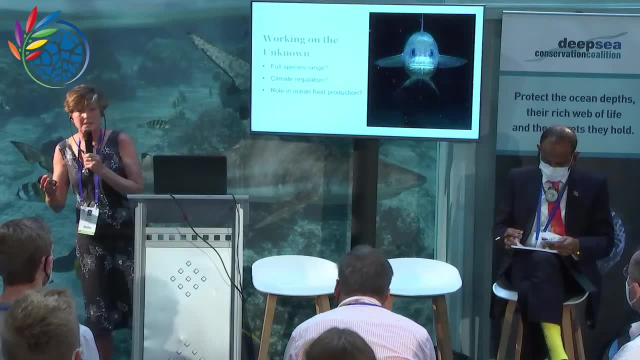 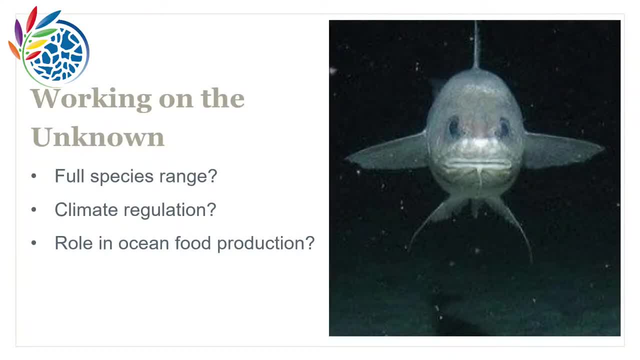 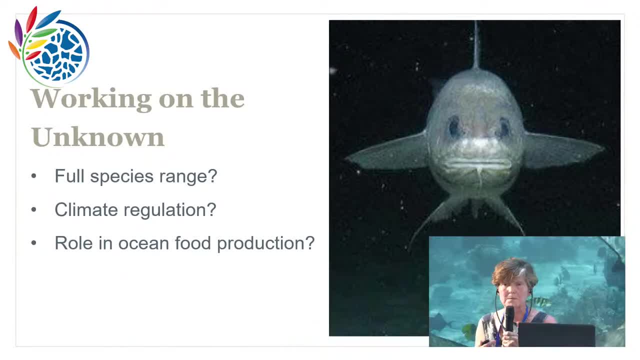 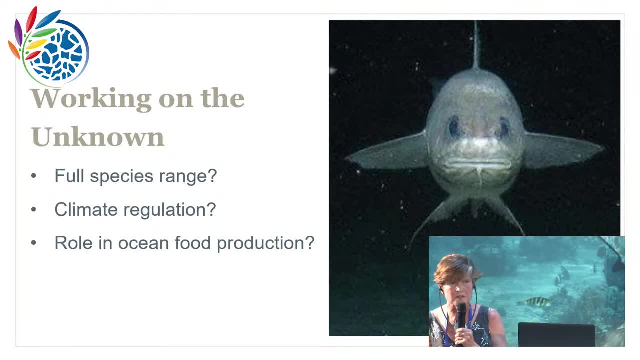 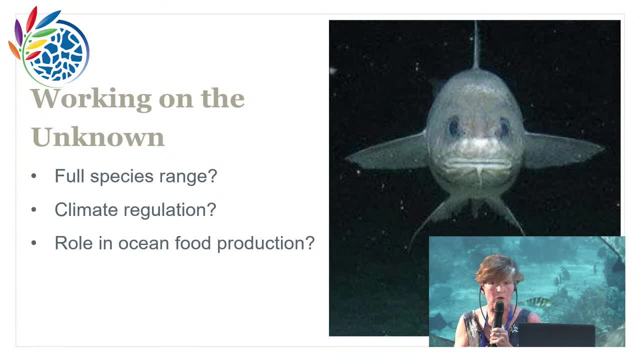 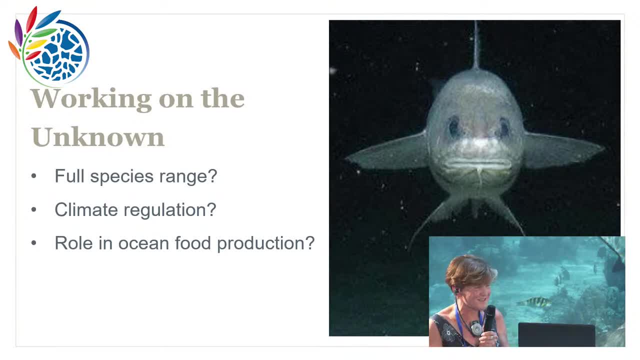 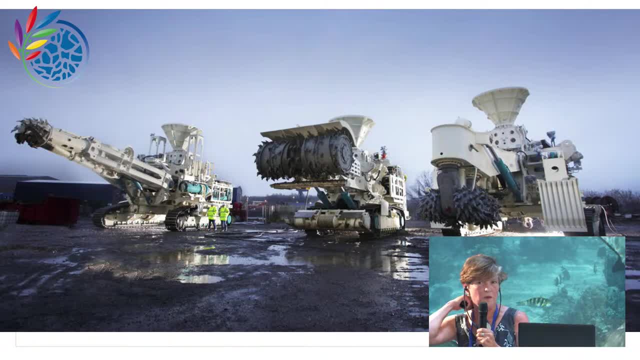 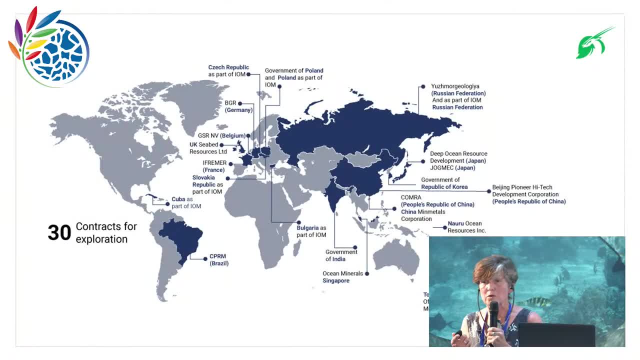 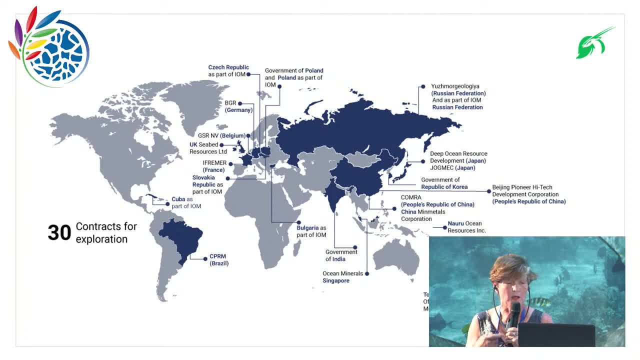 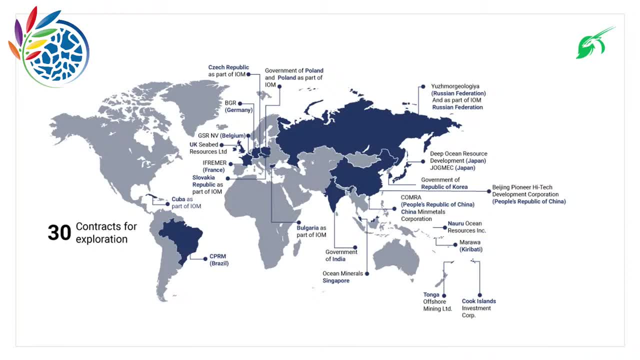 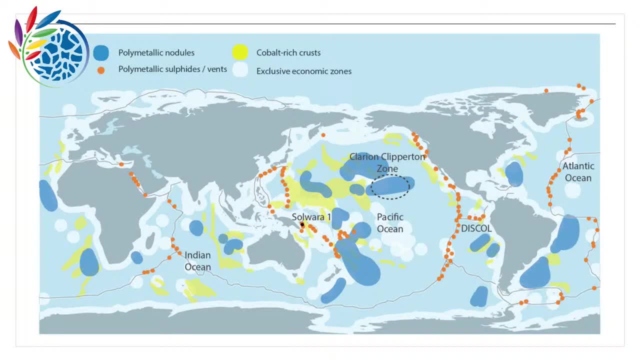 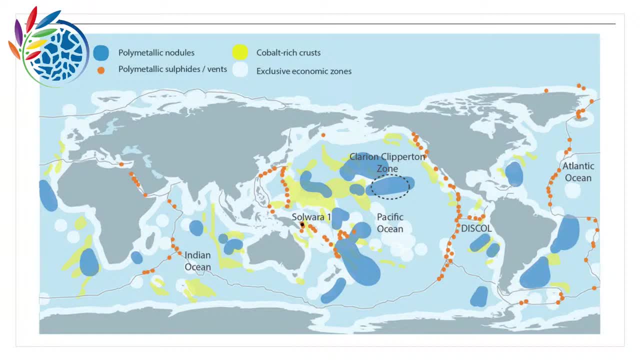 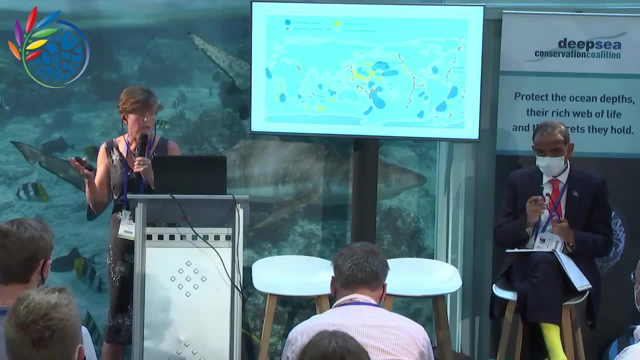 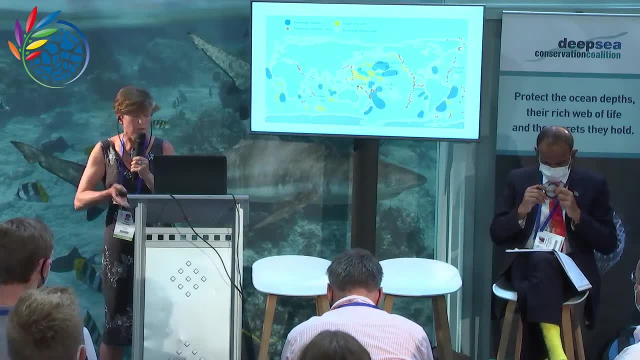 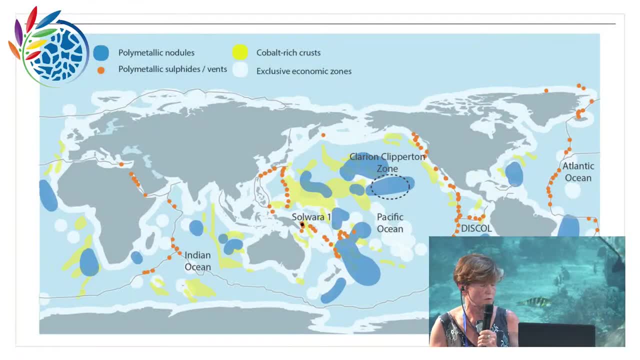 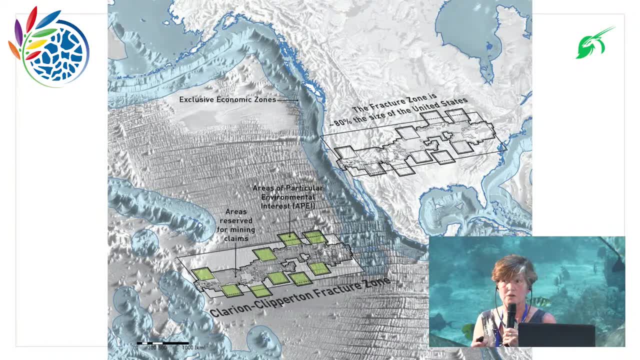 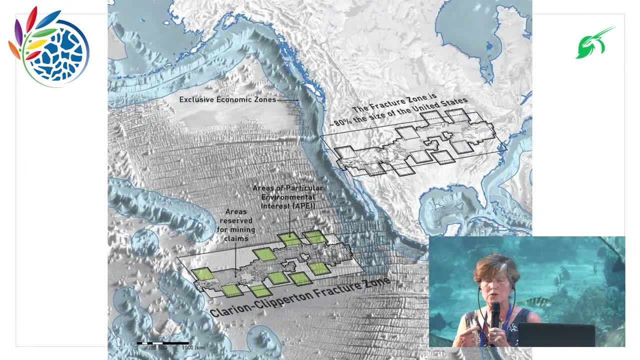 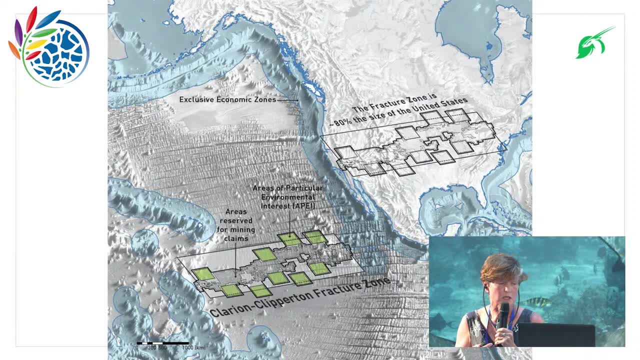 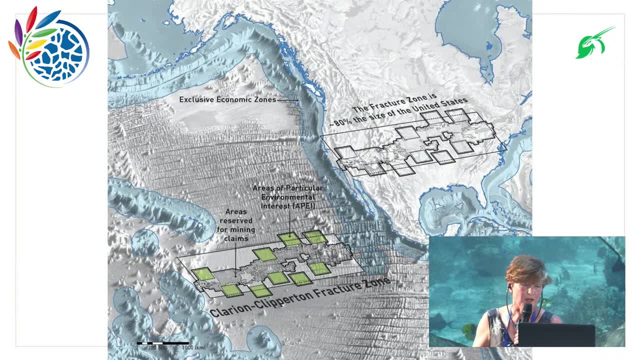 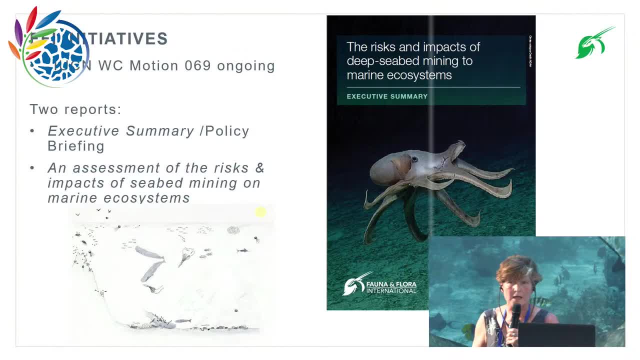 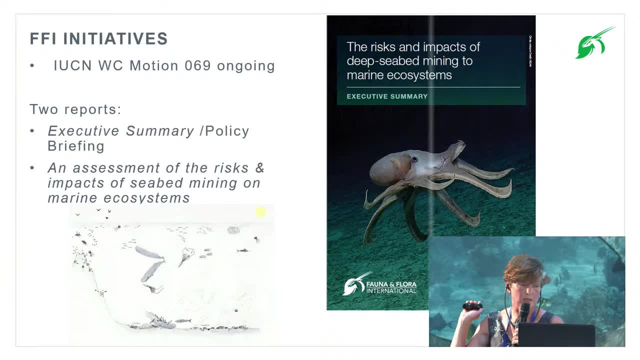 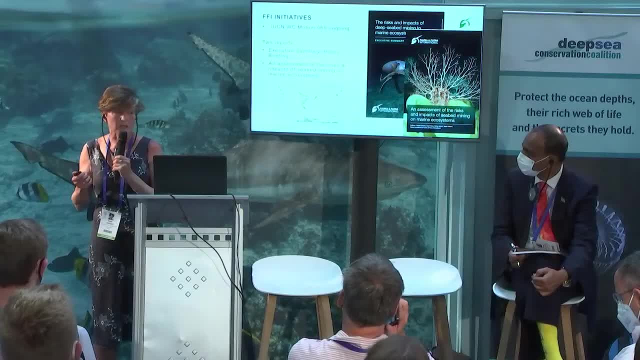 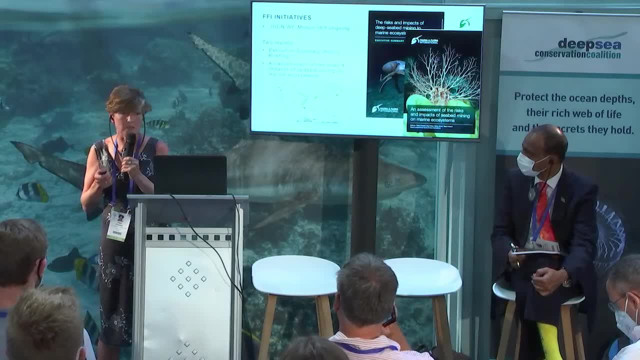 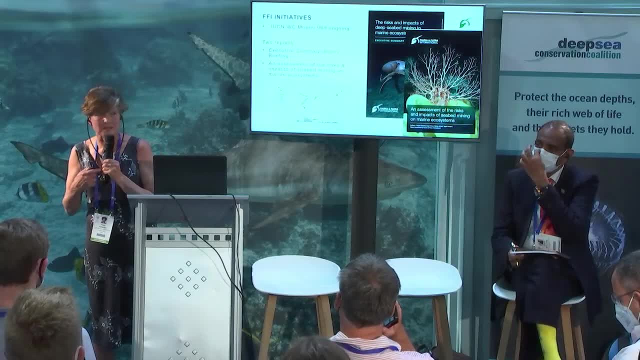 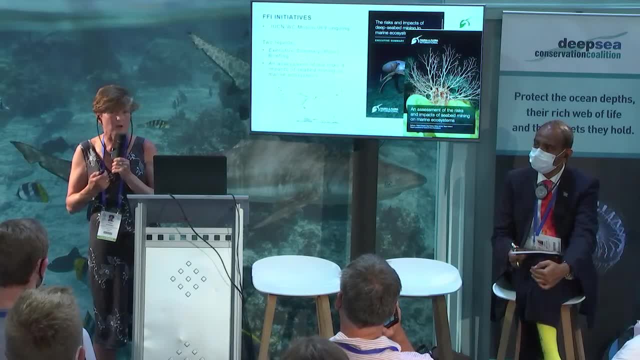 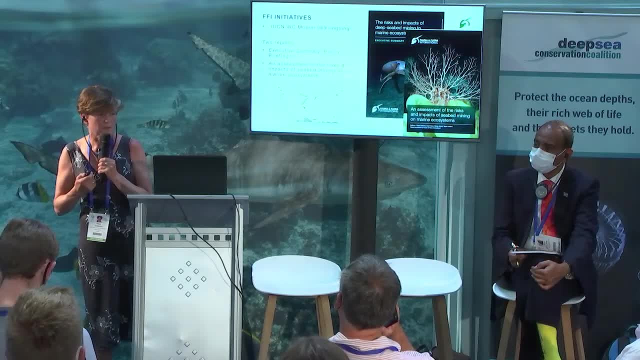 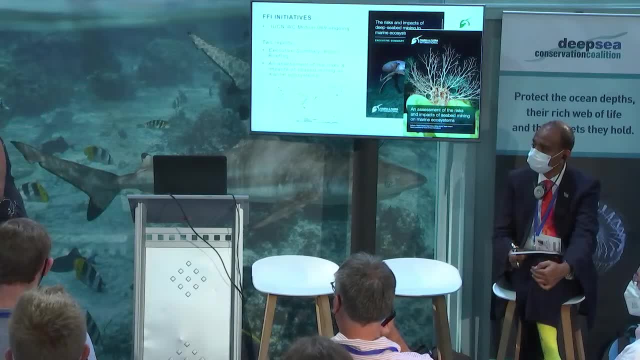 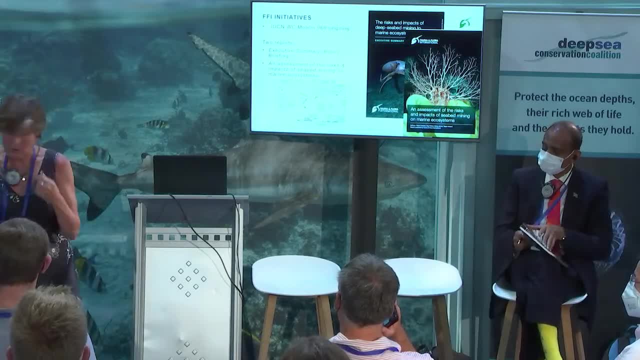 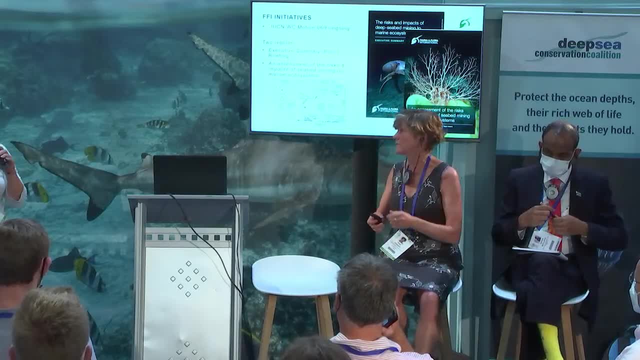 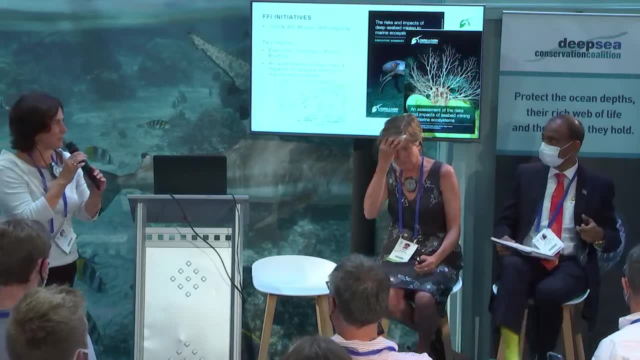 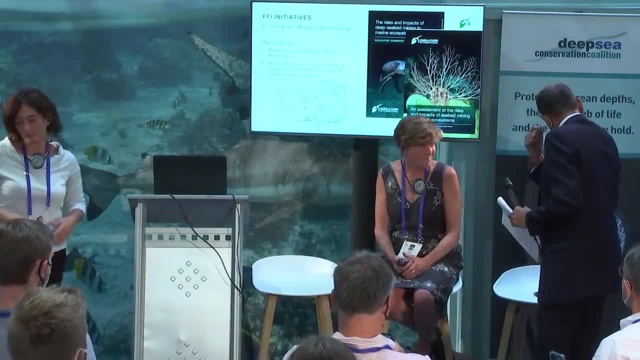 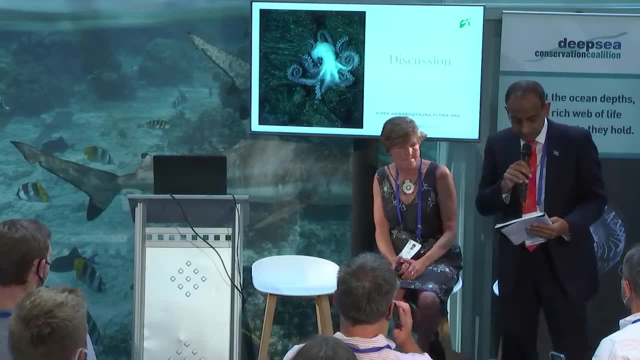 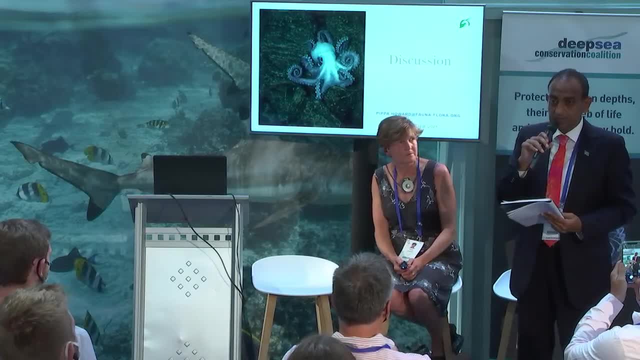 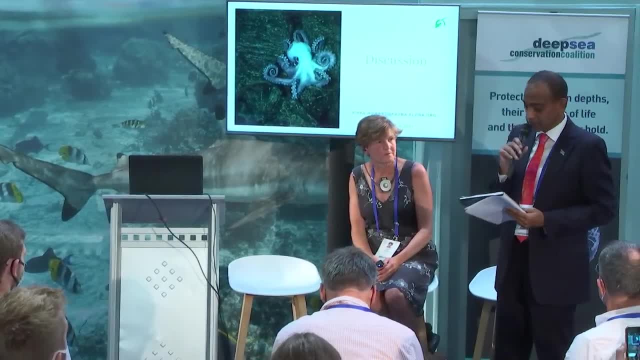 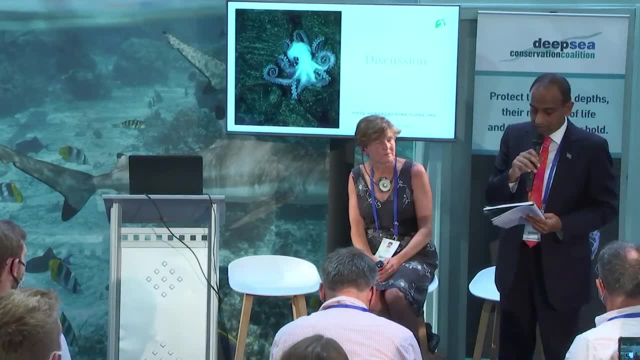 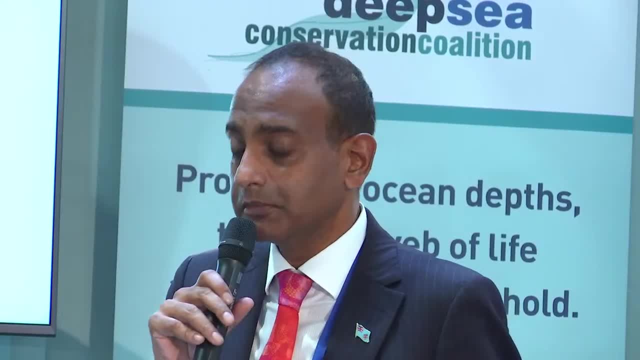 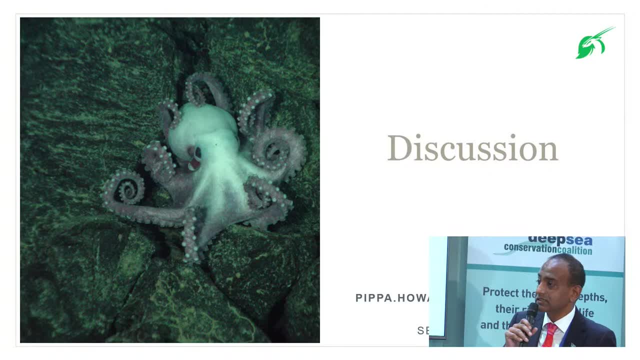 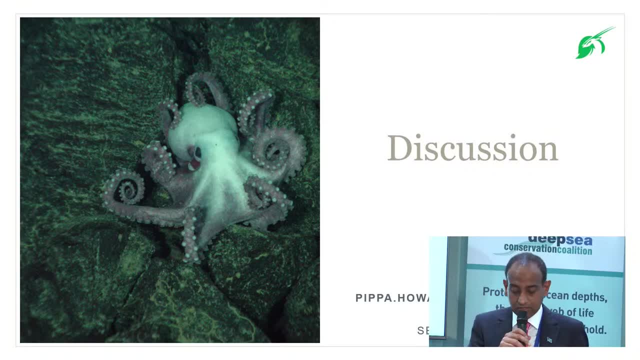 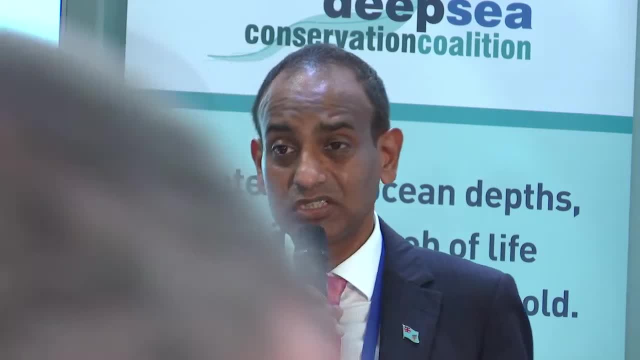 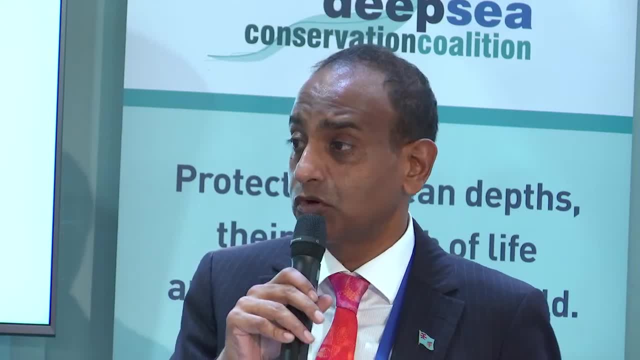 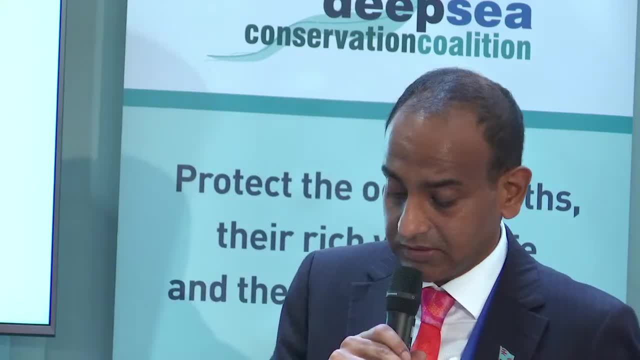 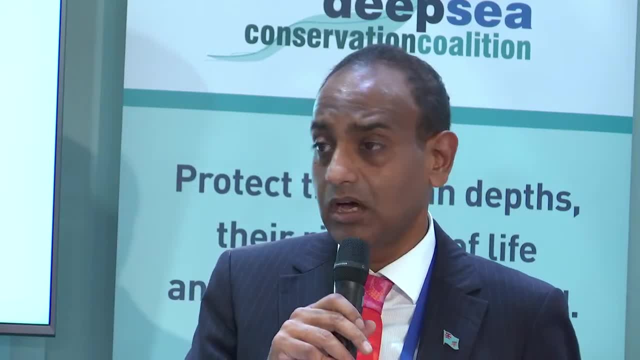 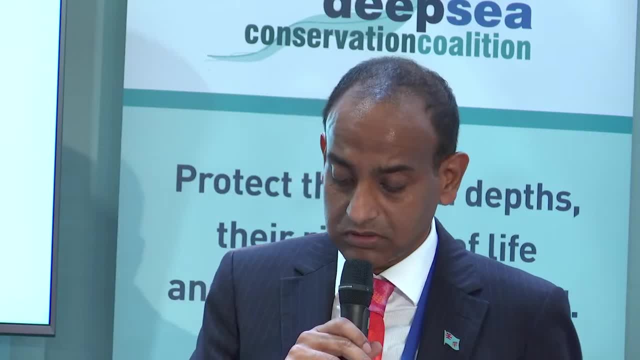 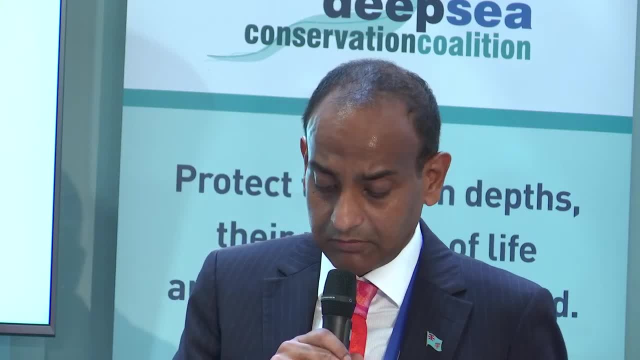 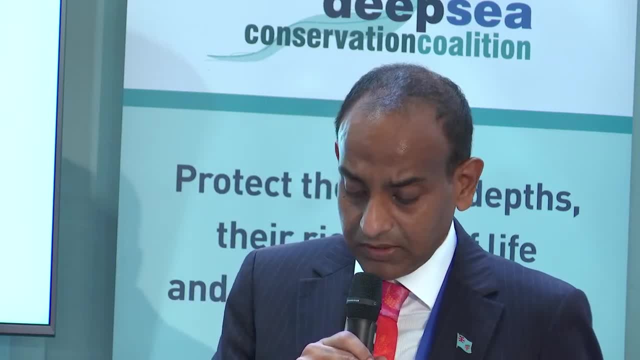 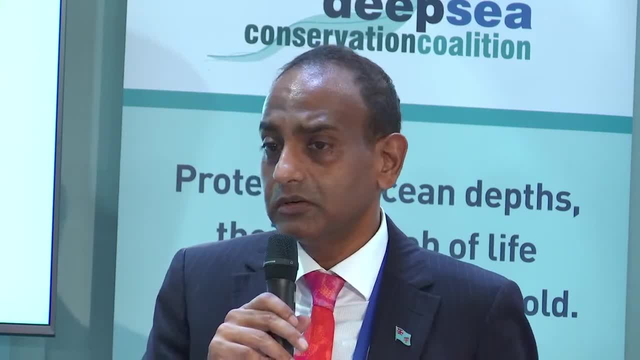 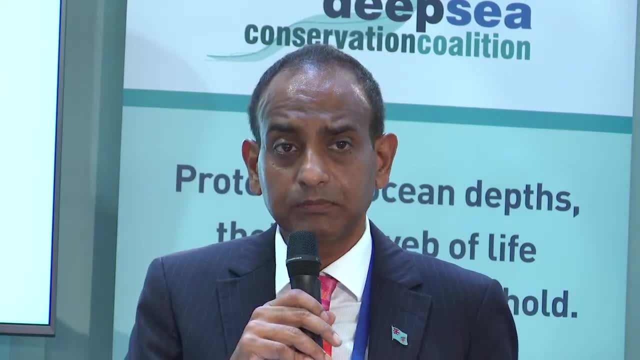 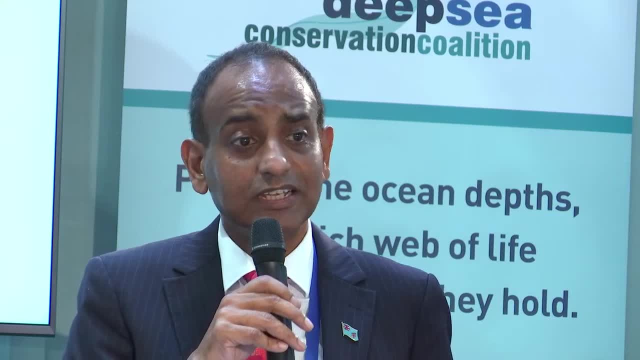 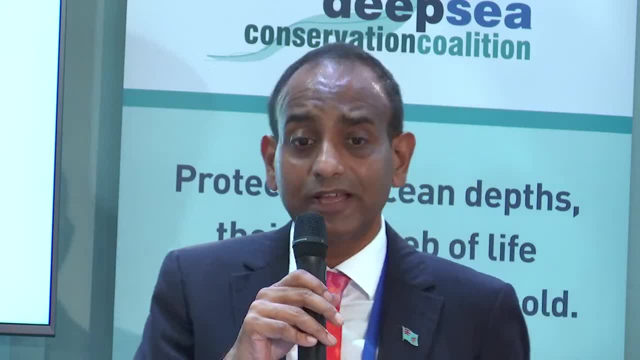 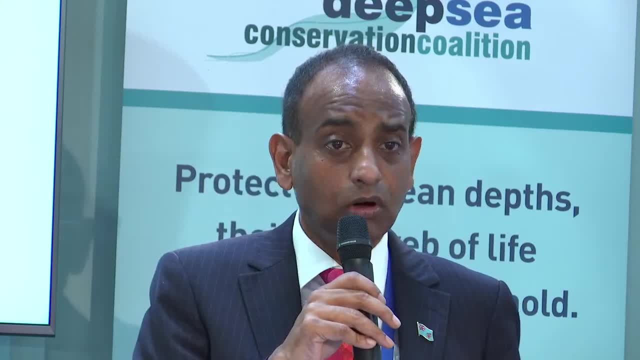 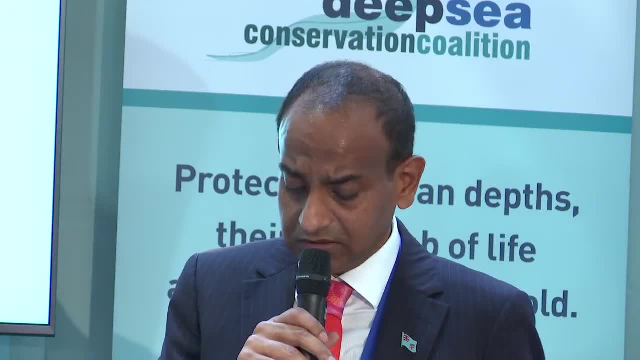 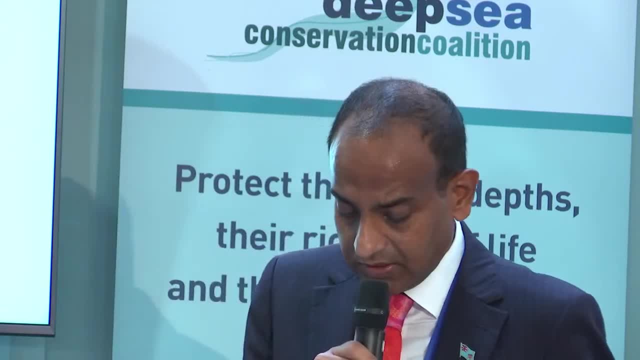 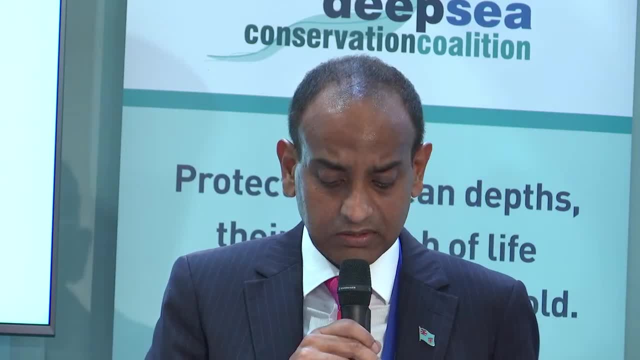 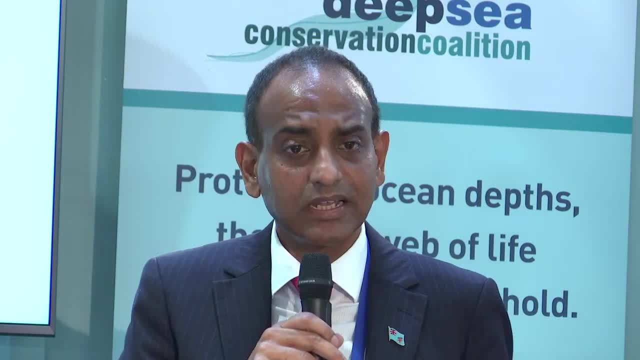 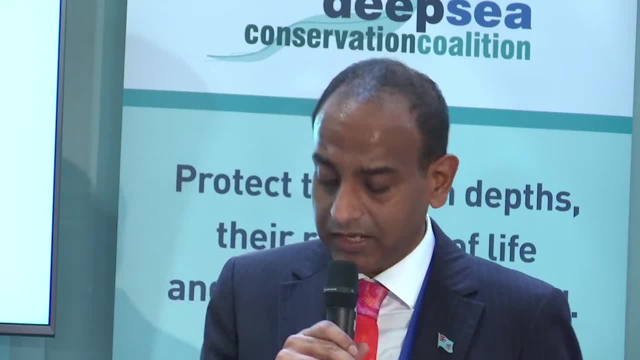 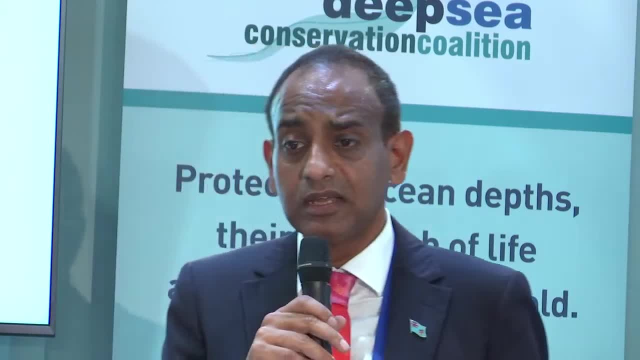 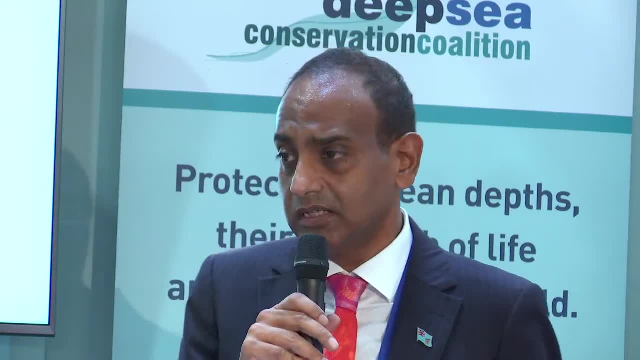 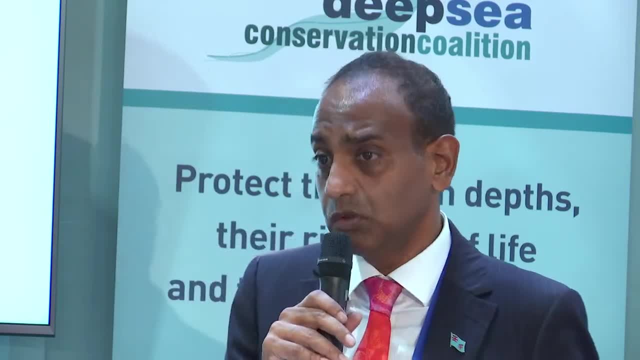 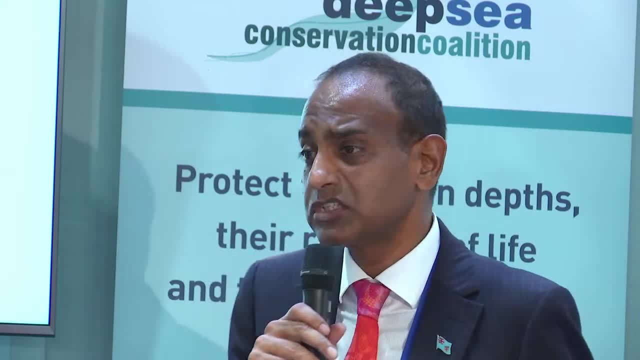 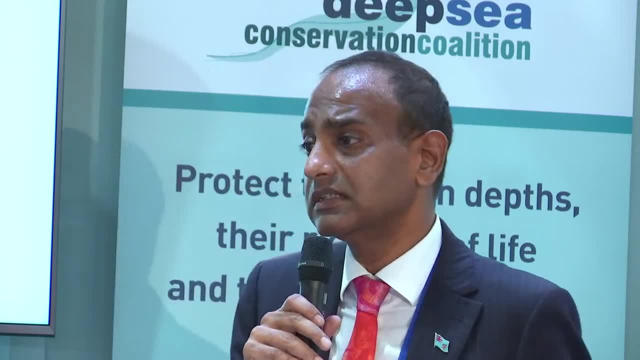 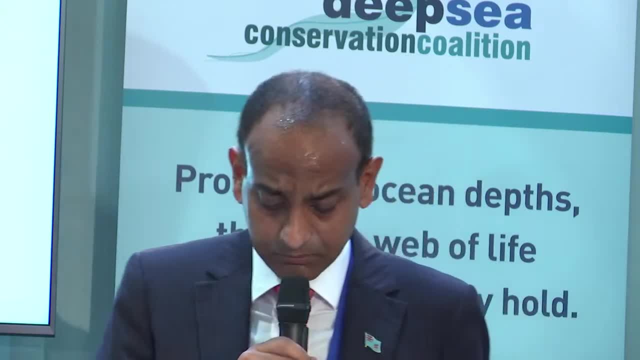 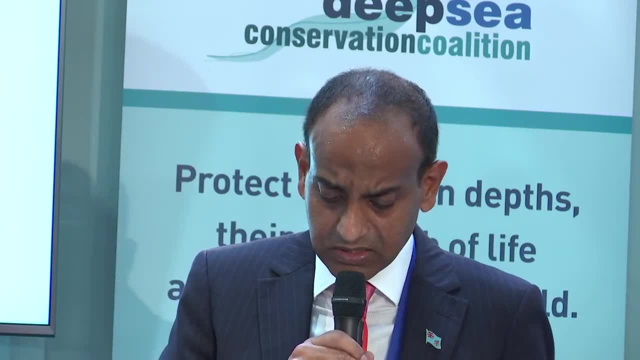 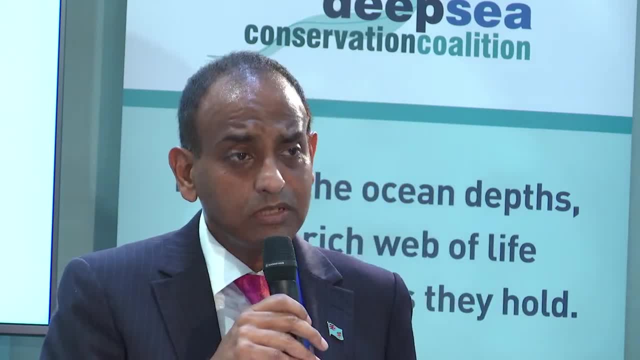 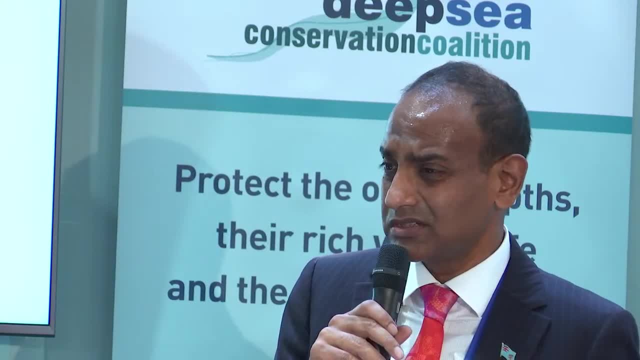 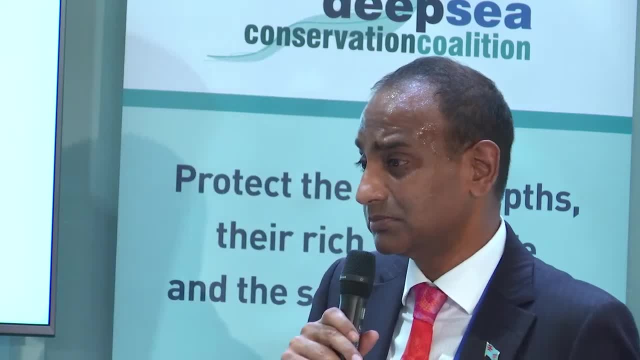 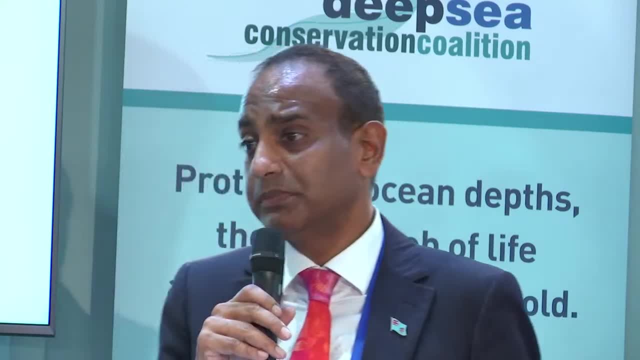 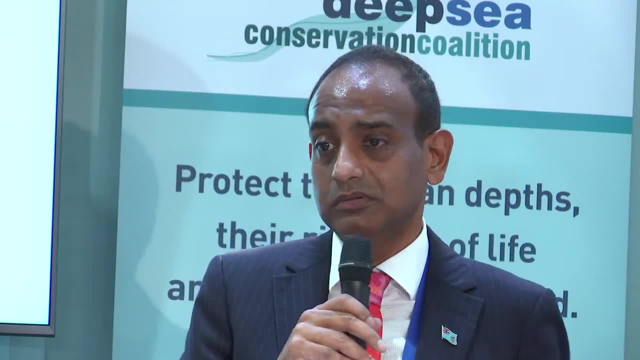 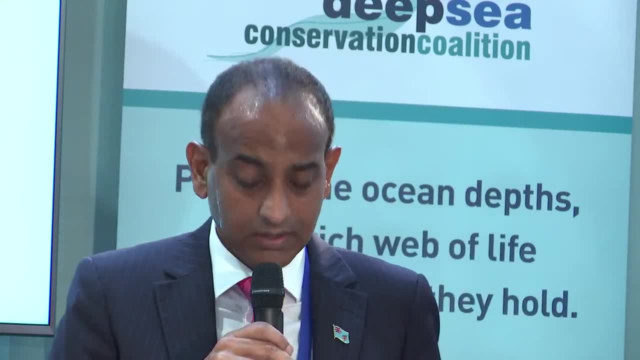 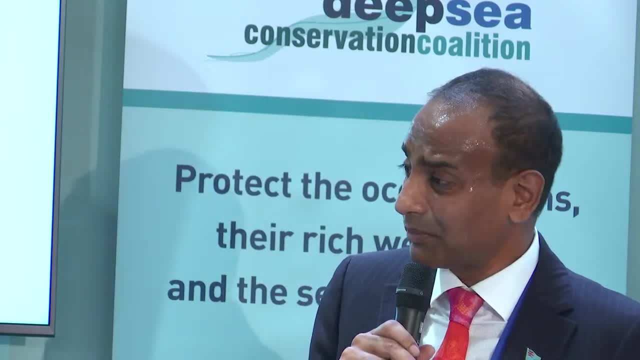 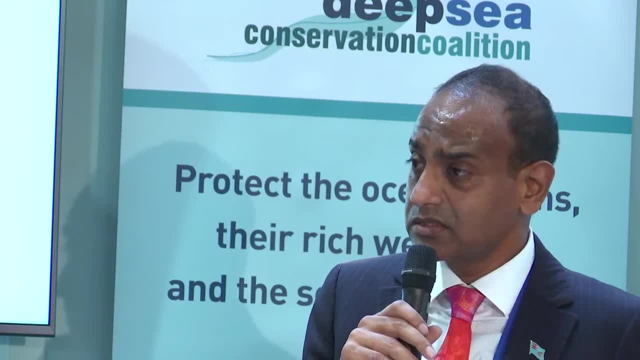 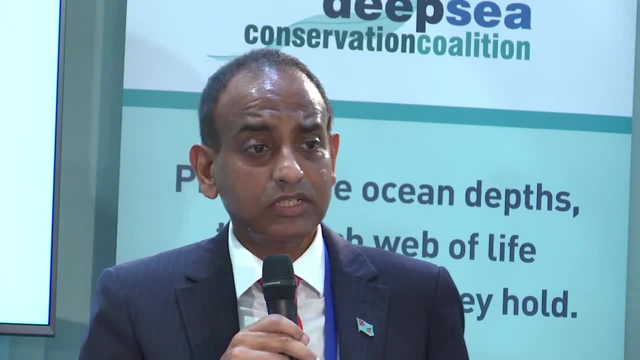 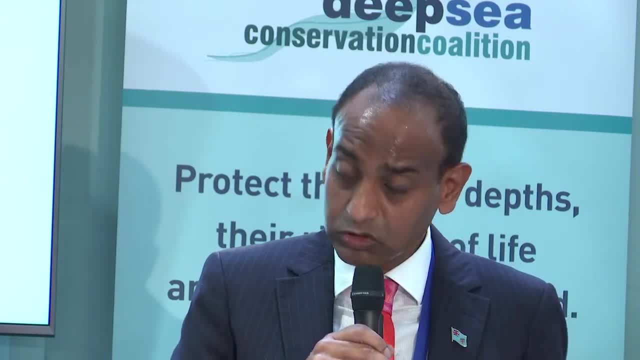 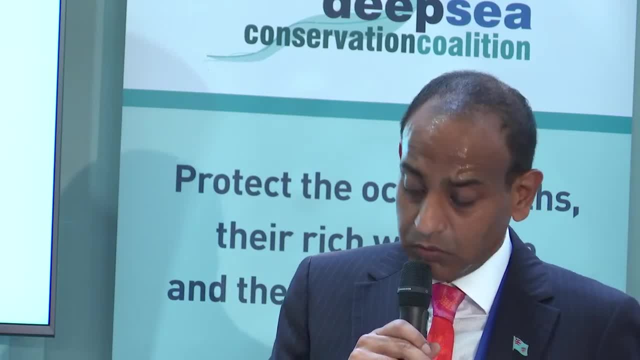 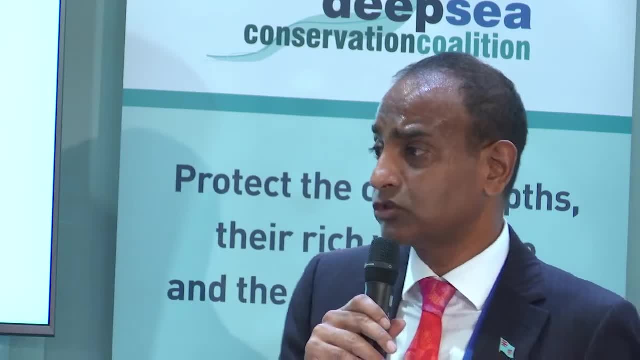 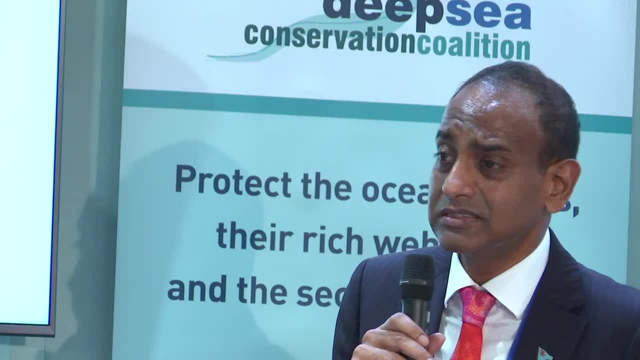 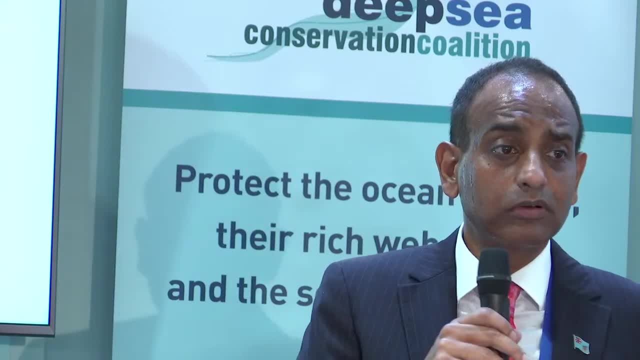 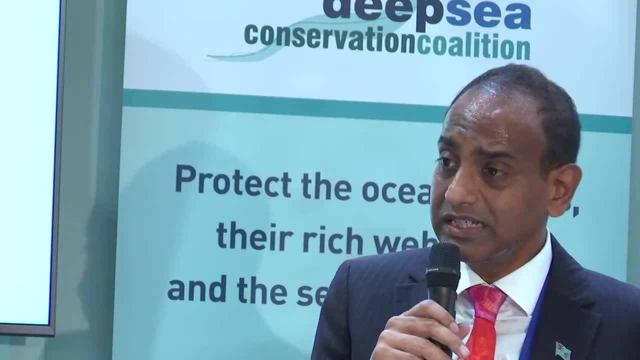 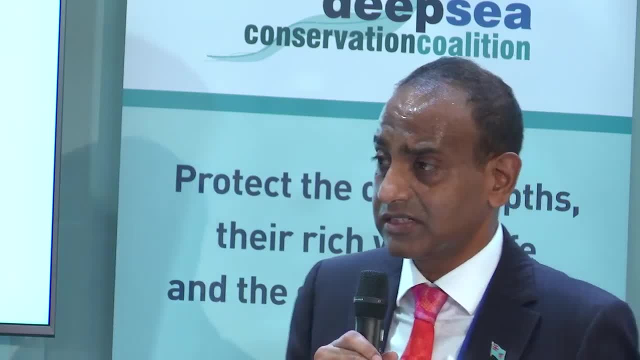 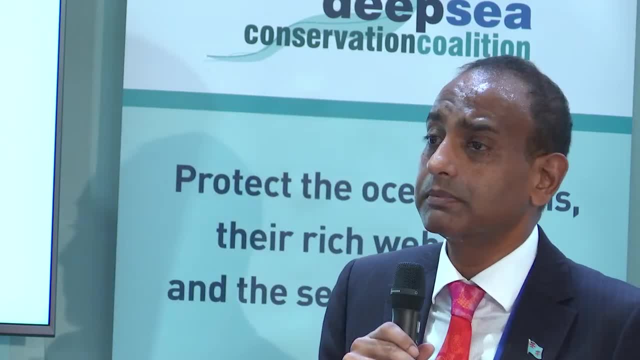 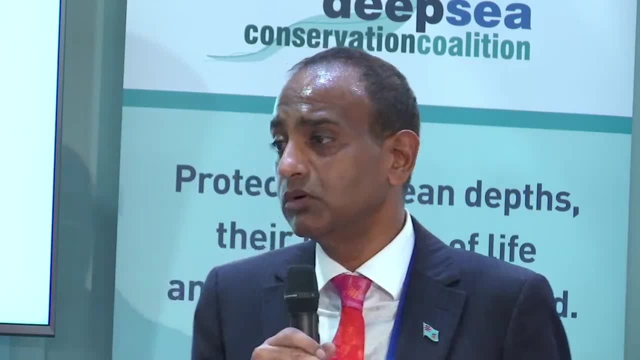 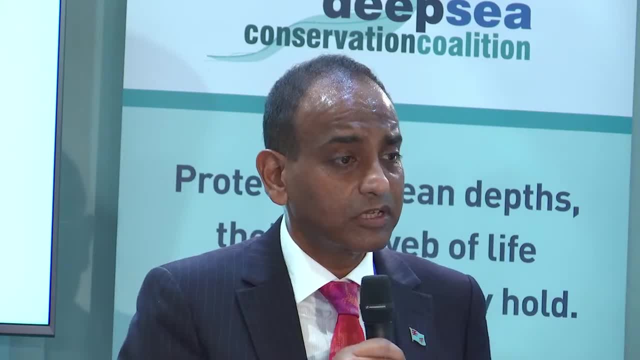 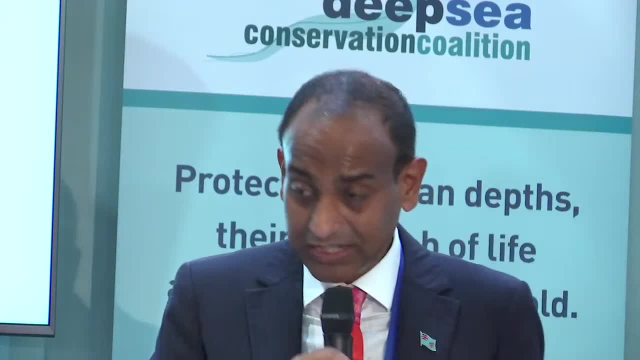 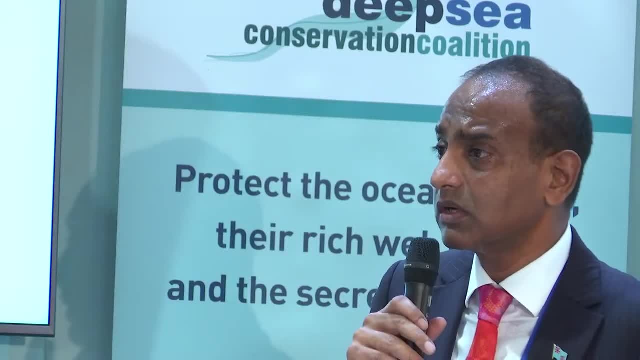 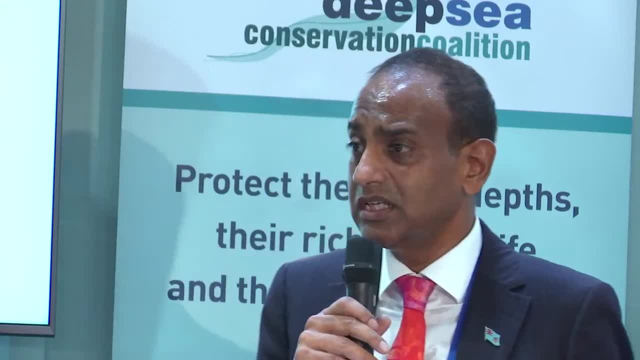 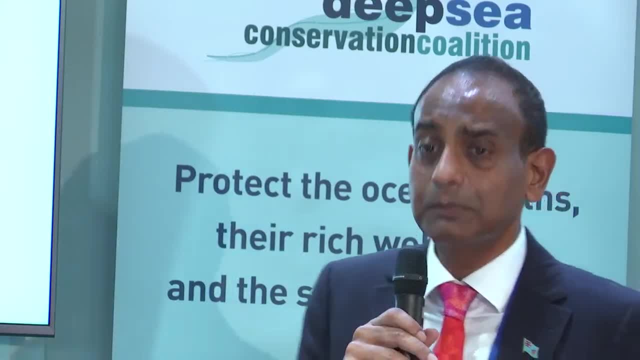 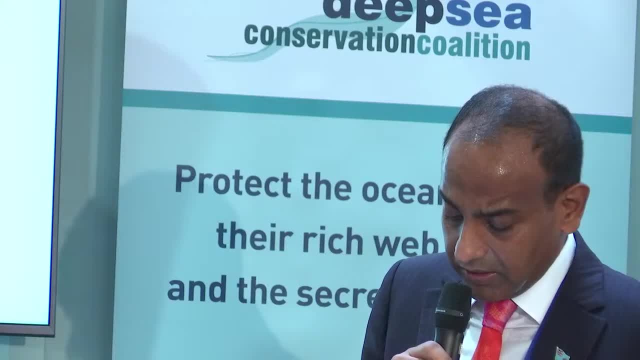 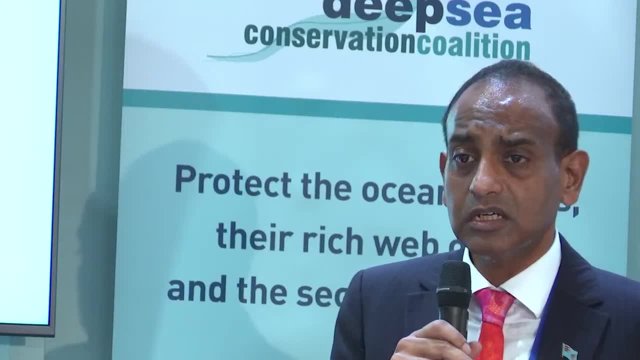 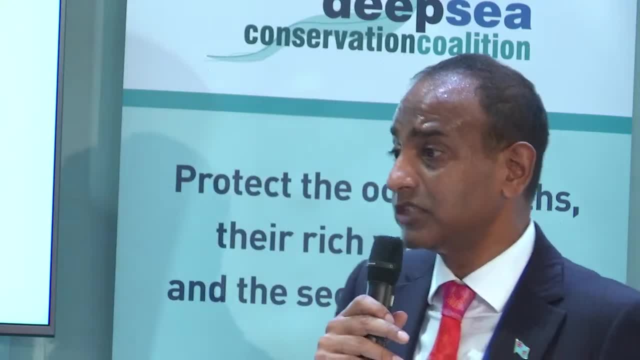 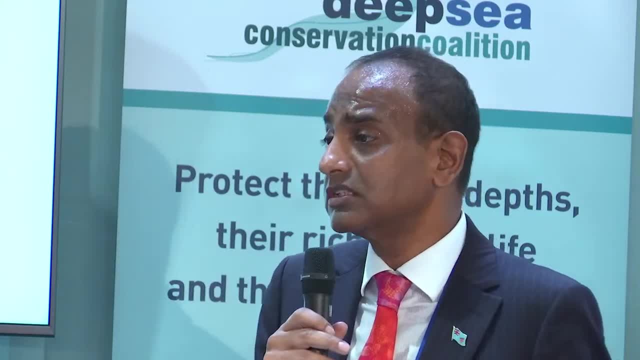 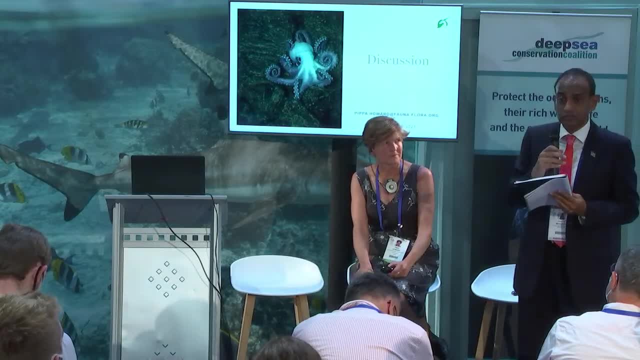 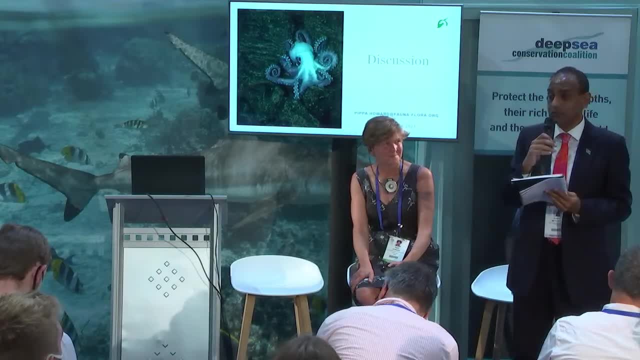 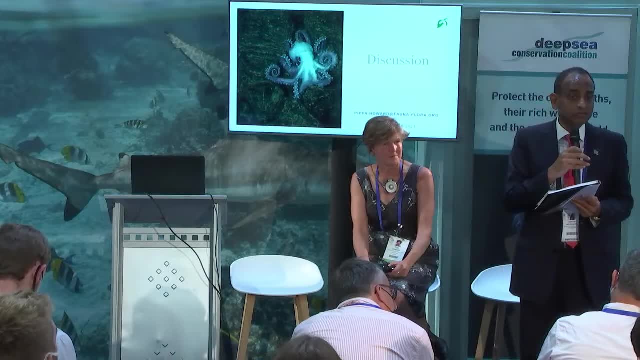 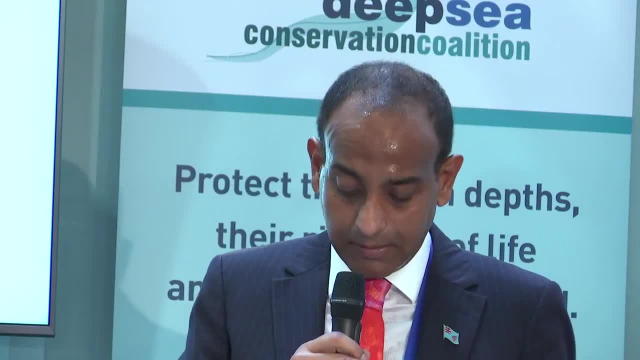 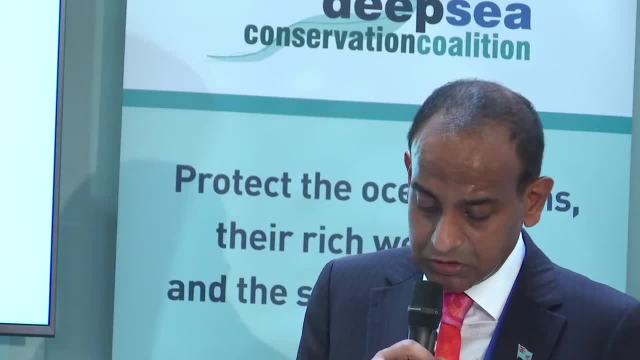 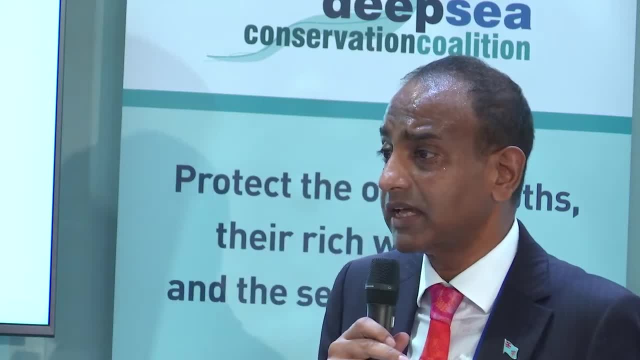 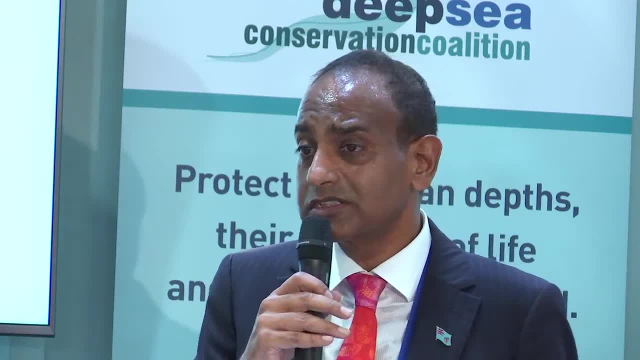 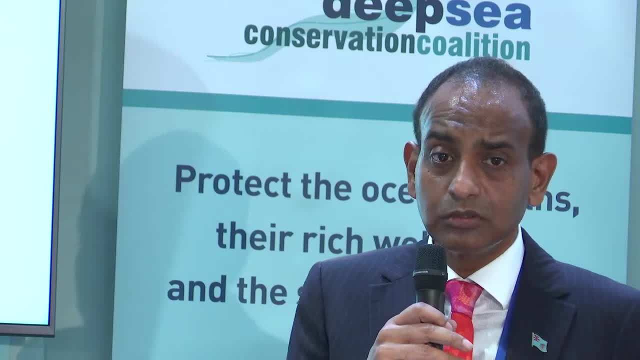 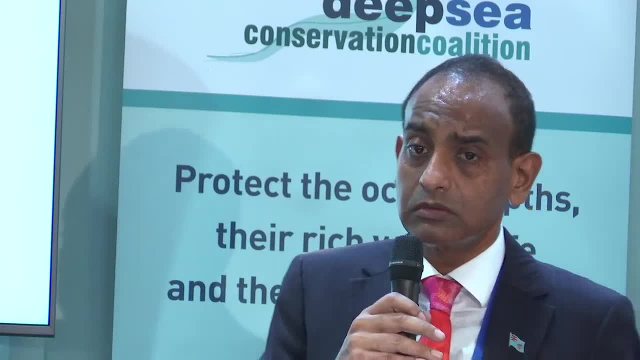 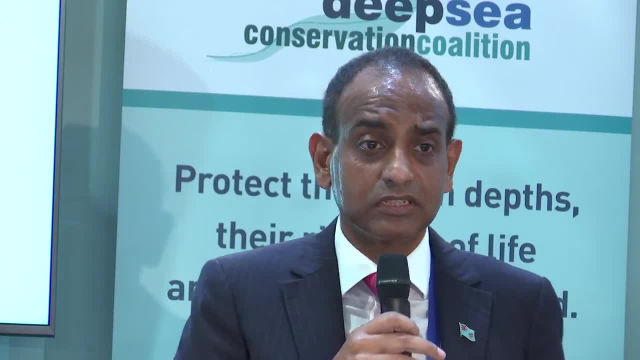 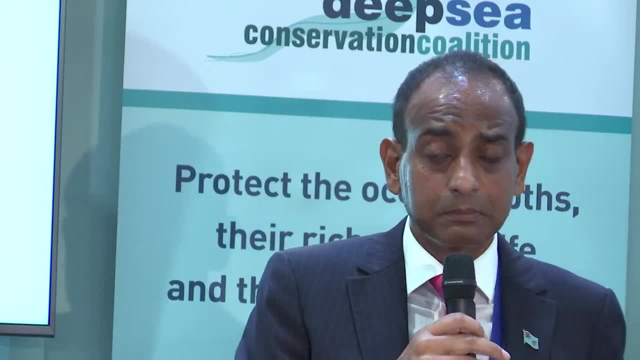 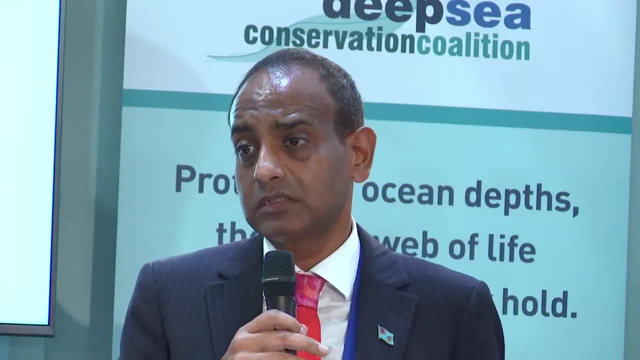 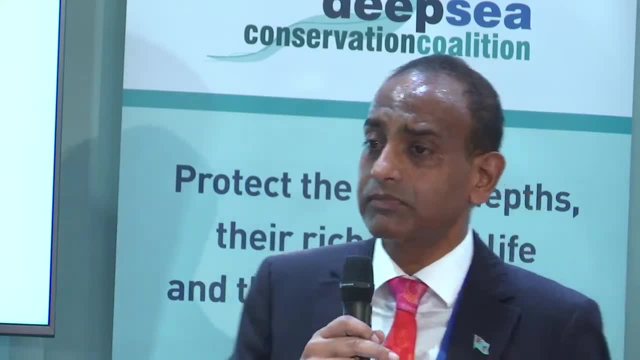 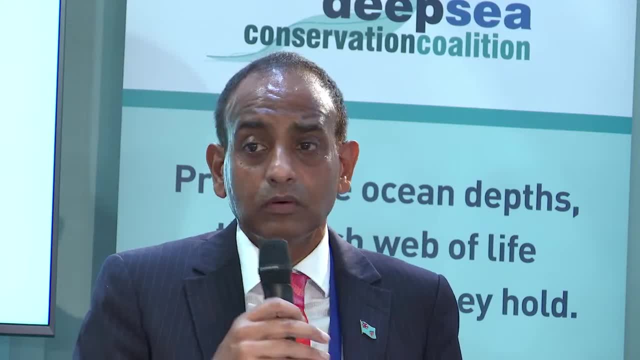 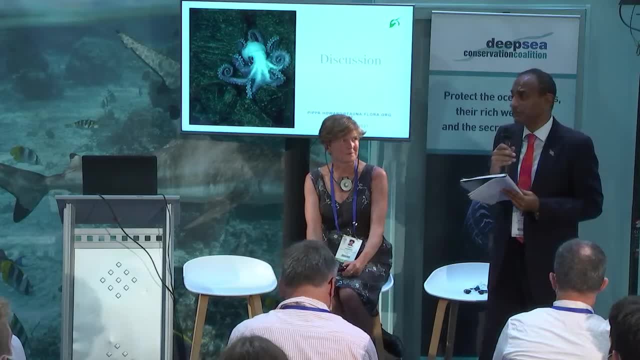 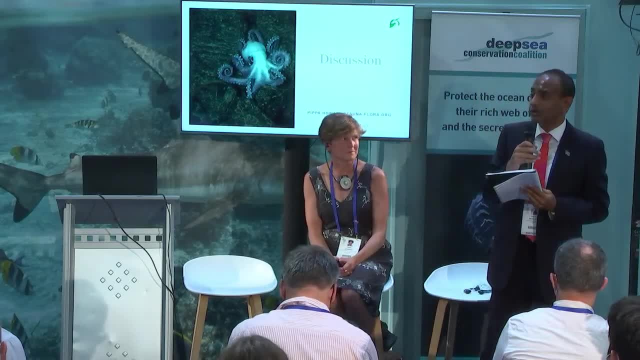 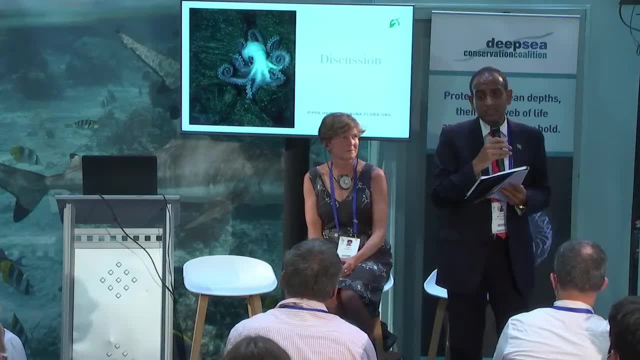 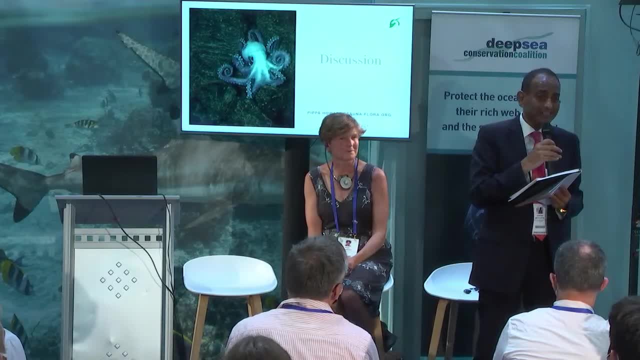 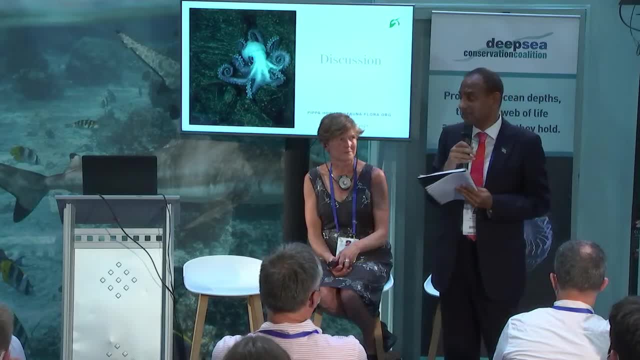 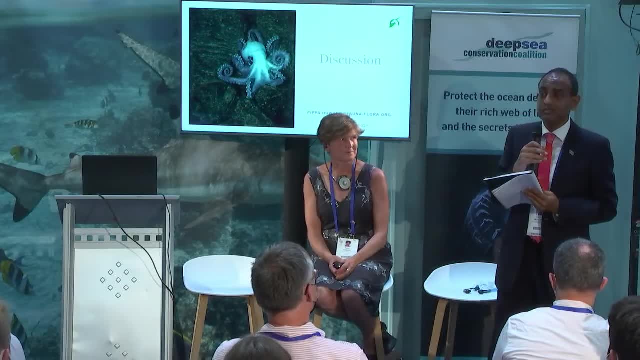 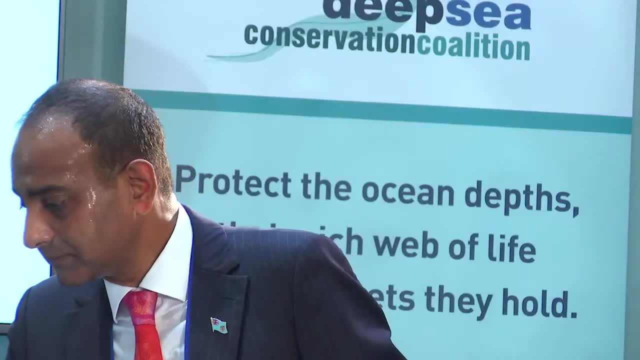 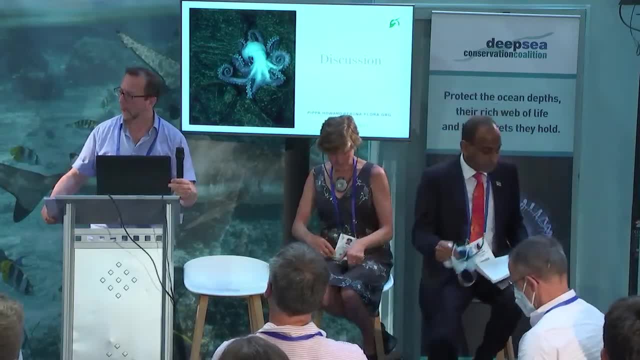 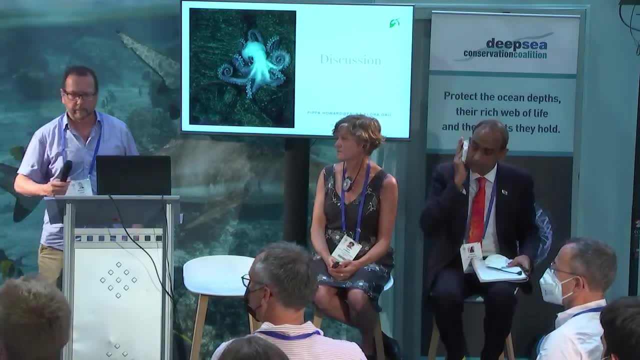 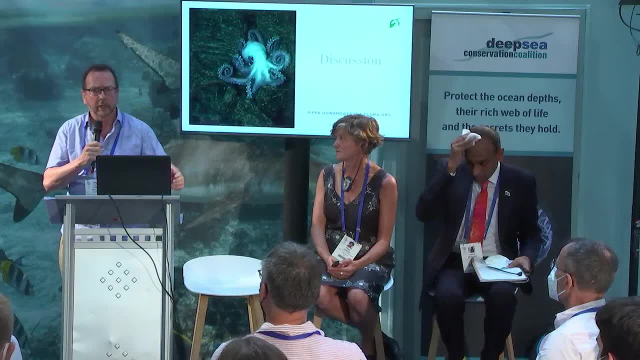 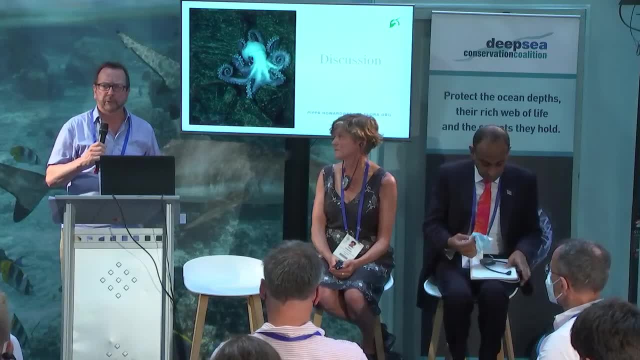 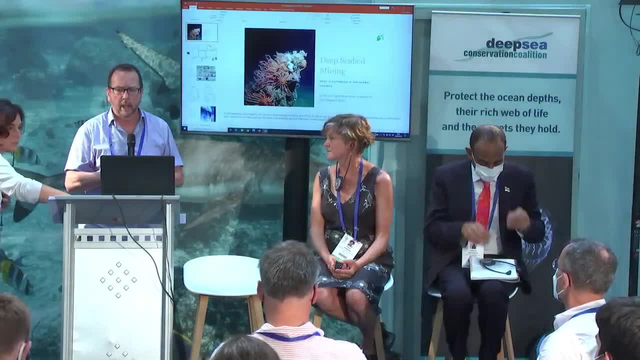 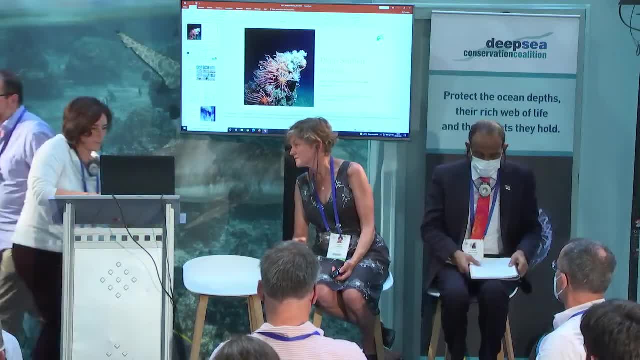 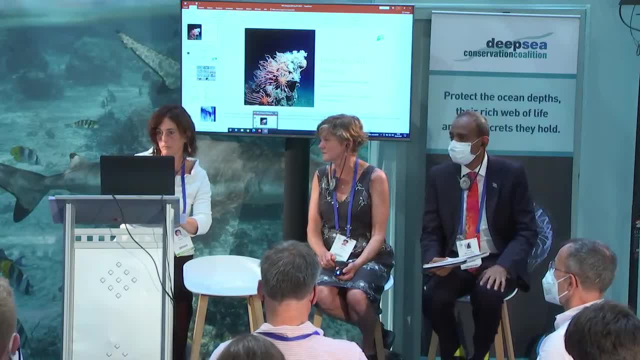 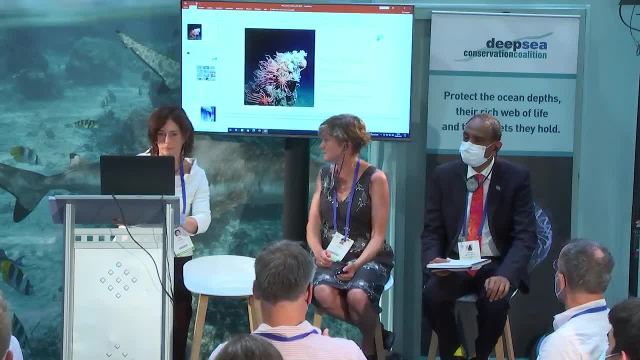 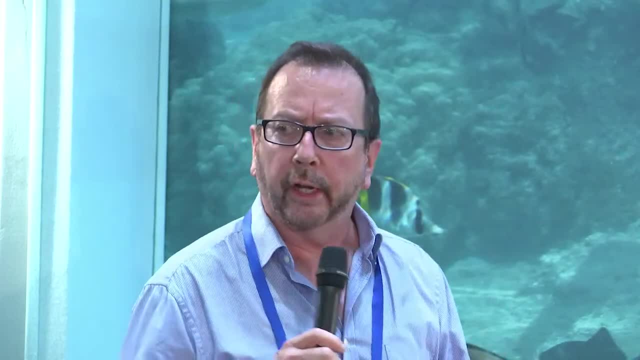 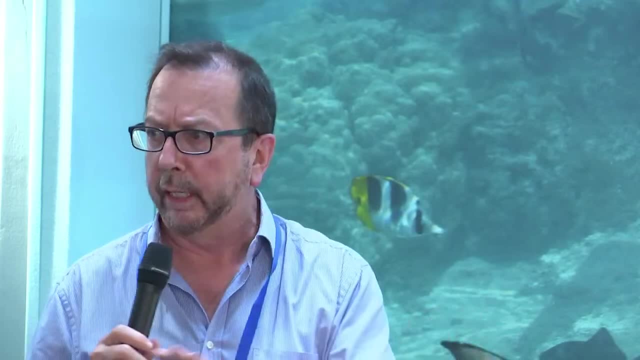 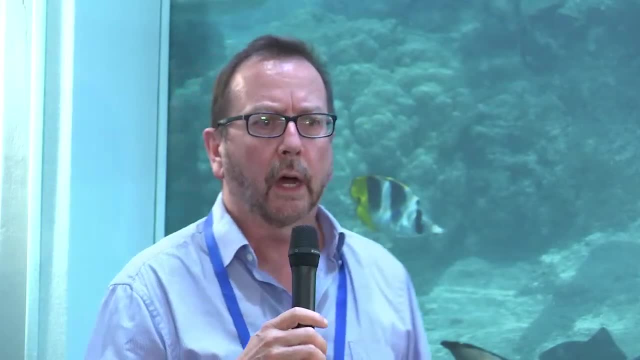 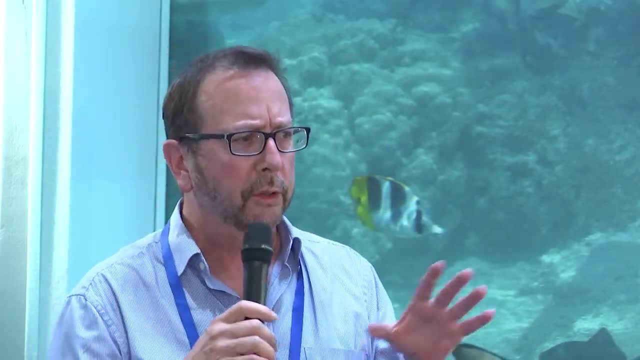 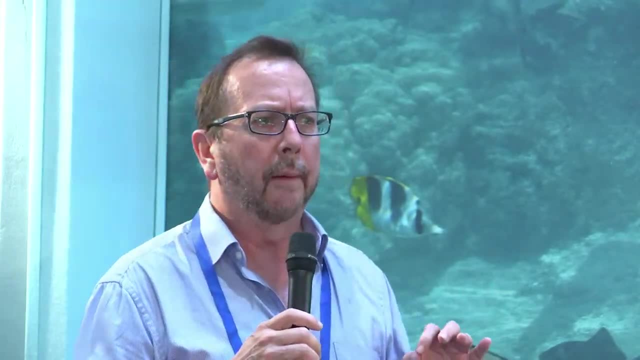 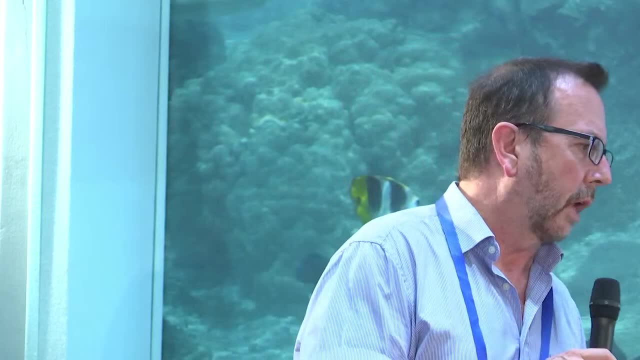 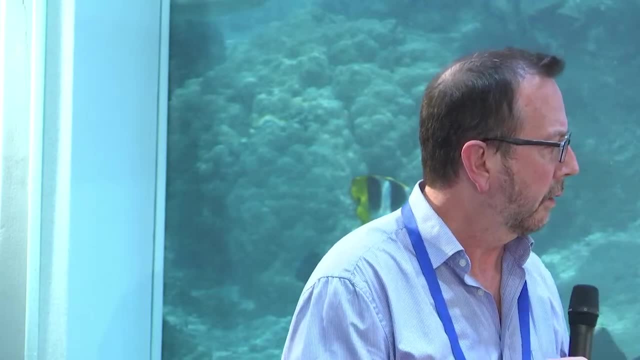 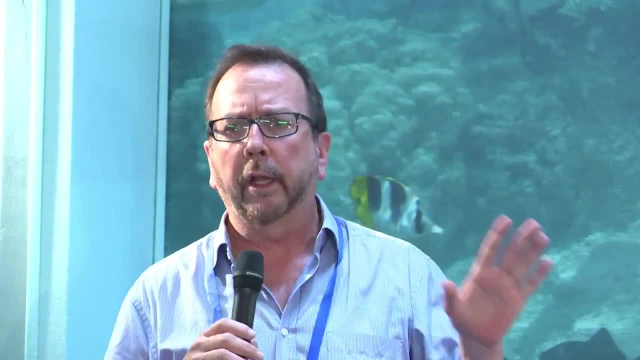 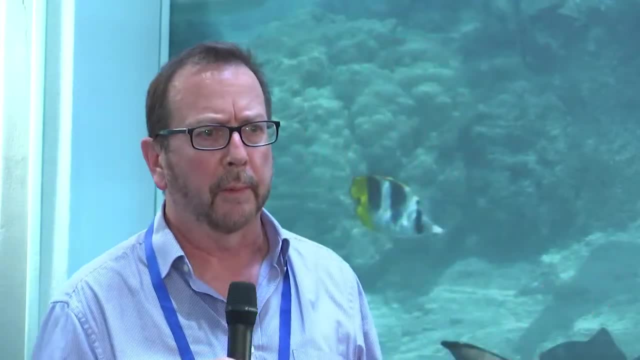 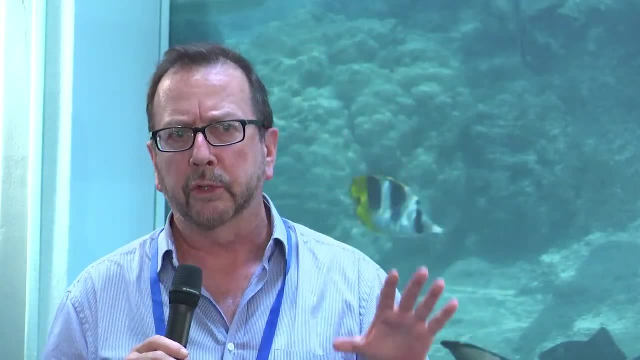 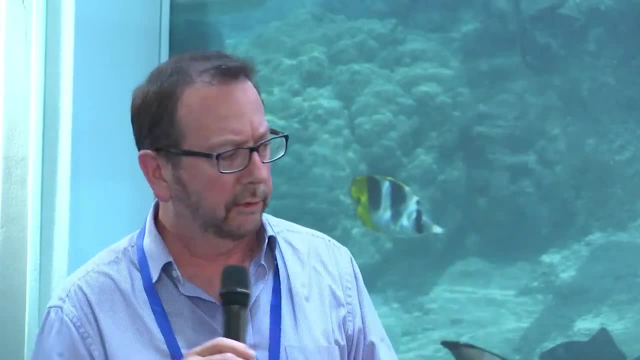 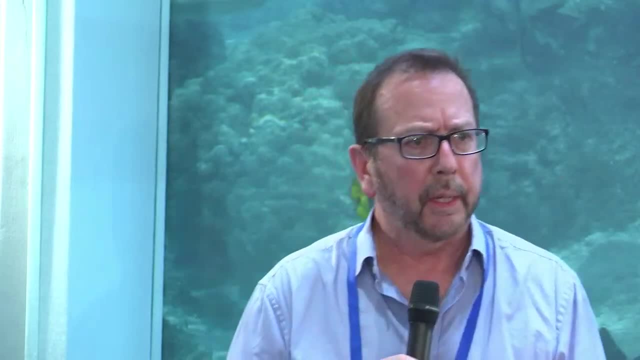 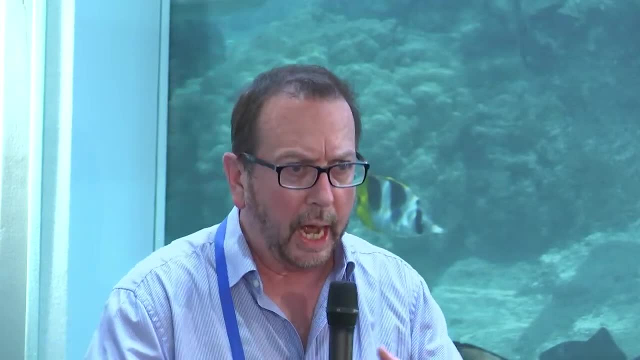 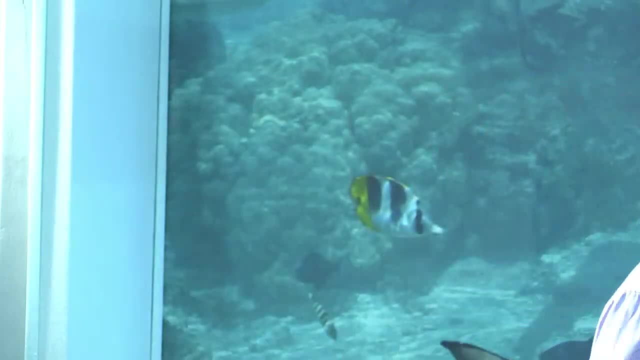 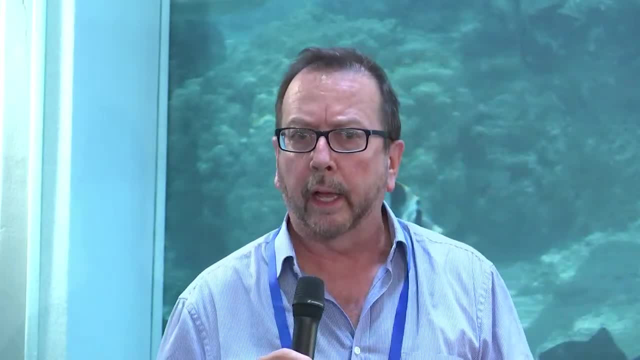 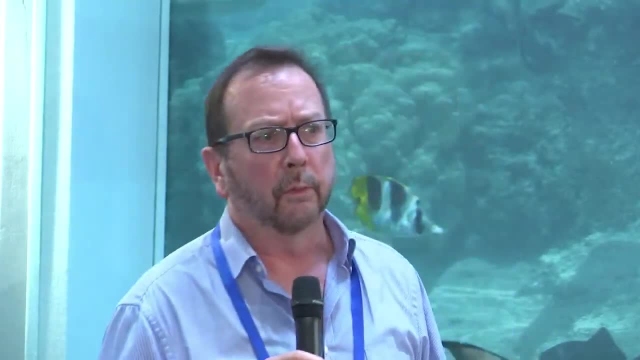 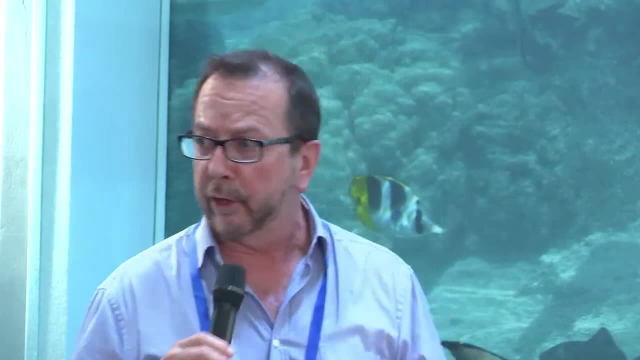 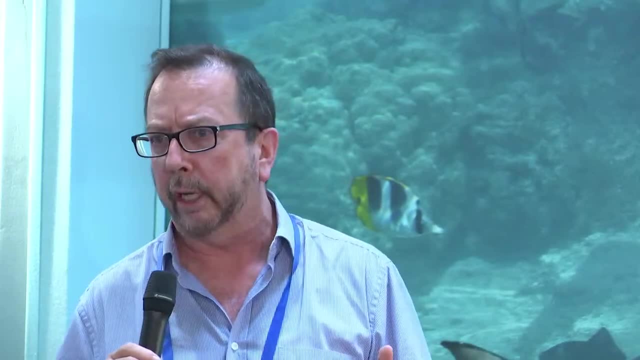 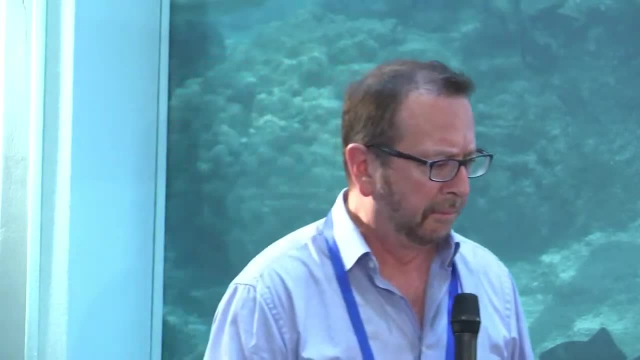 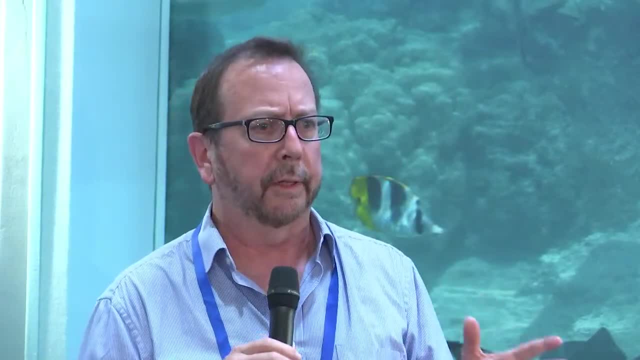 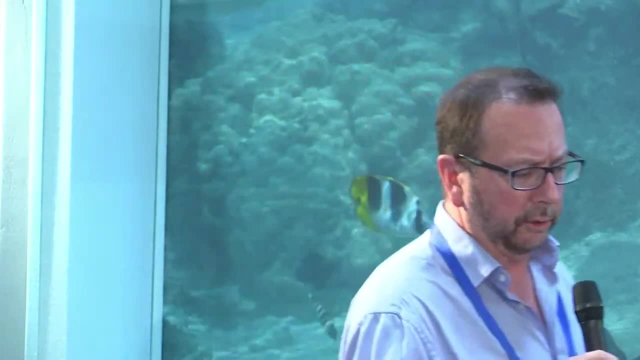 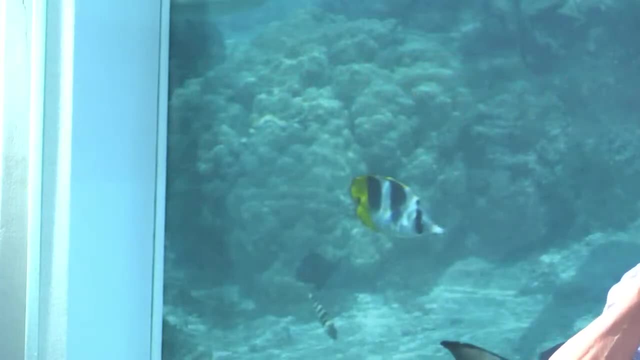 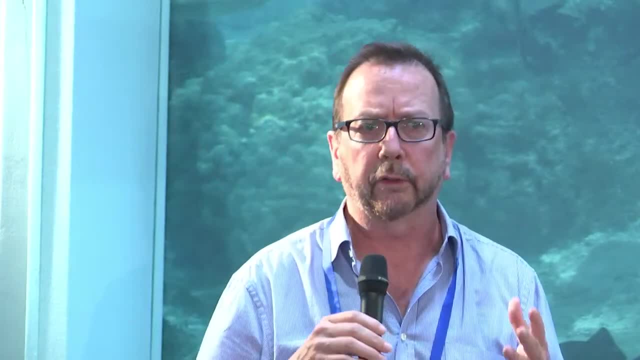 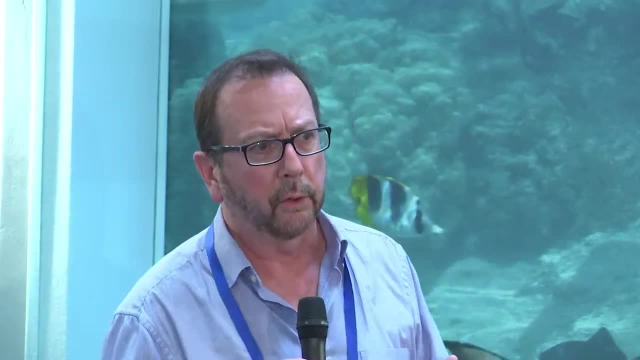 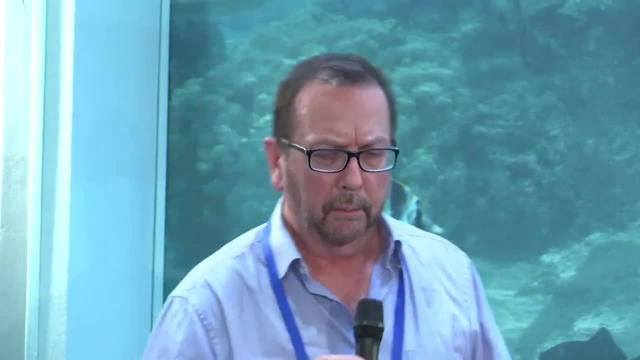 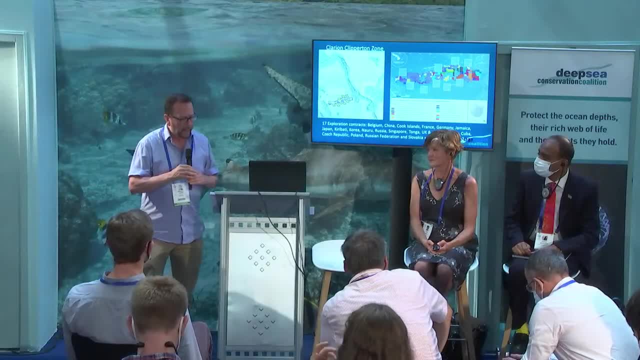 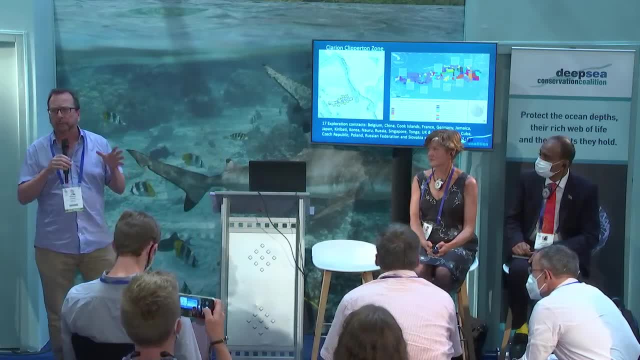 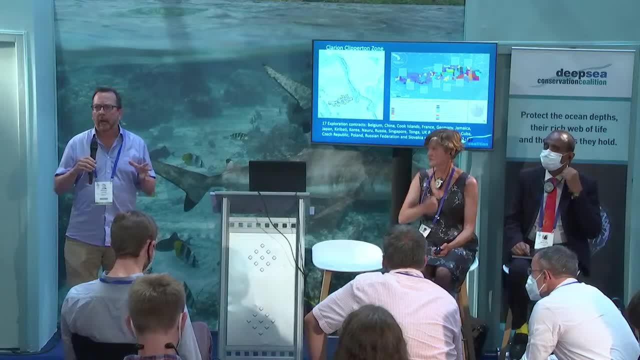 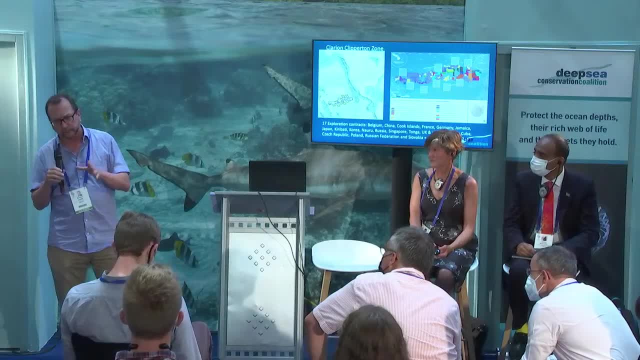 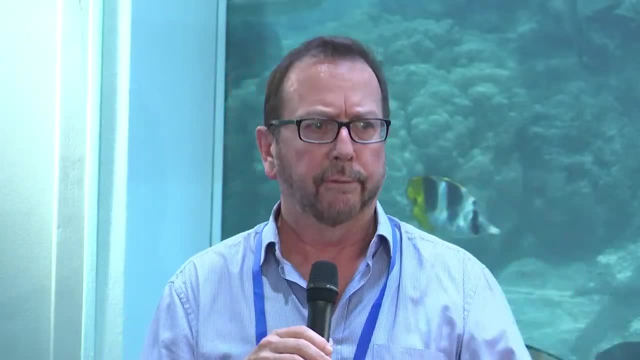 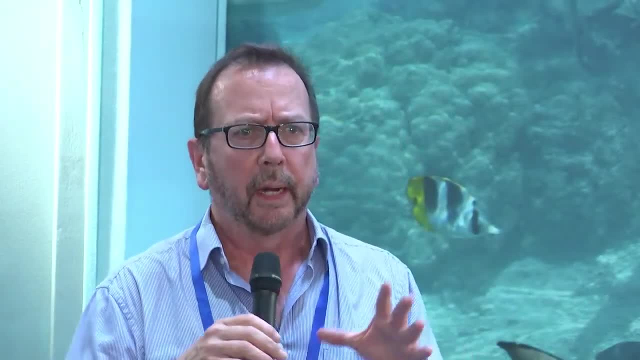 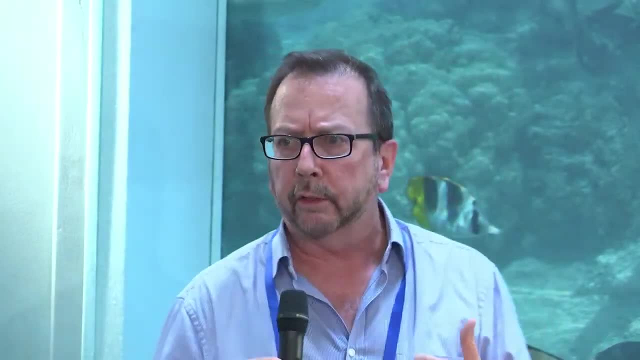 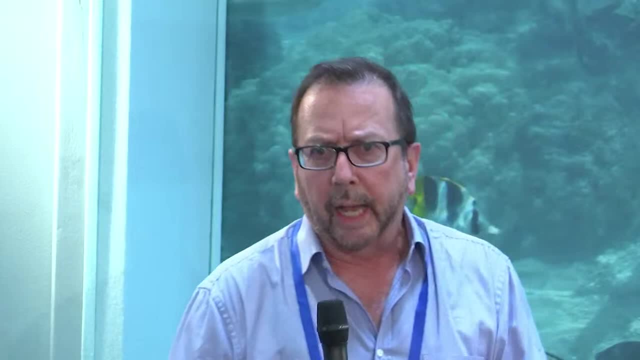 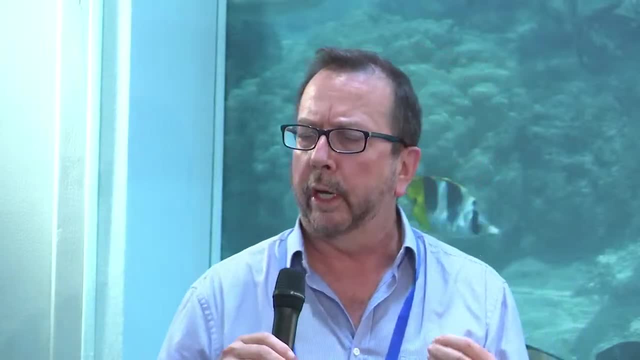 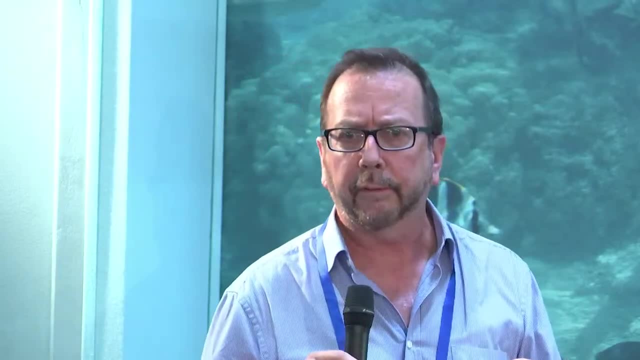 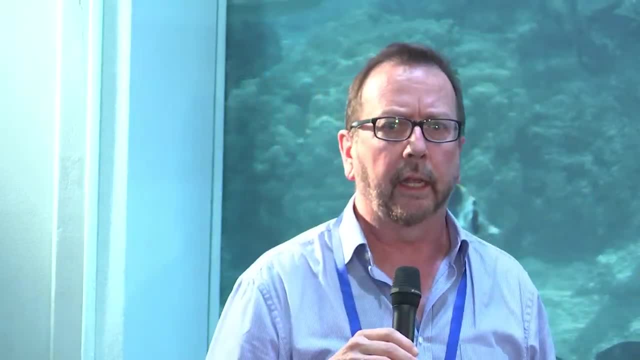 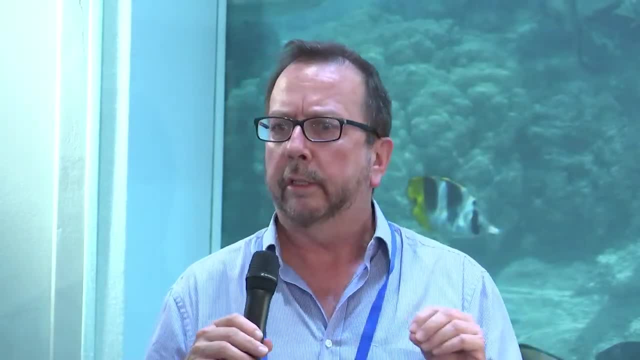 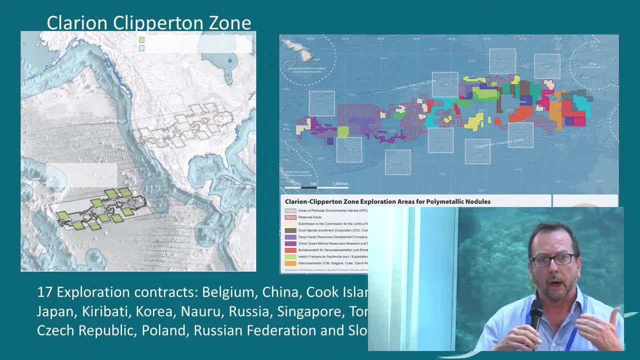 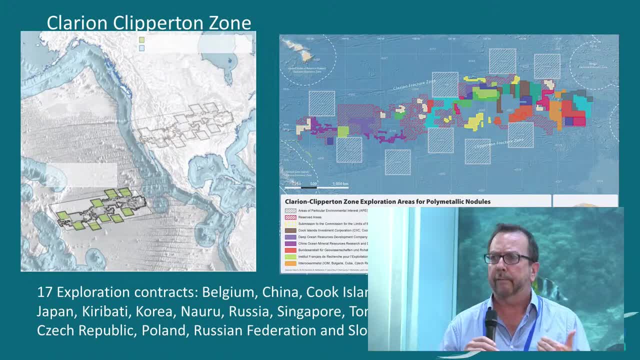 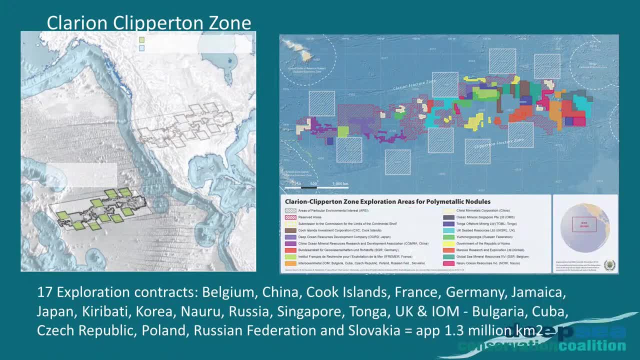 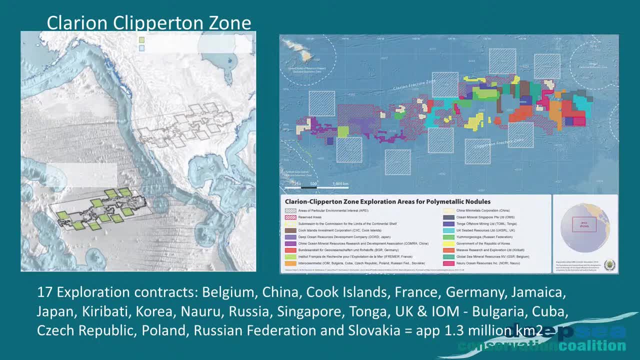 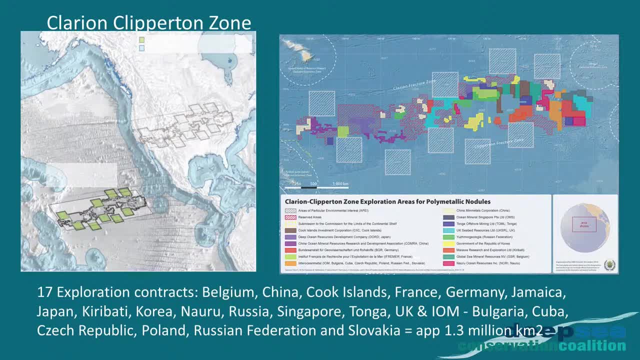 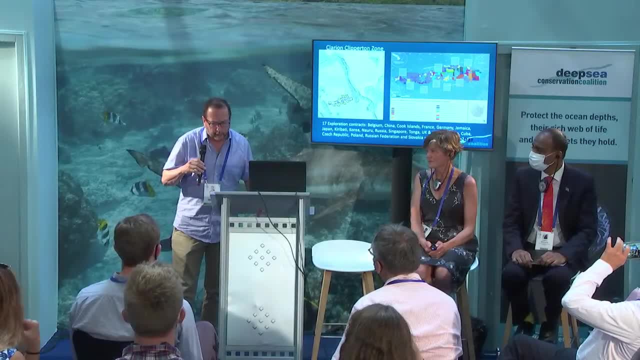 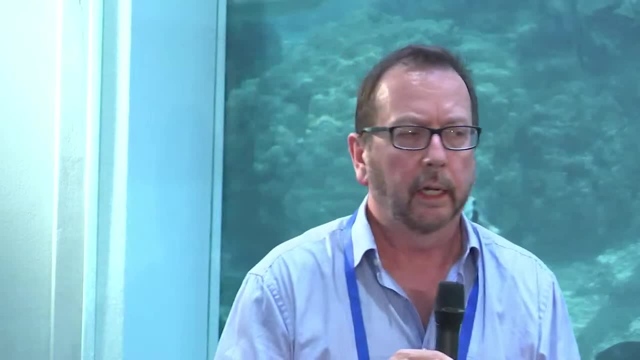 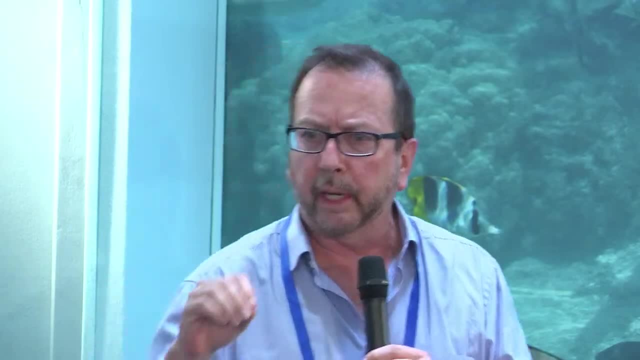 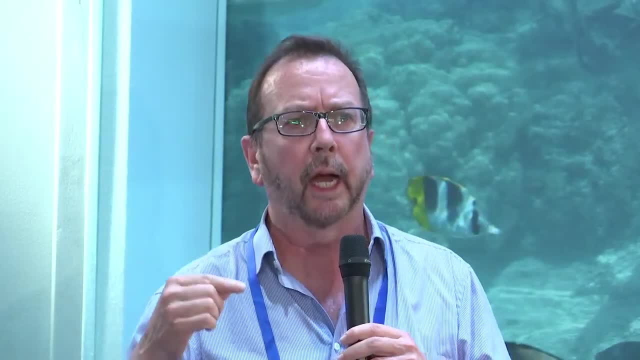 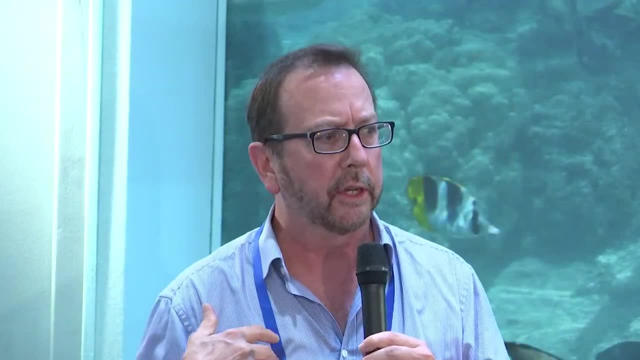 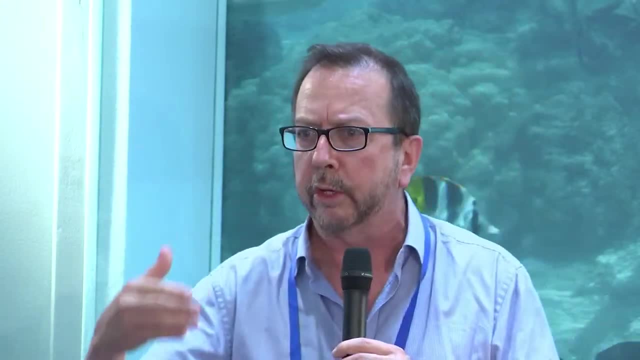 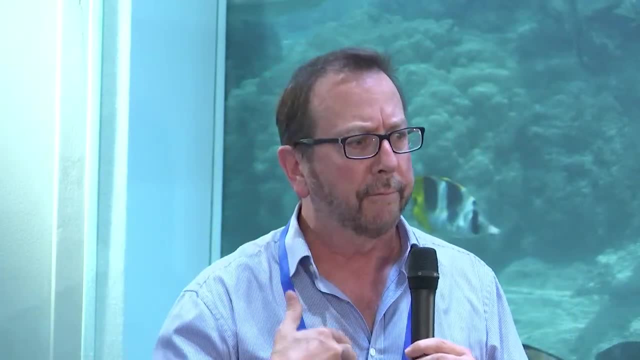 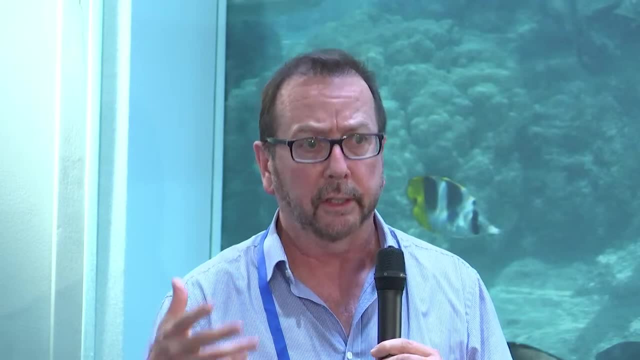 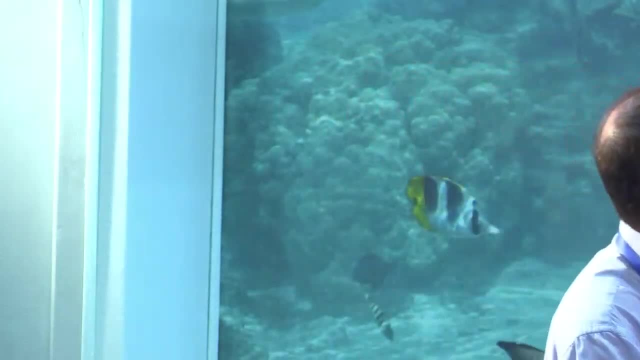 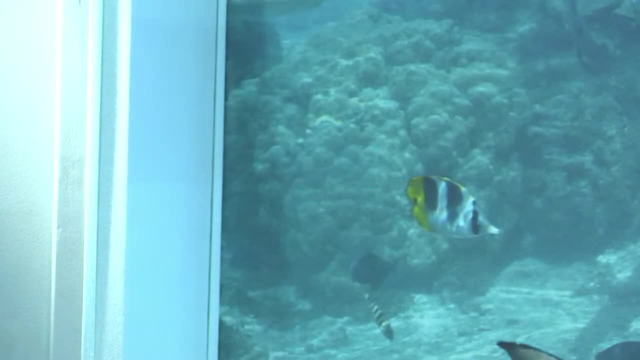 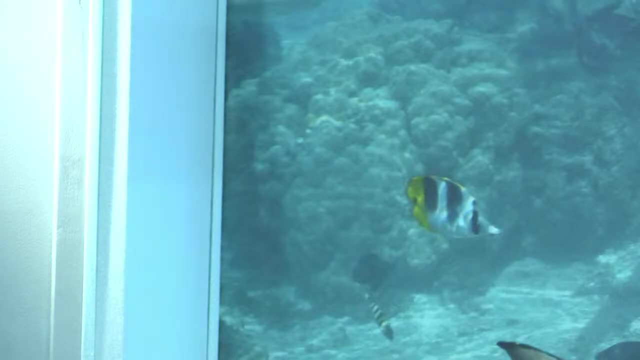 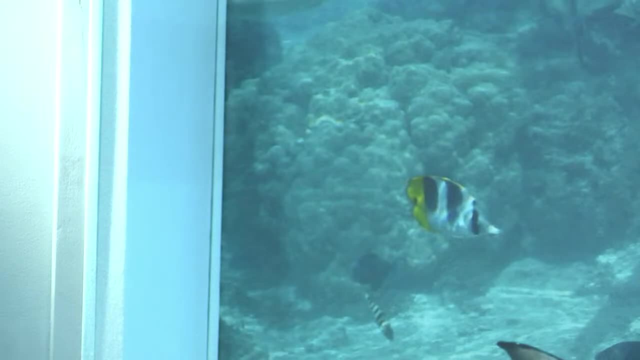 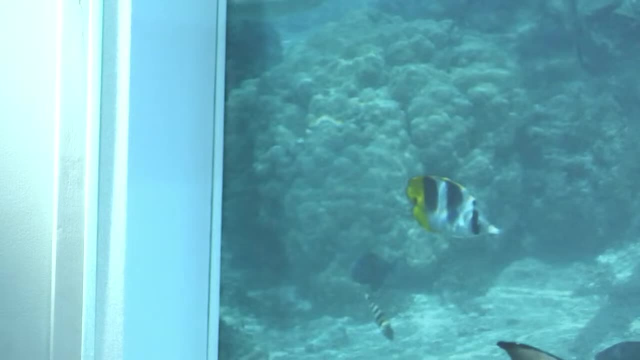 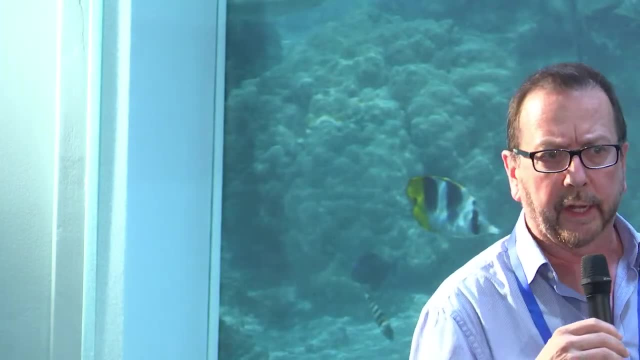 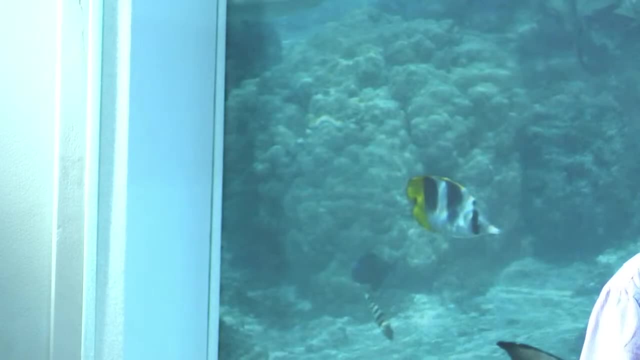 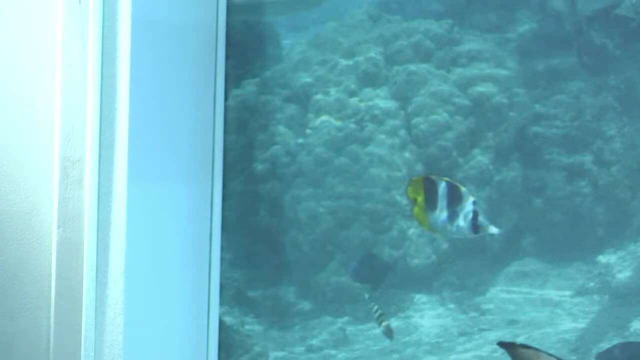 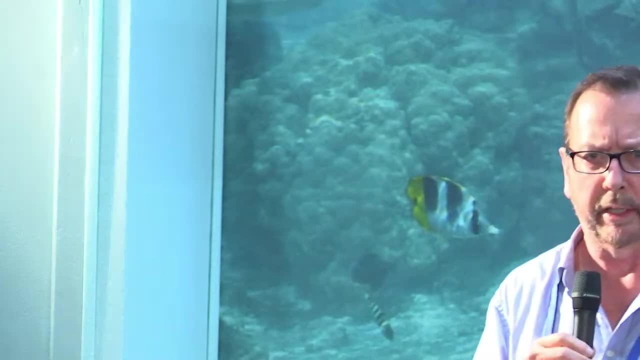 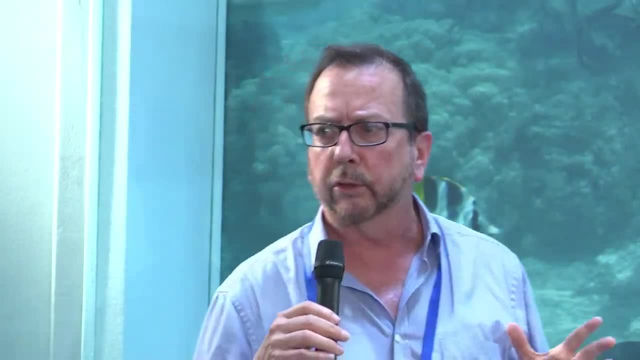 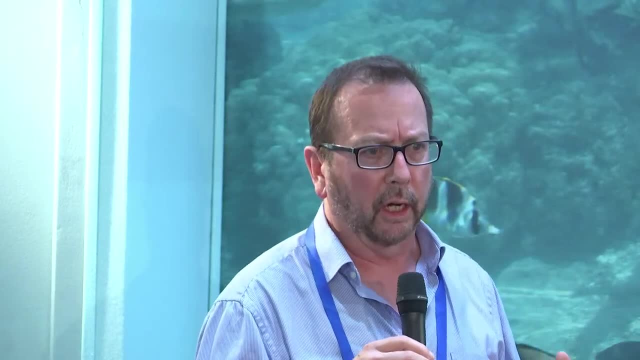 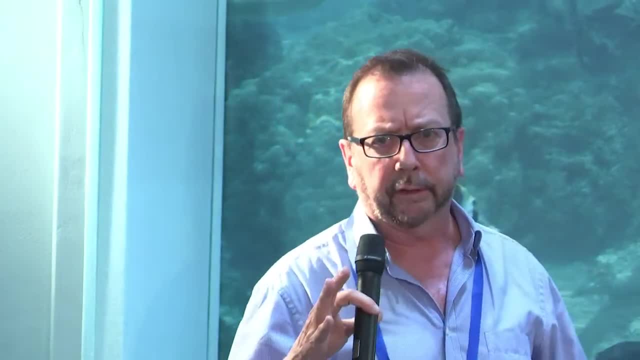 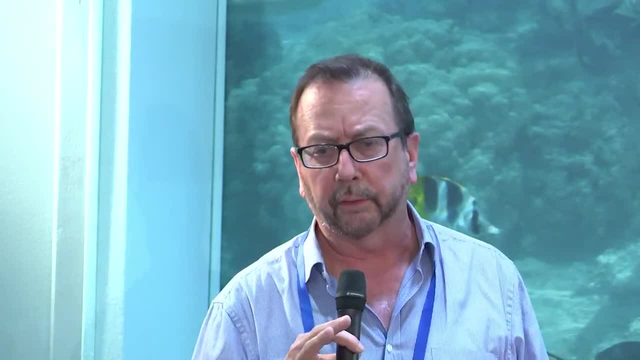 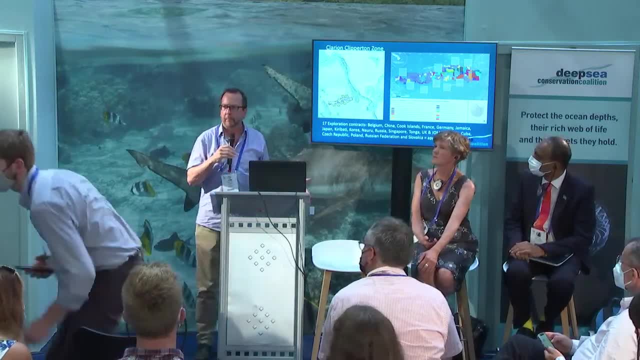 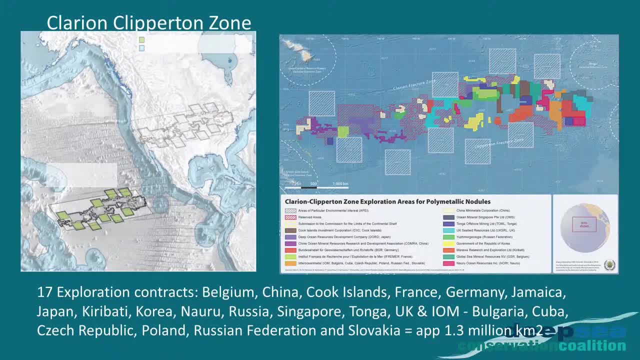 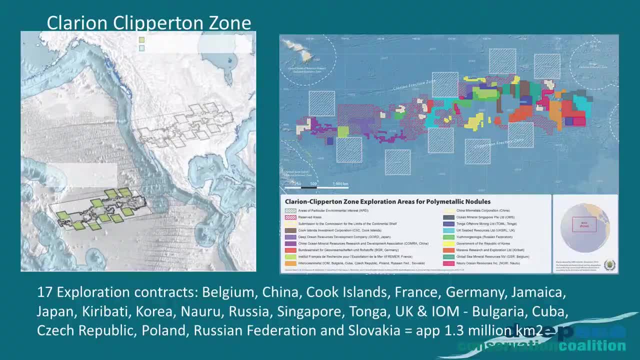 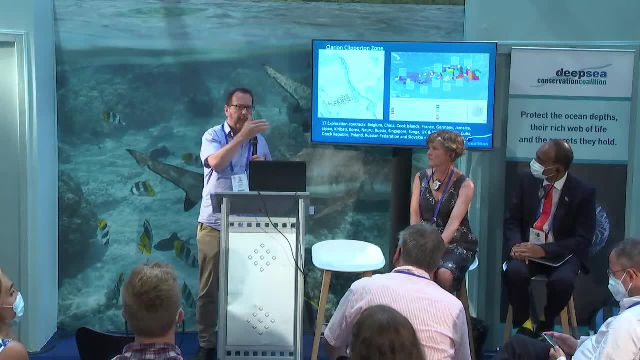 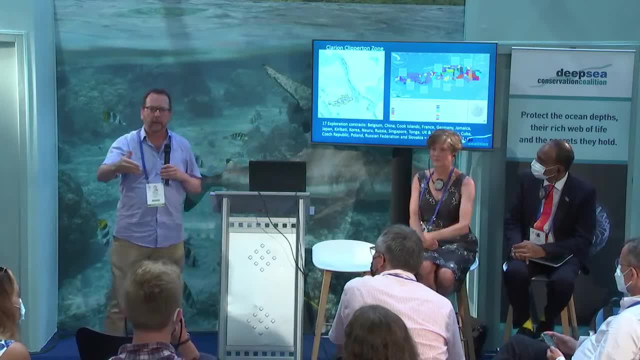 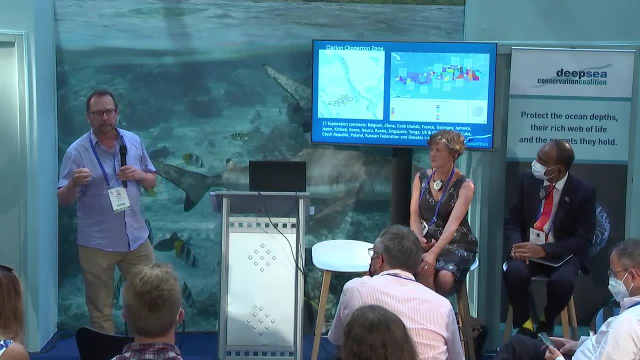 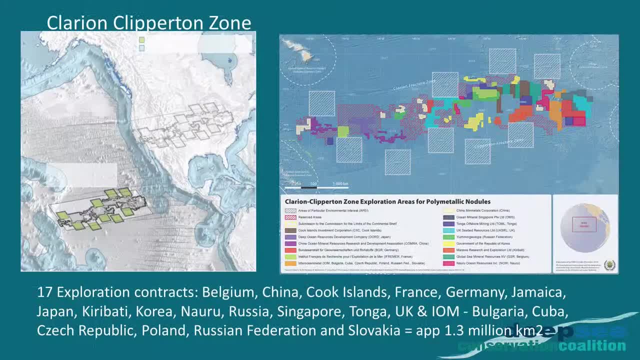 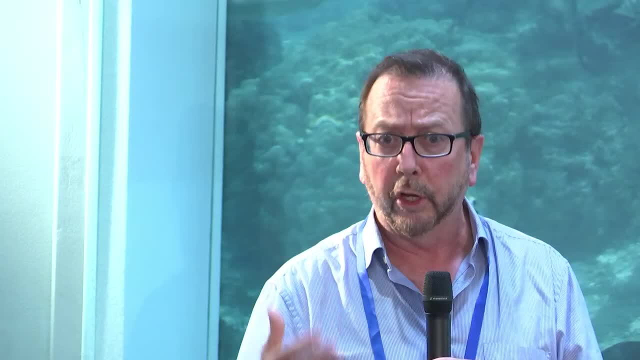 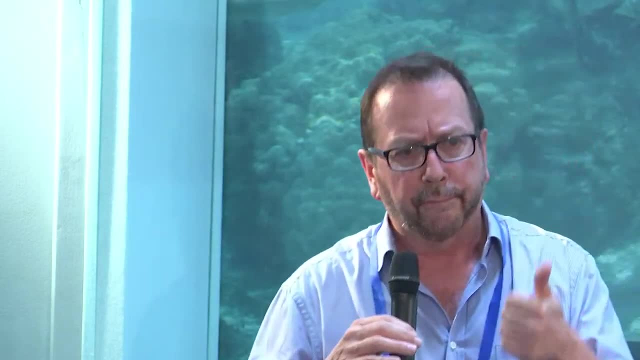 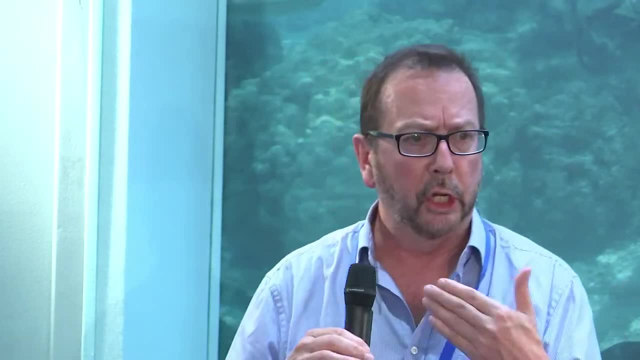 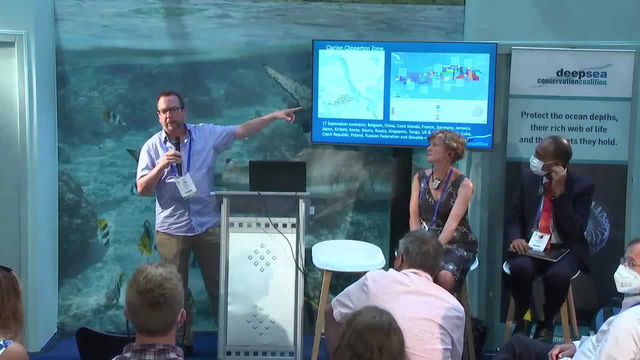 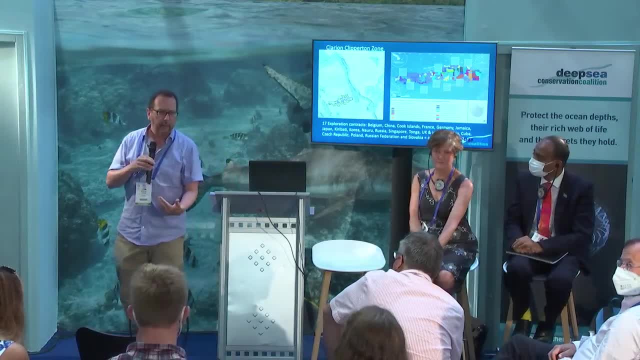 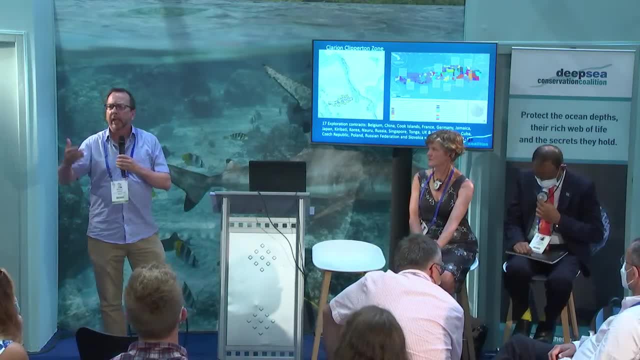 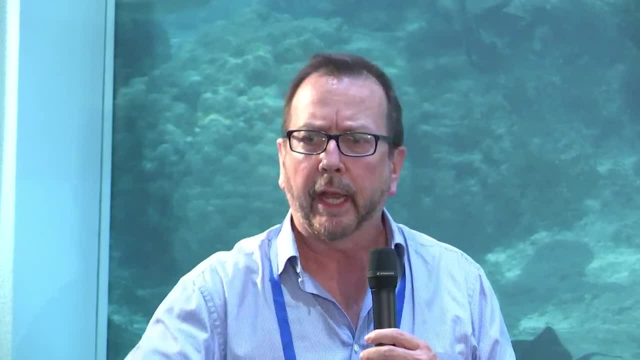 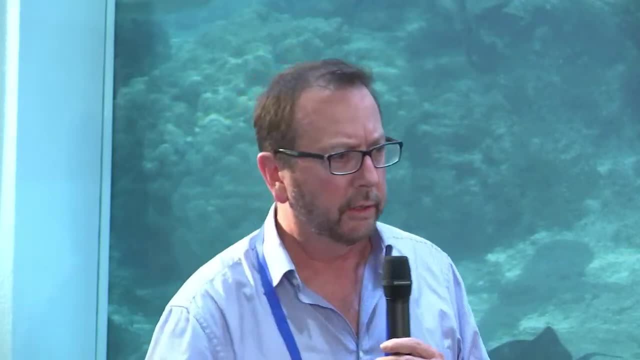 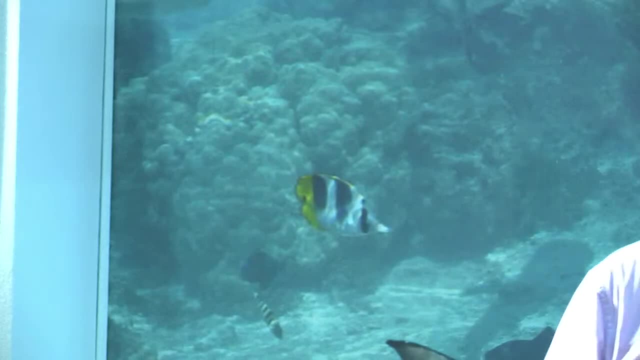 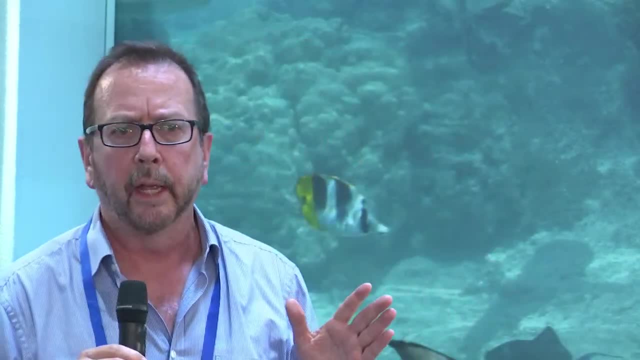 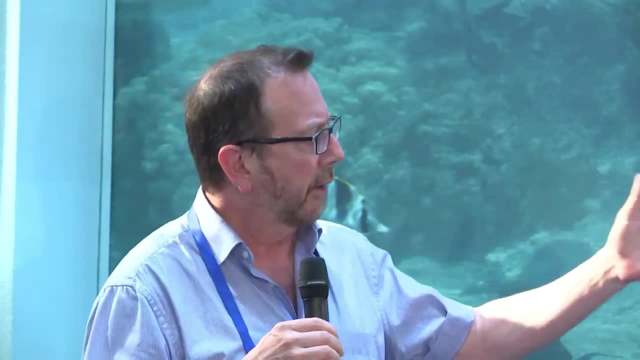 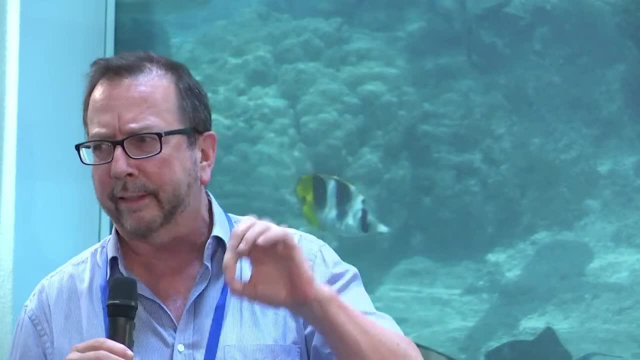 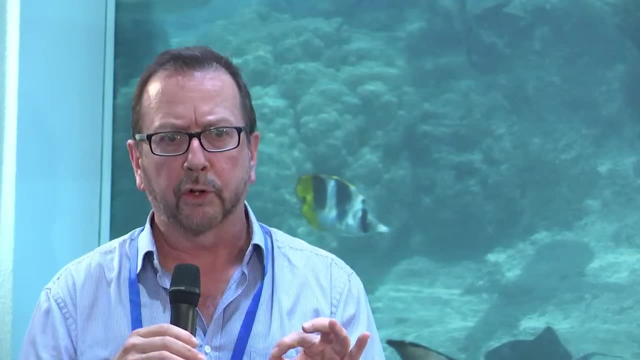 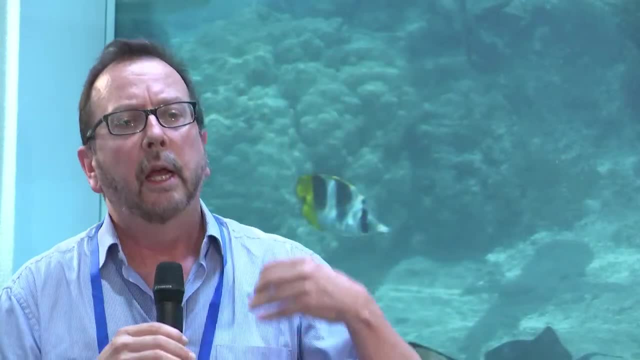 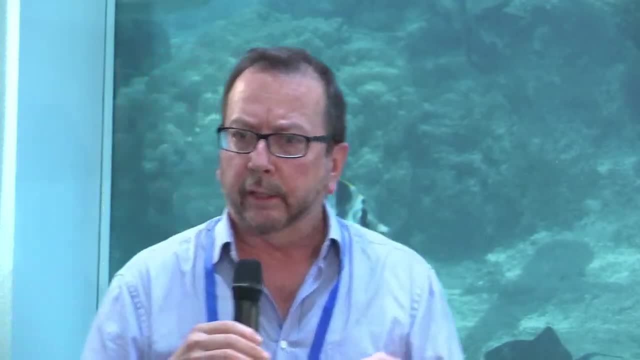 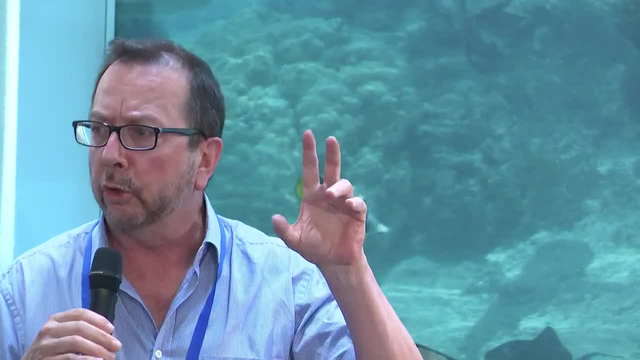 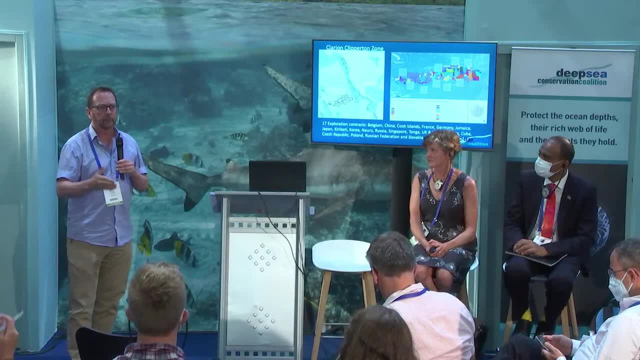 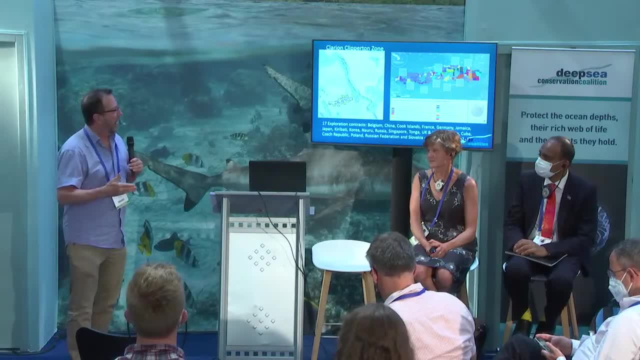 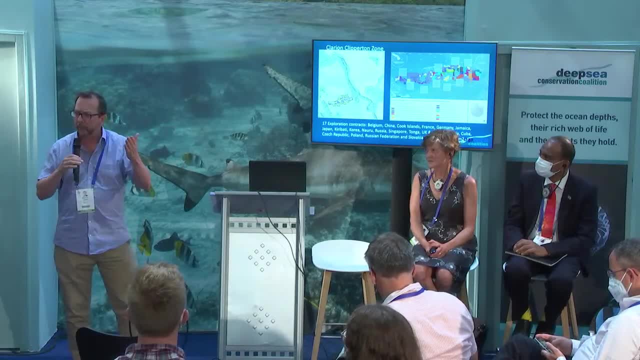 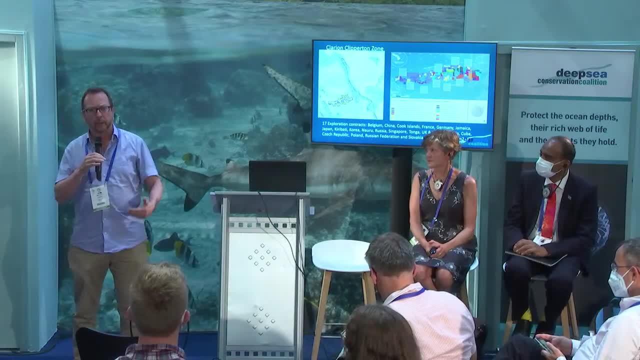 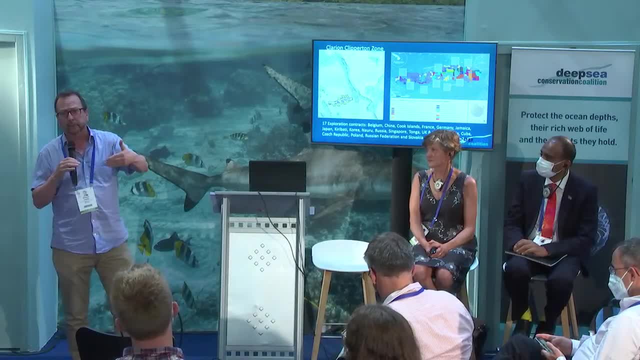 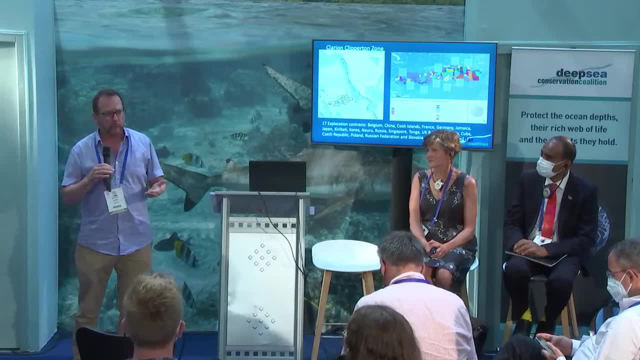 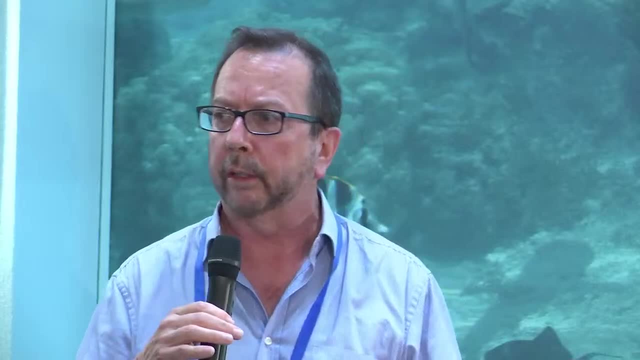 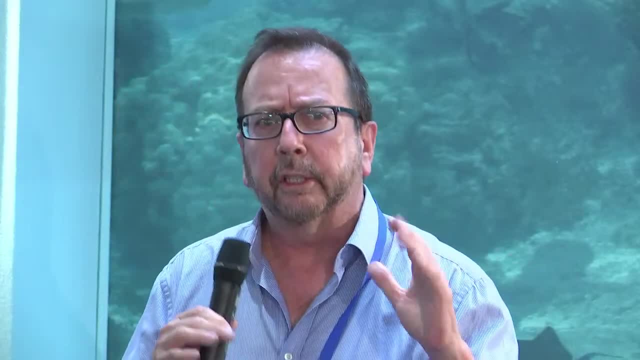 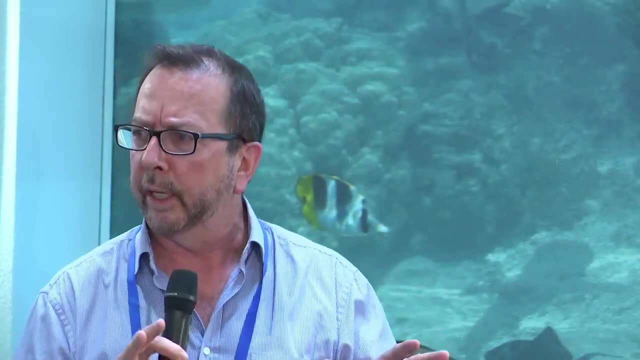 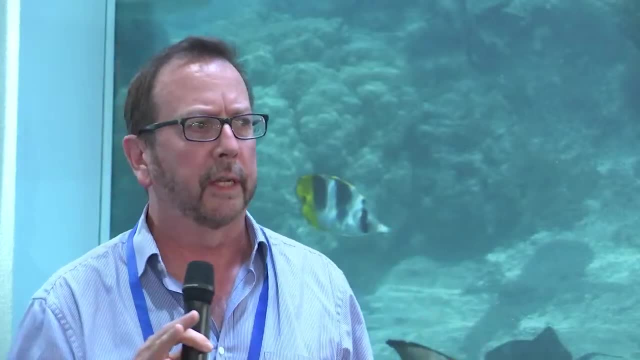 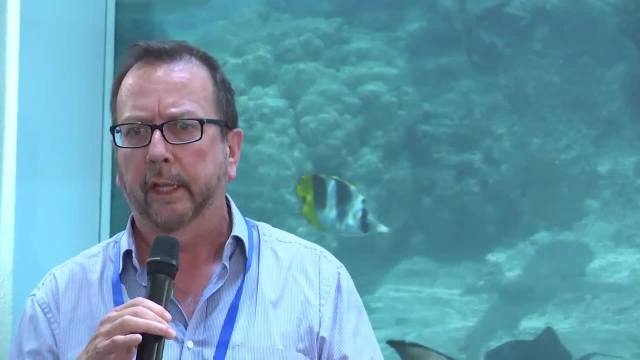 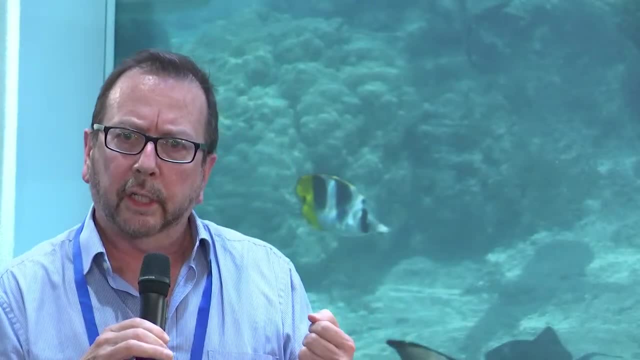 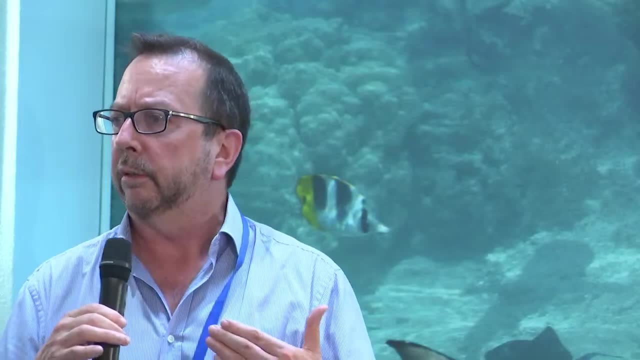 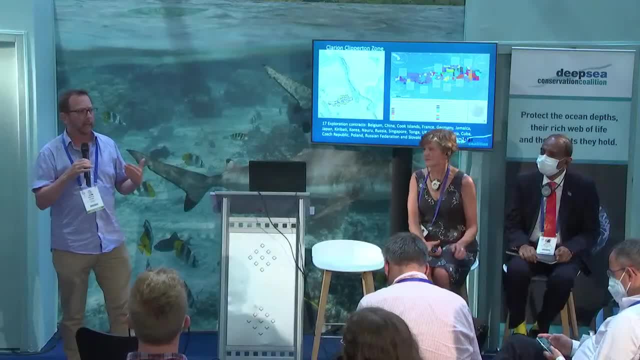 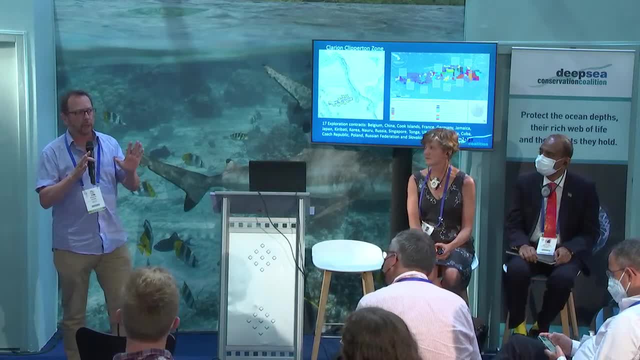 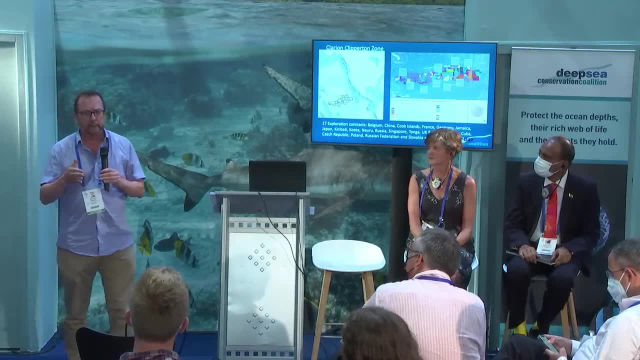 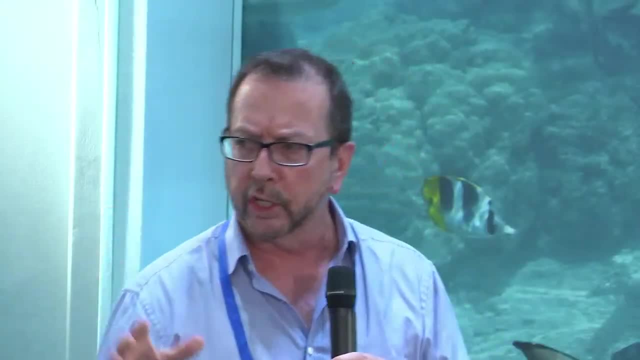 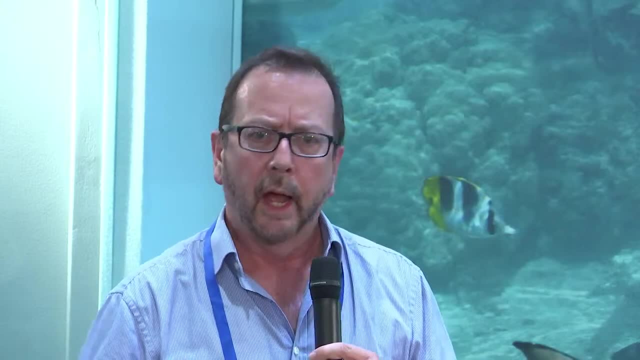 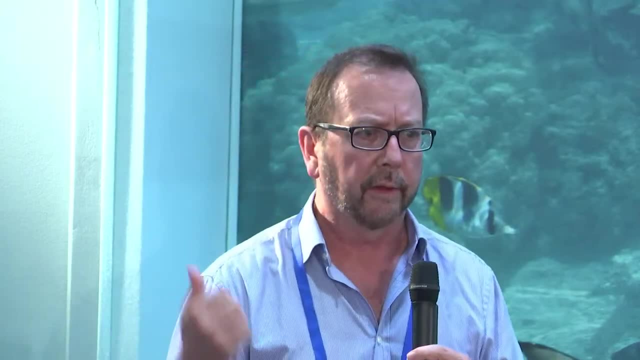 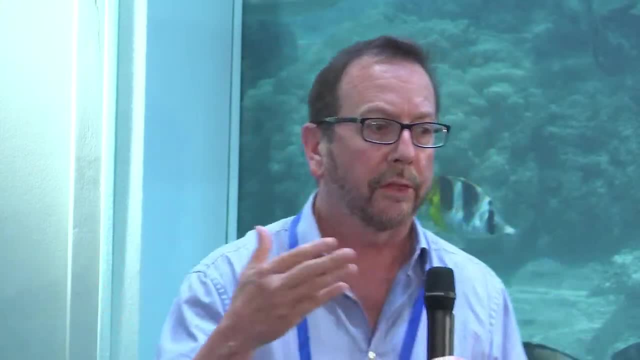 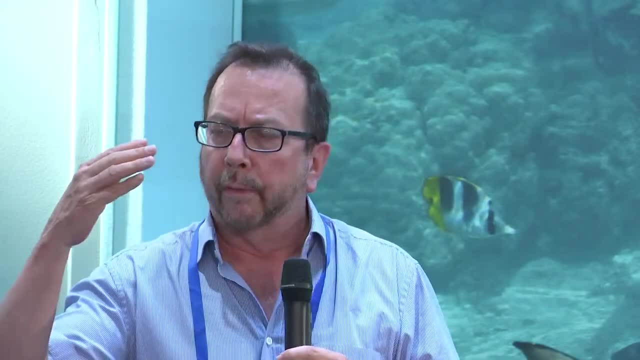 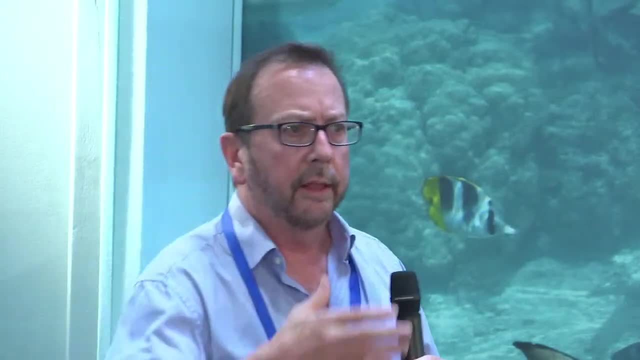 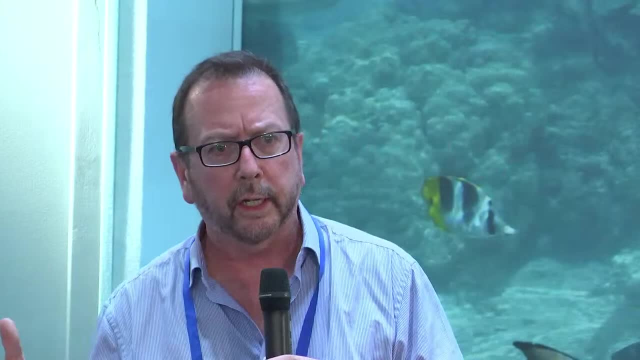 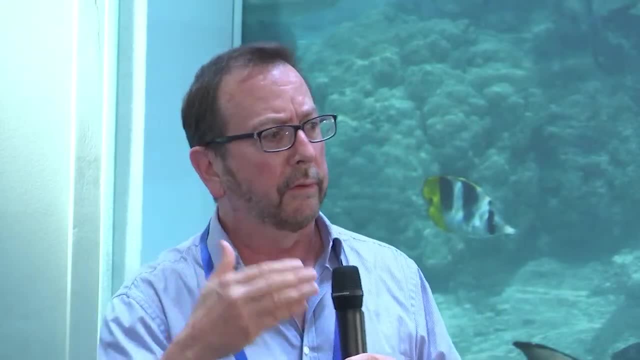 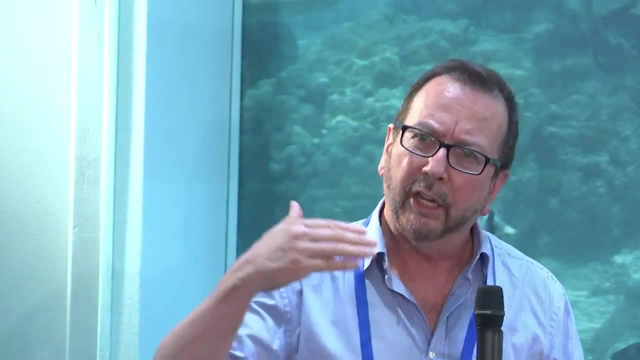 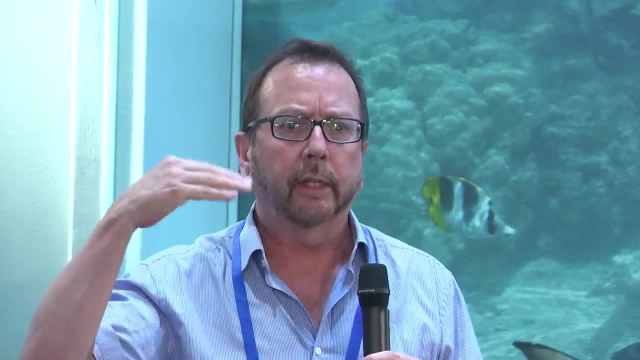 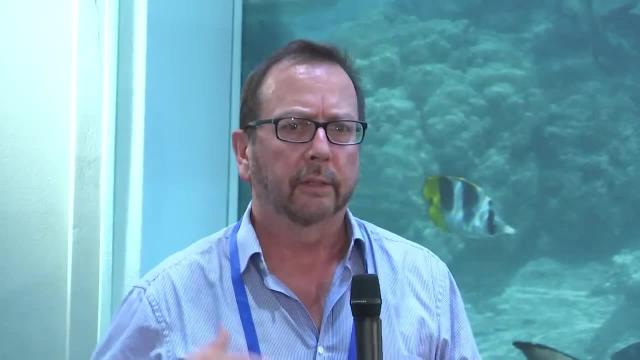 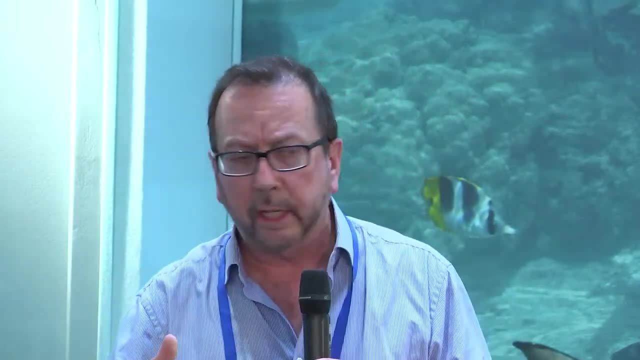 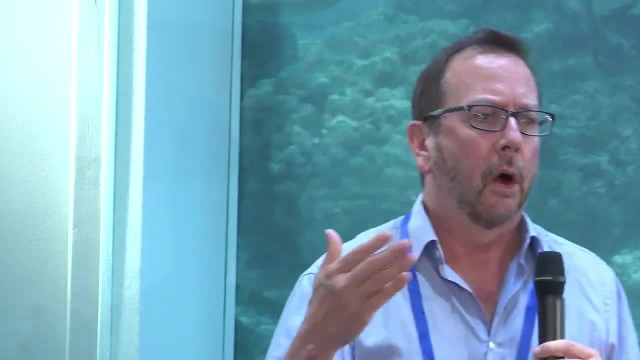 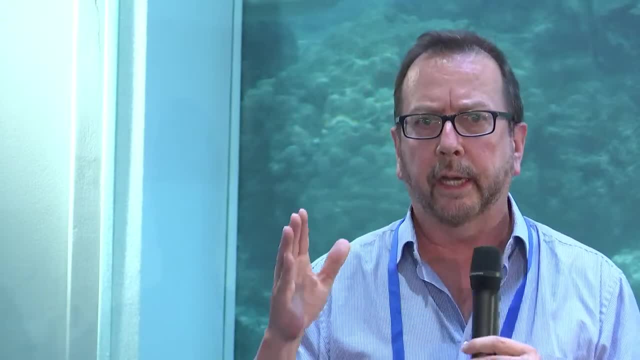 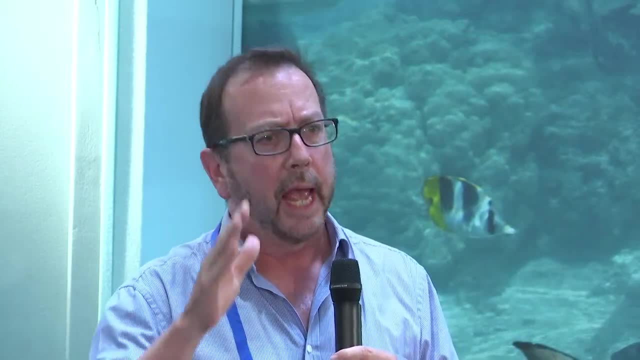 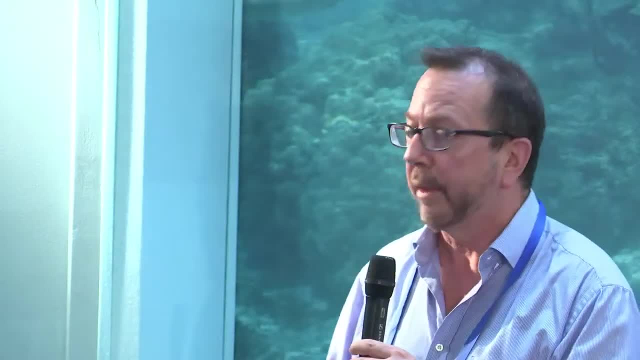 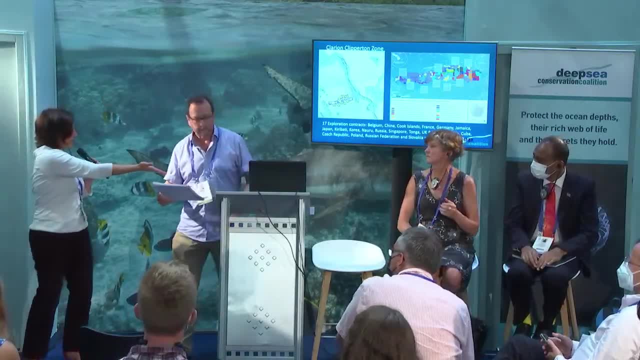 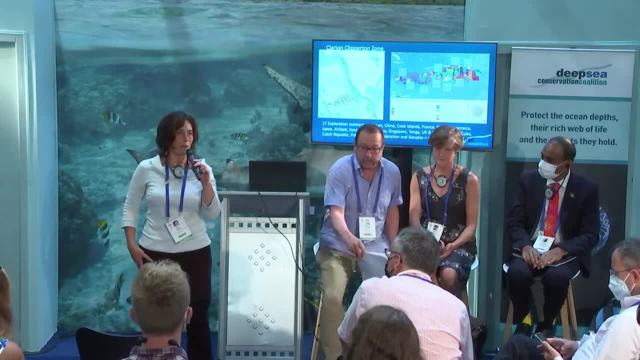 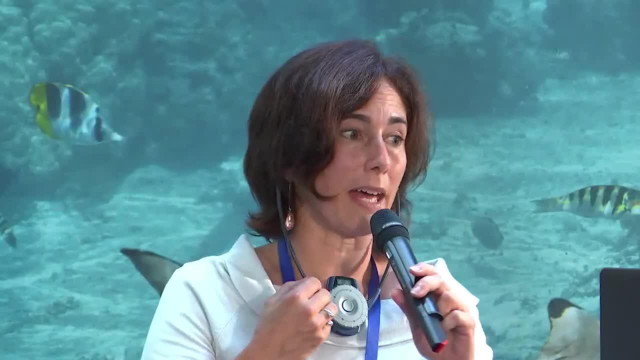 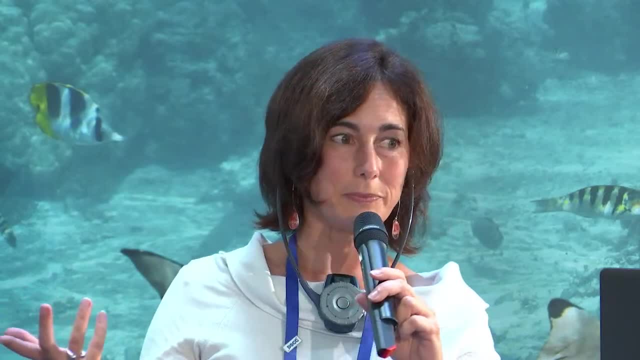 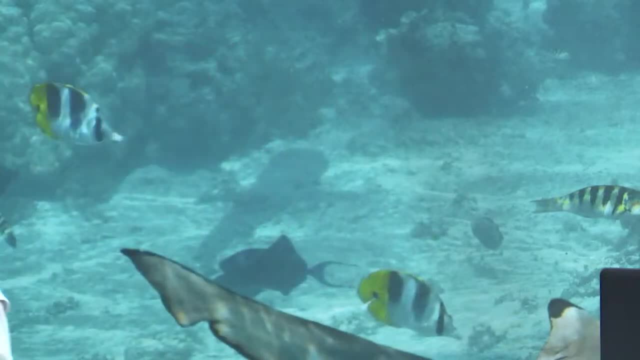 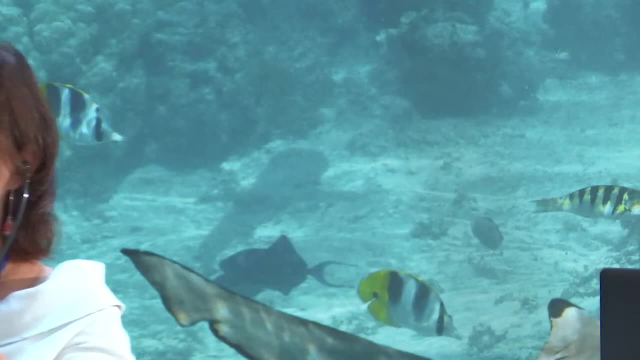 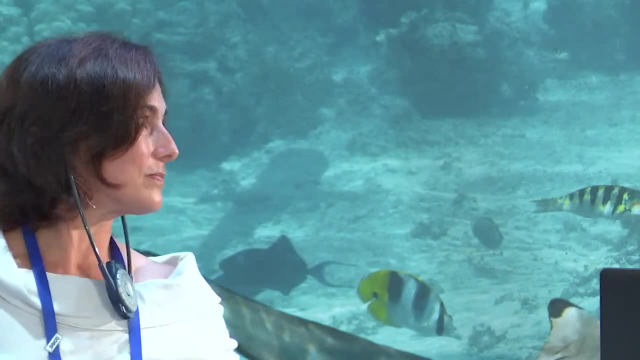 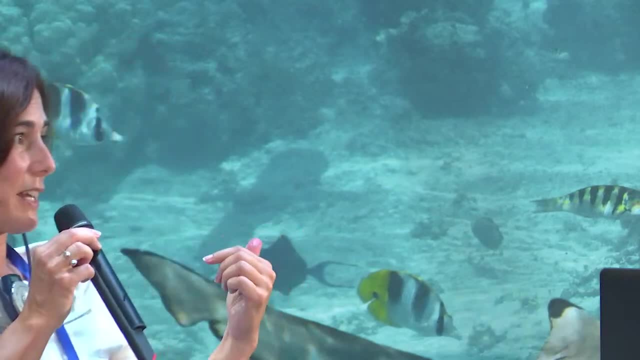 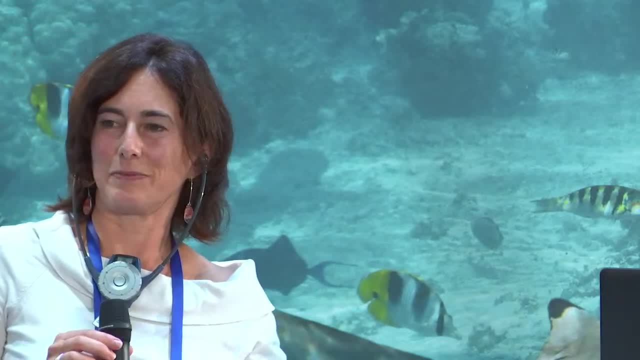 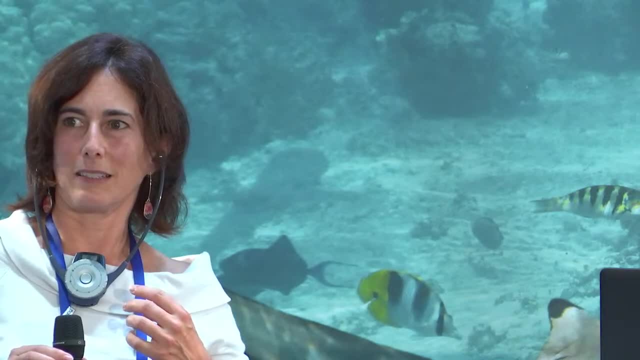 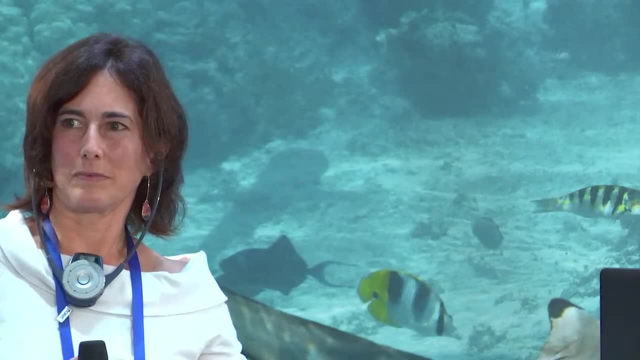 We're going to start with a very brief film to take you into the deep sea. I believe we haven't figured out how the new treaty will interact with existing sectoral management bodies such as the ISA. Do you have any prediction on how the two 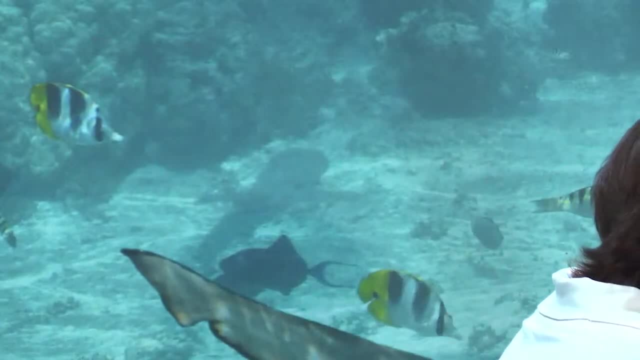 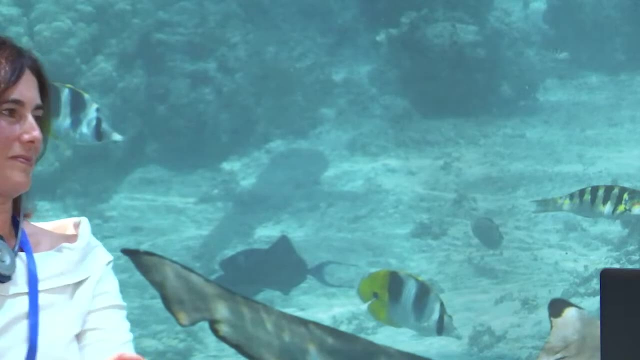 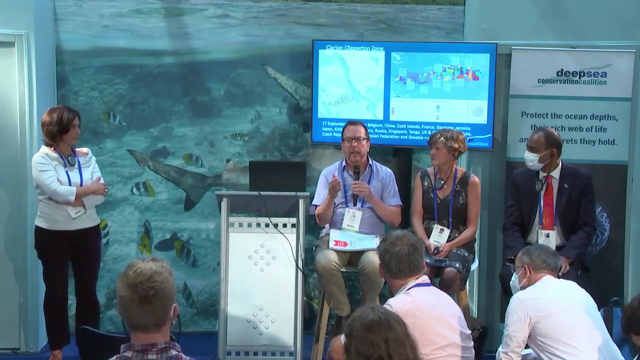 instruments could interact constructively. Thank you, You have a very good question. This is an interesting question and we're trying to promote a recognition there as well. So the BBNJ process is a process established by the United Nations under the auspices of 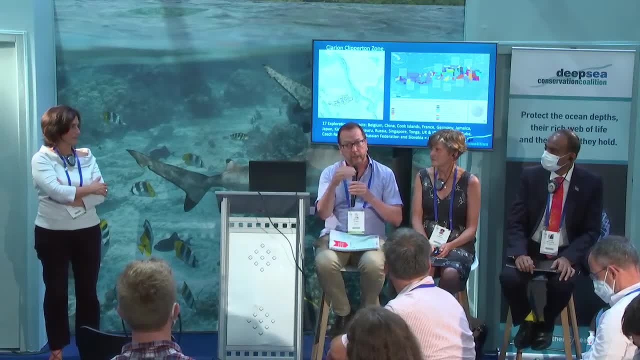 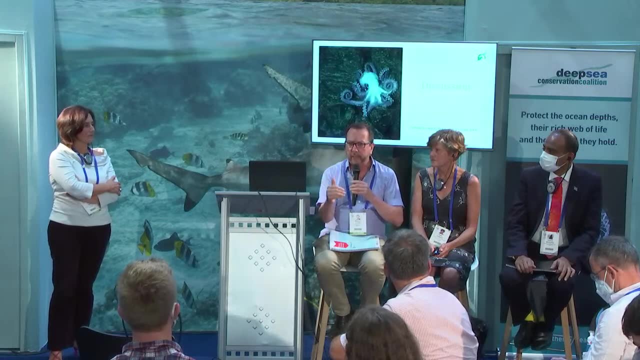 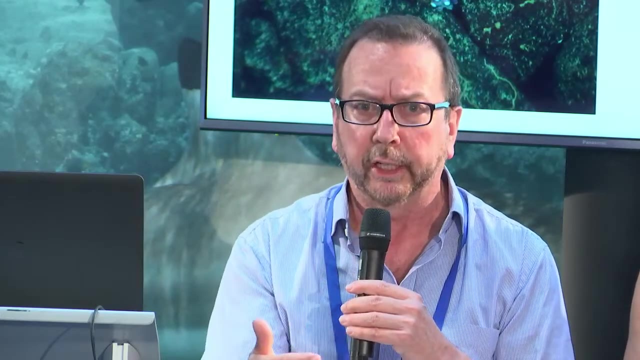 the UN General Assembly to negotiate a new global agreement for the conservation and sustainable use of biodiversity in areas beyond national jurisdiction, And the same countries involved in those negotiations are largely involved in the negotiations at the ISA negotiating a new instrument under the Law of the Sea Convention, in this case. 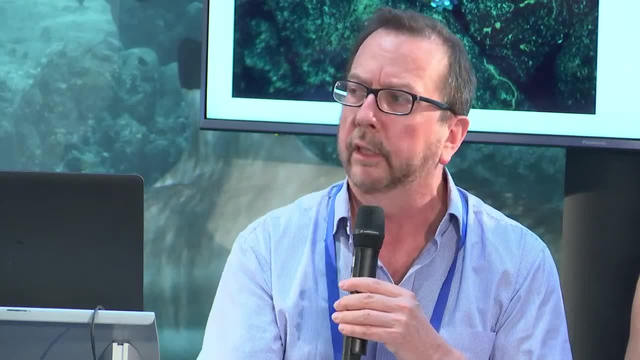 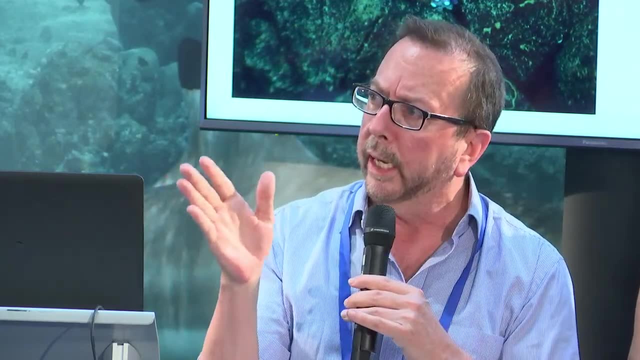 the Mining Code. that will lead inevitably to biodiversity loss in areas beyond national jurisdiction. So we're trying to say the right hand needs to know what the left hand is doing. But more importantly, I think most of the member nations of the UN are involved in the 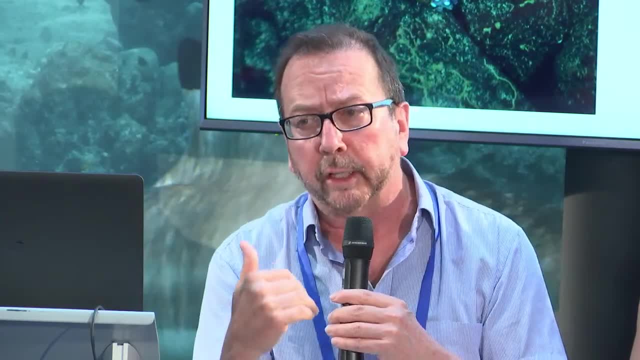 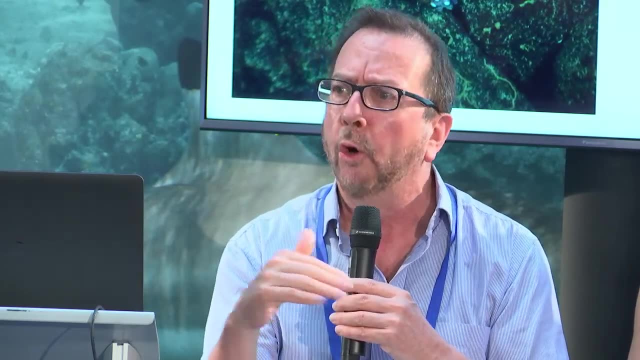 BBNJ negotiations. One of the real weaknesses of the International Seabed Authority is that only about half of the member countries actually show up to the meetings, And so that gives a kind of a home court advantage to the mining interests to be able to push. 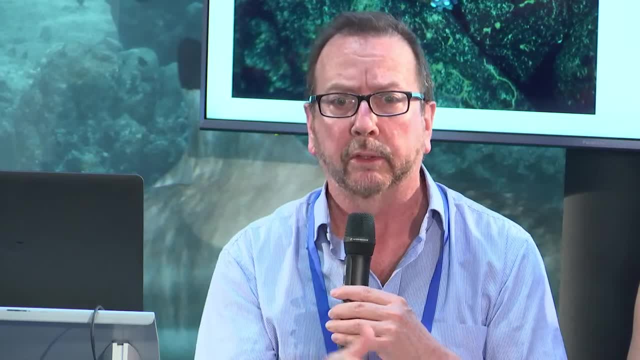 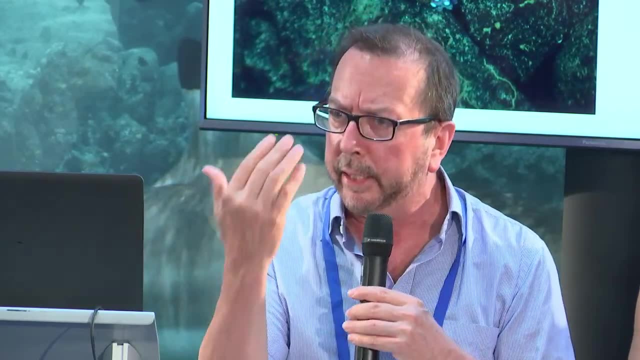 through mining regulations because much of the rest of the world isn't paying attention to what's going on down there. And again, the World Conservation Congress is a great opportunity. It's an opportunity to raise awareness with environment ministries. The CBD coming up is another opportunity to say hey, you know contracting parties to 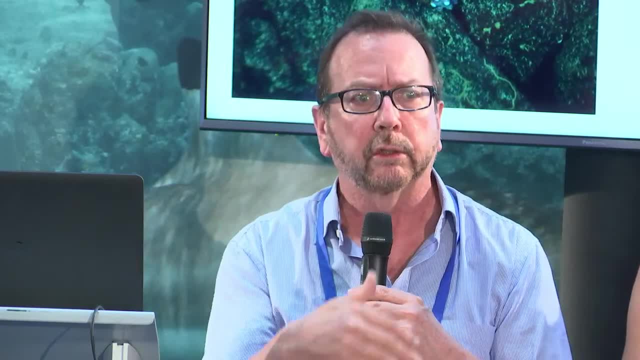 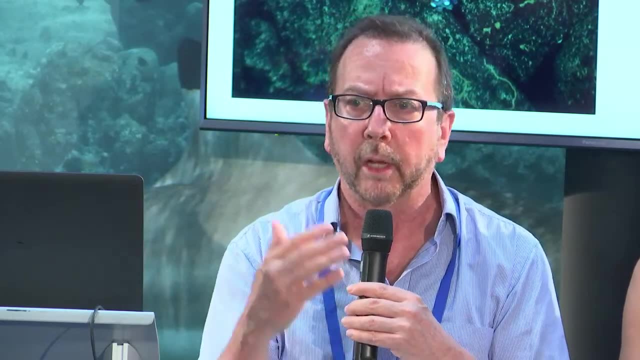 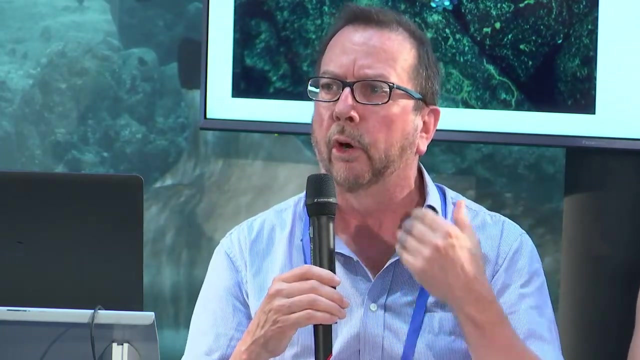 the Convention on Biological Diversity. in your coastal and marine decisions, in your global biodiversity framework decisions, you need to be calling for a moratorium on deep seabed mining, Biodiversity losses will inevitably occur, et cetera, And that's what we're hoping to try to use the BBNJ process for the CBD process for. 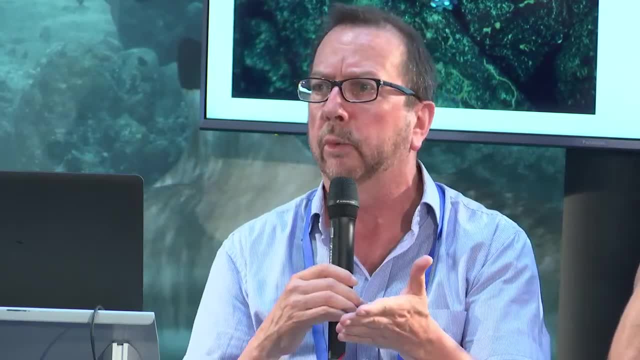 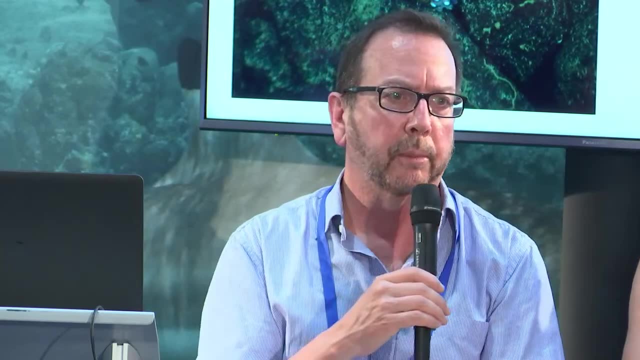 the UN Ocean Conference next year in June of 2022.. Thank you, And ultimately get a decision out of the ISA member countries as participants at the ISA to put the brakes on the process. Thank you for that question and for your response, Matt. 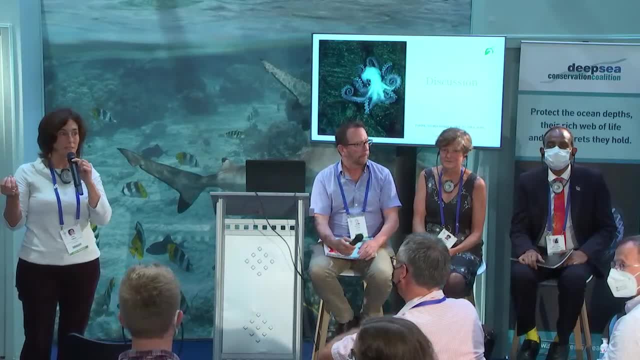 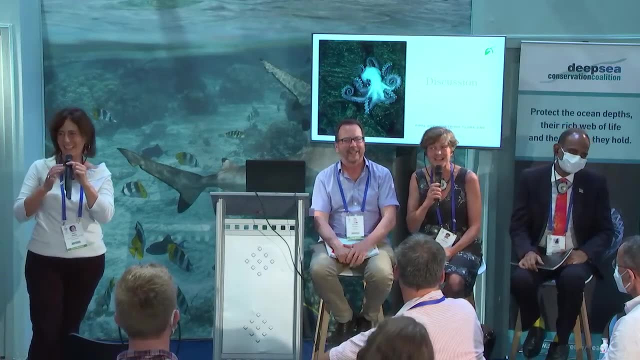 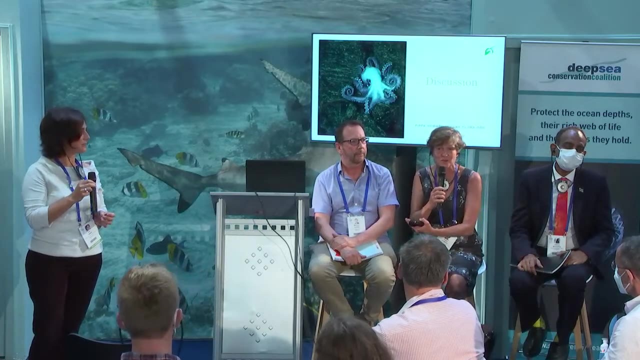 Any other questions or comments. I think we've shocked everybody into submission. Yeah, Yeah, It's a very stark reality. in actually taking you through, you know not only the governance that's being fought with with difficulties right now, but also the pace that things are. 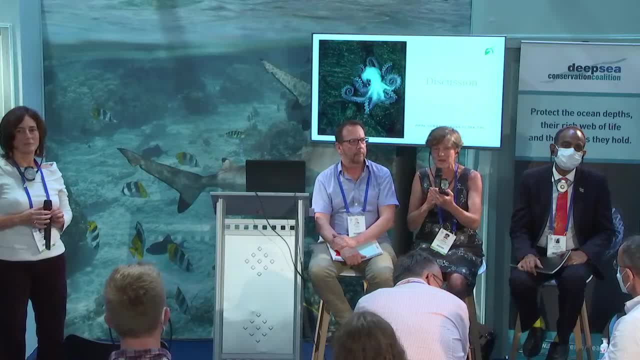 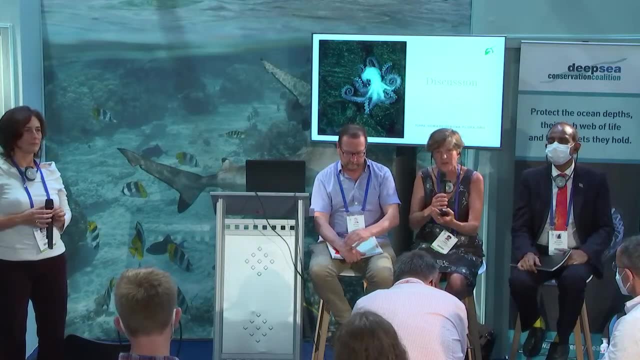 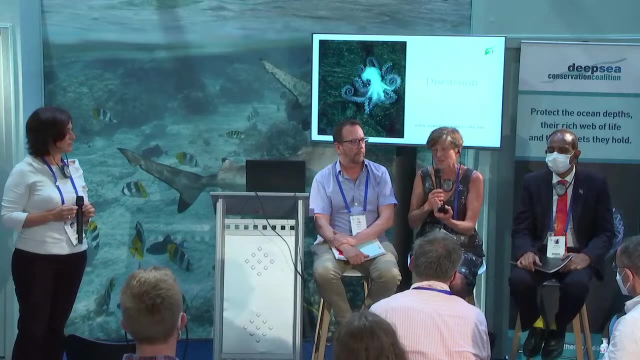 the pressures are coming on by the two-year rule trigger by, you know, the lack of engagement and the social license to operate. Most of us don't know that actually this is even a proposed industry, let alone know what the ramifications and repercussions might be. 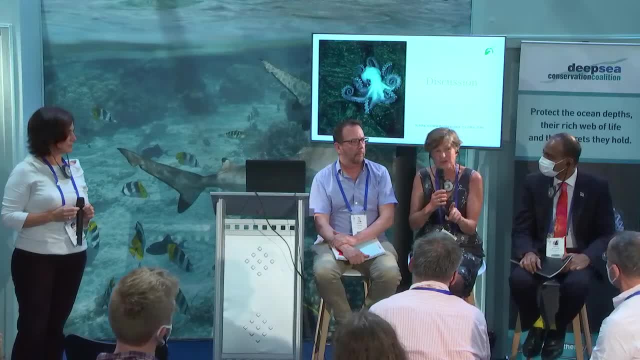 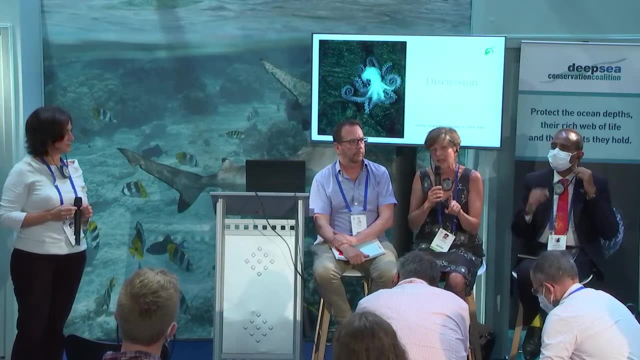 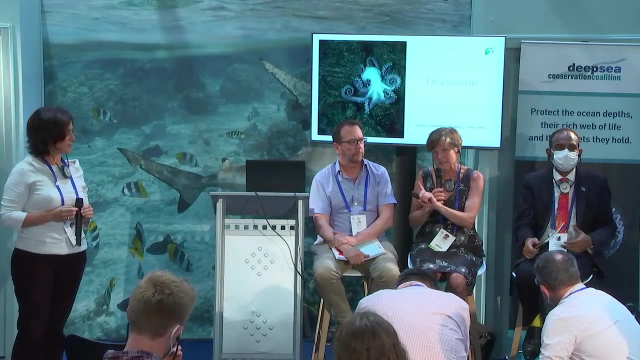 And just to add, Sean, if I may, to: if we think of, oceans are connective. they're a continuous system, They are absolutely fundamental. They're the lungs and the heart of our planet And when an impact from one of those concessions takes place, it's connected through big ocean. 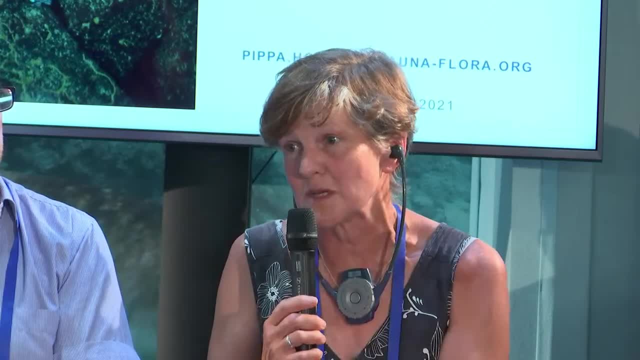 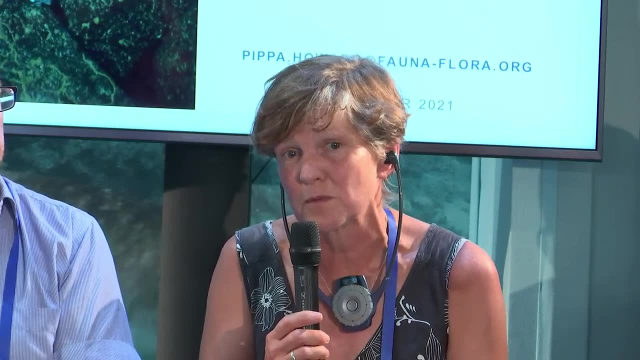 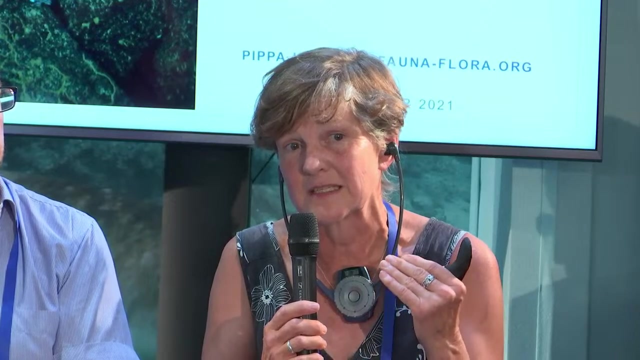 systems, not only around the oceans, but, you know, three-dimensionally, you know through the water column and can spread throughout the global system. Also, the kind of fundamental role that the ocean plays- Yeah, The, the, the oceans play in climate regulation and the whole biological pump is at risk. 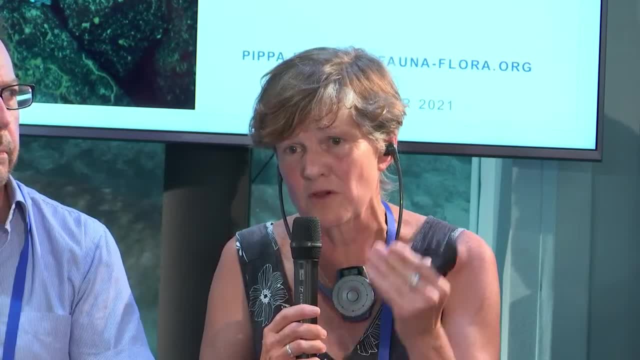 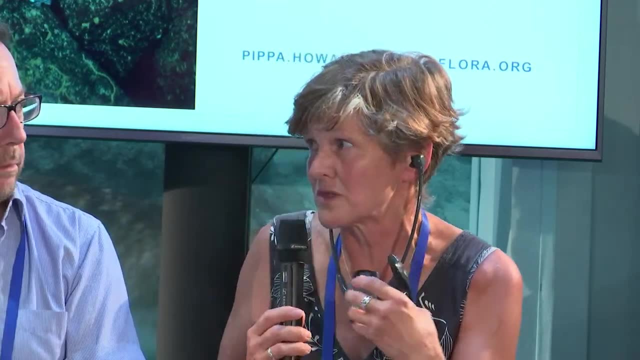 And we know from bottom trawling what the effects of loss of sediments are are doing to the kind of climate sequestration potential of our ocean beds. So you know this is disrupting, when tens of thousands of kilometers the system. 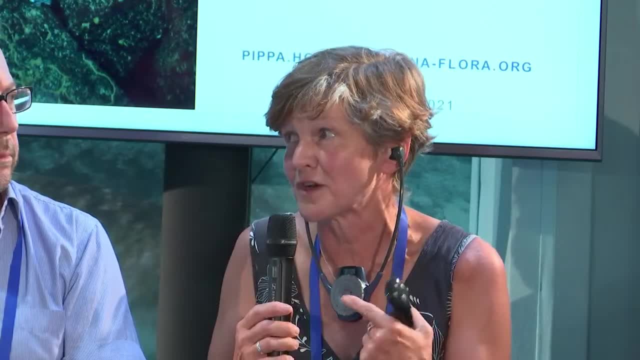 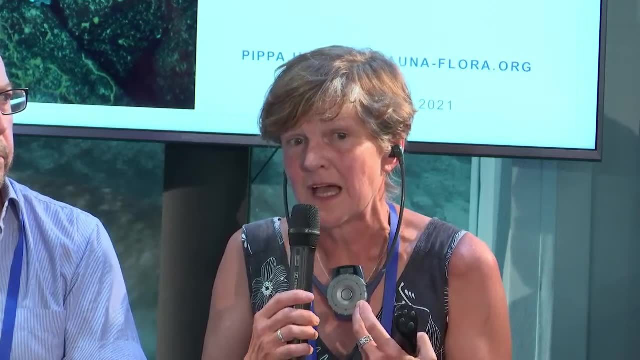 We don't understand, I don't think what the repercussions are. I remember first time I sort of started to really get into the into the nuts and bolts of the science of the ocean, Yeah, The science of, of seabed mining. 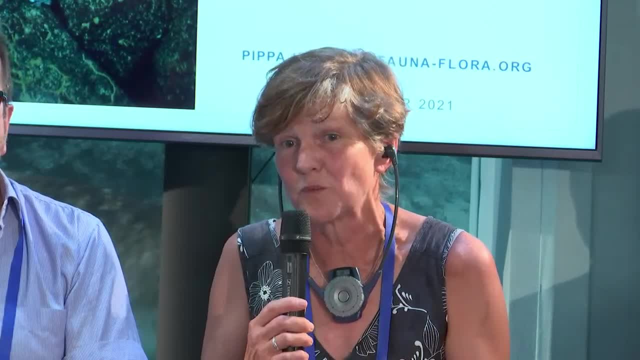 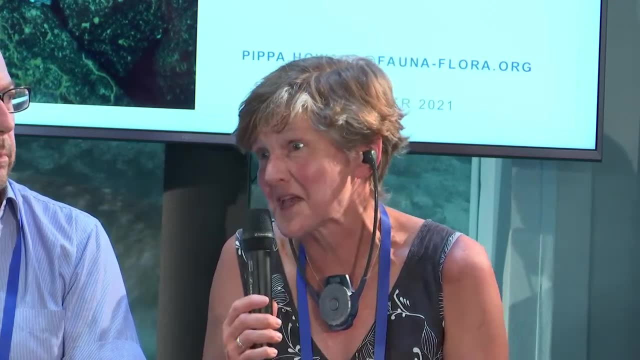 I thought this is. this is worse than climate change. If our oceans fail, we, we will fail the planetary processes of our, of our whole. you know the system will fail. So yeah, it's all a bit scary actually, yeah. 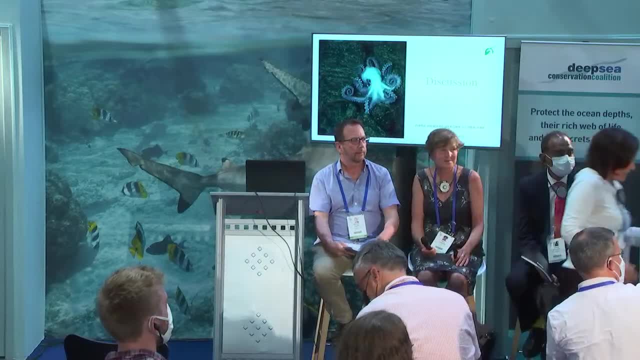 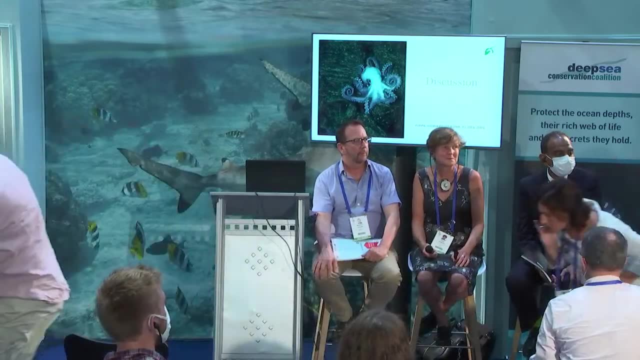 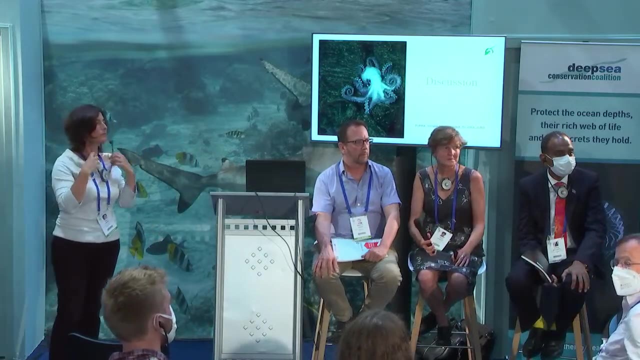 Thank you, Pippa. Yes, Hi, I don't know if you covered this, cause I don't have headphones in, but my question is: there are deep seabed mining companies. This Friday Deep Green became the metals Company and they've been very outspoken saying polymetallic nodules are just down there for. 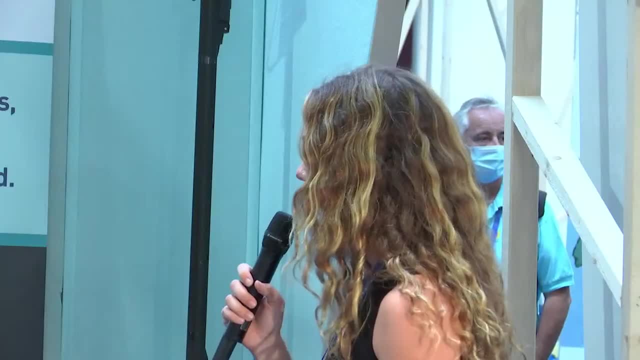 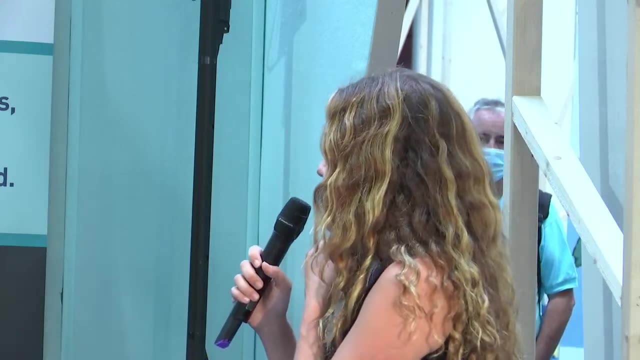 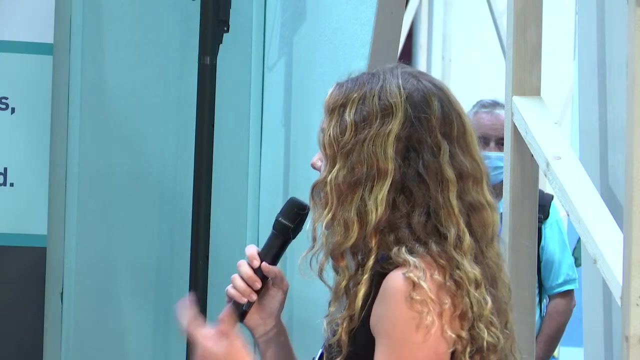 the taking. They're kind of just rocks, just sitting there like dead potatoes. Is that true? And are they just down there for the taking? and they say this process is relatively sustainable? Can there be a sustainable way to mine these nodules And what? 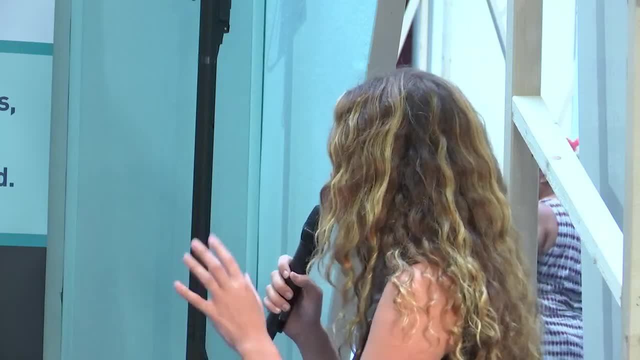 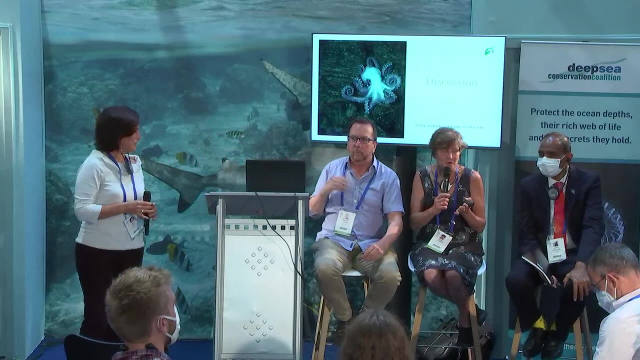 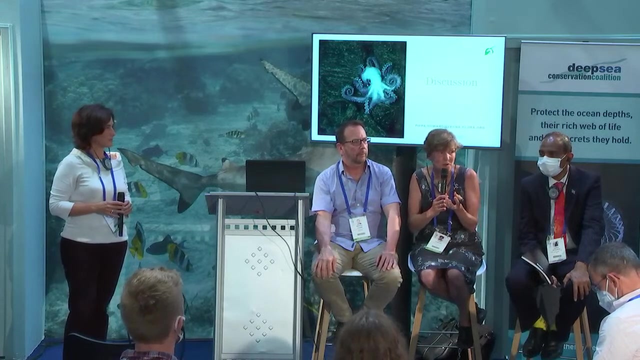 What will it actually do to these ecosystems? I know you mentioned a little bit beforehand, but specifically on that, Thank you. Thanks, Vasa, I'll. I'll respond to that. So no, they're not inert systems. They are. they are substrates for very complex ecosystems and they may be microbes. they 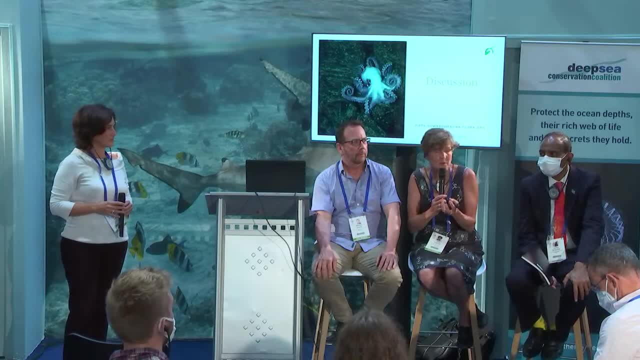 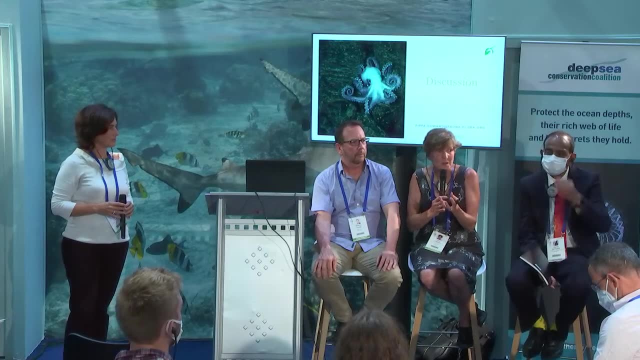 may be bacteria, they may be, you know, very tiny, We can't see them, but they're playing a fundamental role in the whole ecosystem function of of our oceans. Um, Removing them, Removing those, those fundamental processes, actually from from from our oceans. 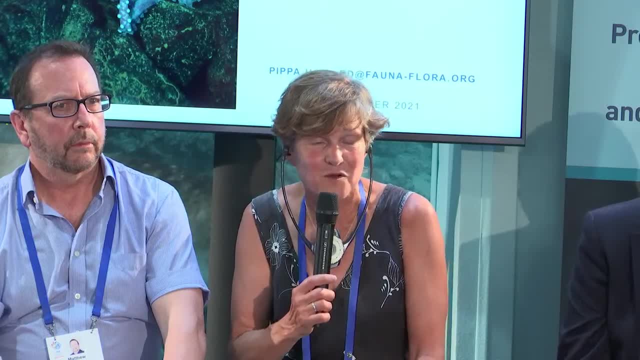 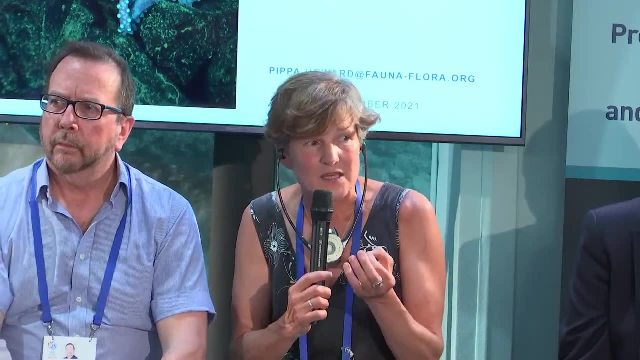 Um, There has been a statement that it's like plucking golf balls off a driving range, which kind of just says it all, doesn't it? And um, so no, the, the, the implications are very, um, are very serious, but also we. 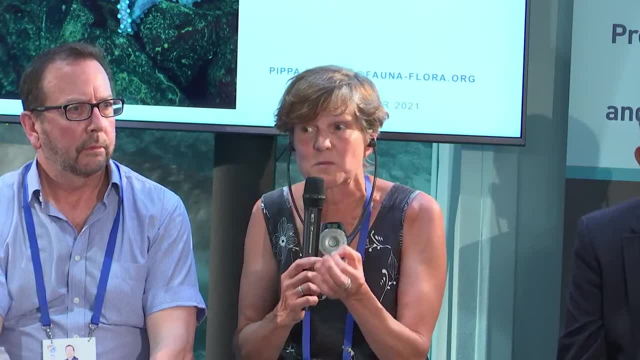 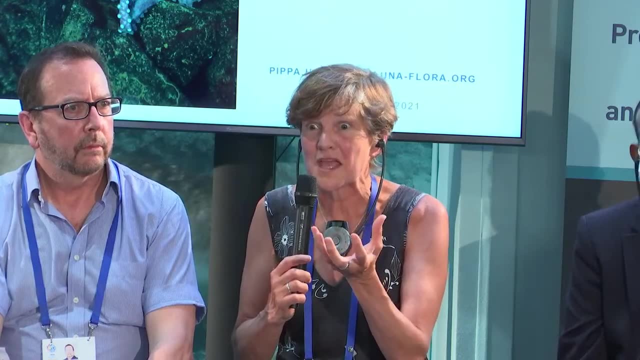 don't really understand this: the role that those microbes are playing in in the regulation of trace metals, of nutrients, of of the whole ecosystem. Yeah, Because the large um chemical composition of our oceans that allows life to take place. 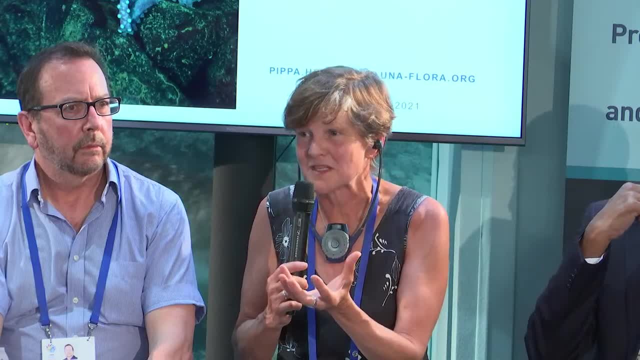 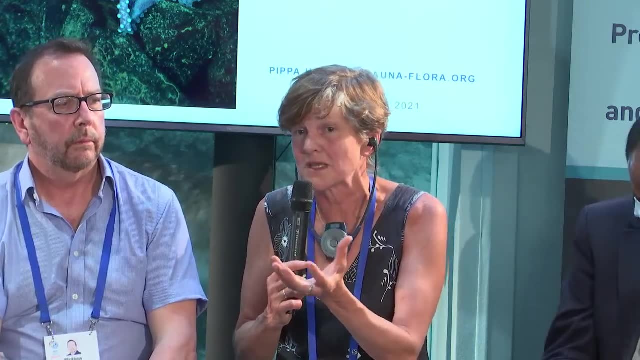 in the first place. So, um, one likening I've said, and without being too, too dramatic, is that that actually using these polymetallic nodules would be like you you making cement out of coral reef systems. you know, it's just, it's that, it's that type of analogy and and it would be. 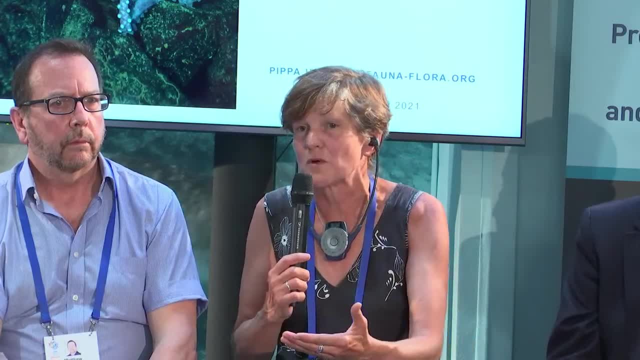 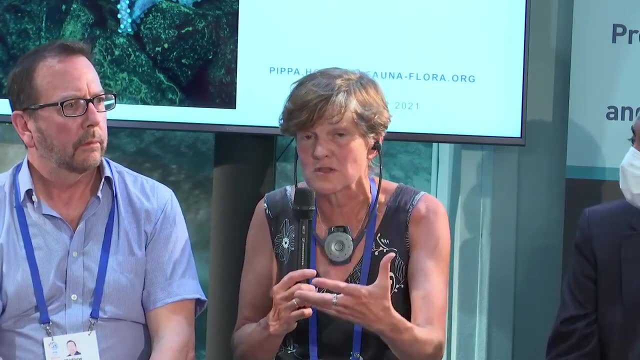 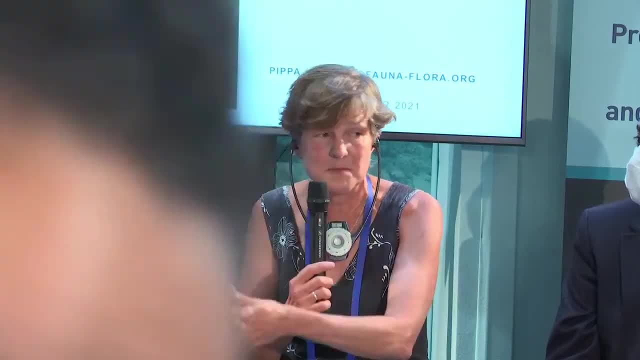 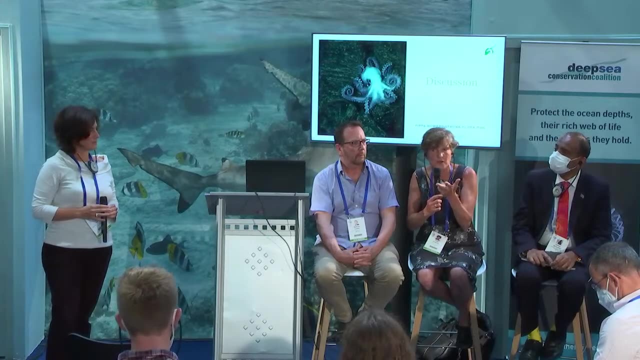 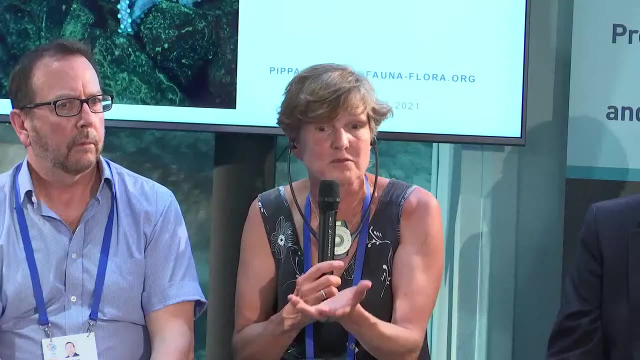 But the clarity of knowledge now is that, as Matt said, impacts are irreversible. they're very long term. you can't restore or offset these. so the application of the mitigation hierarchy that you would apply in any sort of terrestrial mining situation just does not apply in the ocean. 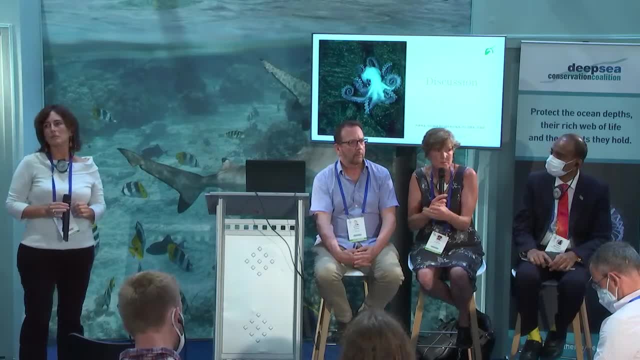 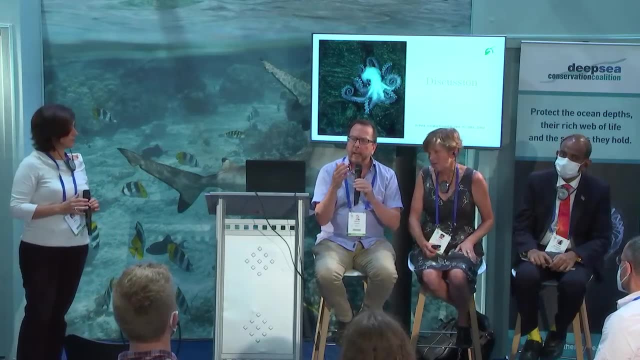 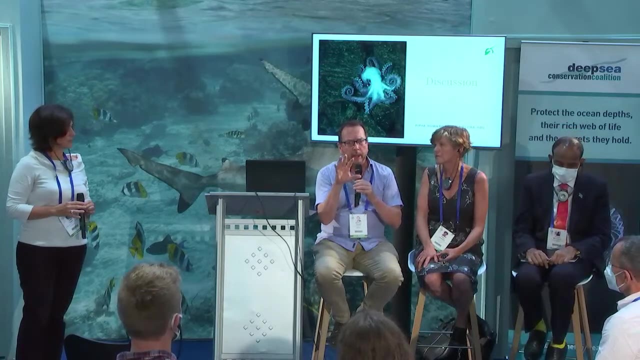 These are permanent geological time frames that we're talking about in terms of the impacts. If I could just add to what Pip is saying, this is another issue in relation to the reform of the ISA that we're calling on because there is language in the Law of the Sea Convention, in Article 145,. 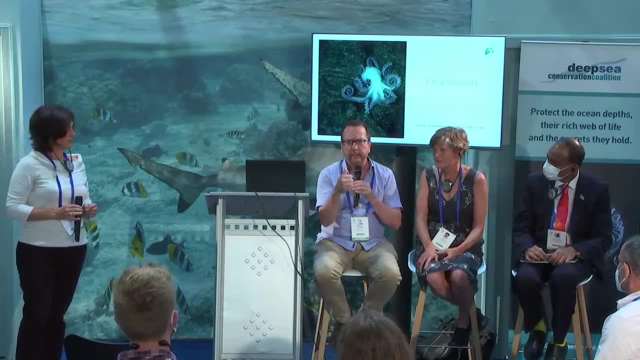 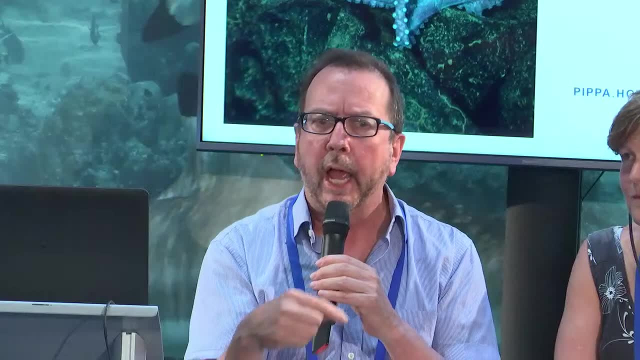 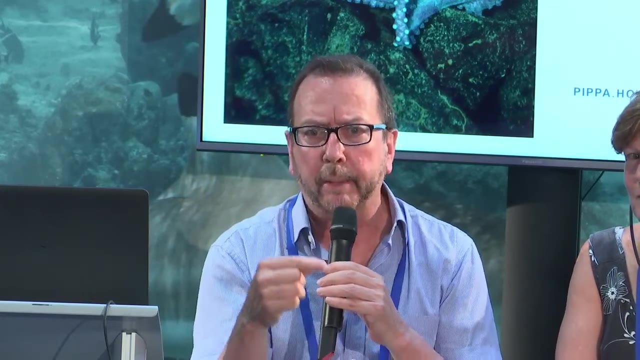 which is part of the seabed mining provisions. that says that the ISA must ensure effective protection of the marine environment from harmful effects of the sea. This means that the marine environment must be protected from harmful effects of mining activities and must prevent damage to the flora and fauna of the marine environment. 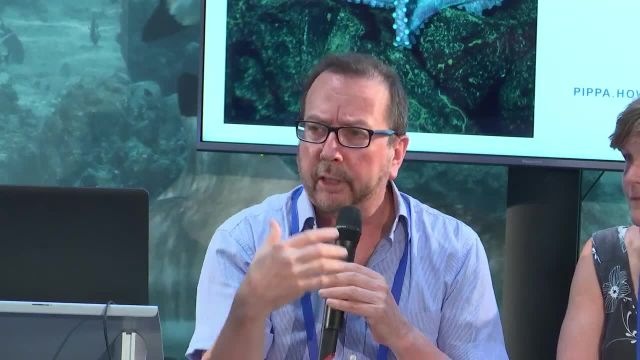 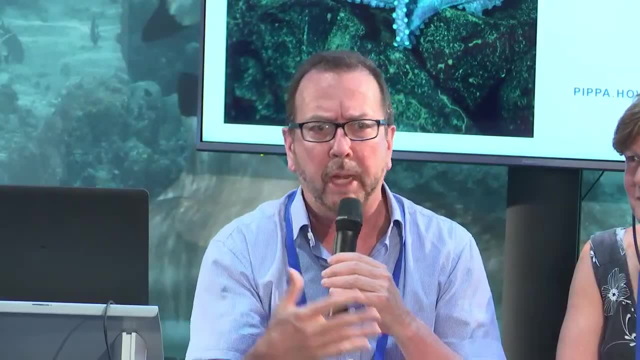 And that was back in the 70s. they negotiated this when they basically were only looking at the nodules and basically the view of that particular part of the world. the deep abyssal plains was. it was an area, a vast area of rocks and mud, with maybe a few worms crawling around in it. but not much else. Fast forward to 2021 and the scientists are saying: this is one of the most diverse areas of the deep sea and there will be significant damage to biodiversity as a result. It may not be high in abundance in terms of the actual numbers of animals there. 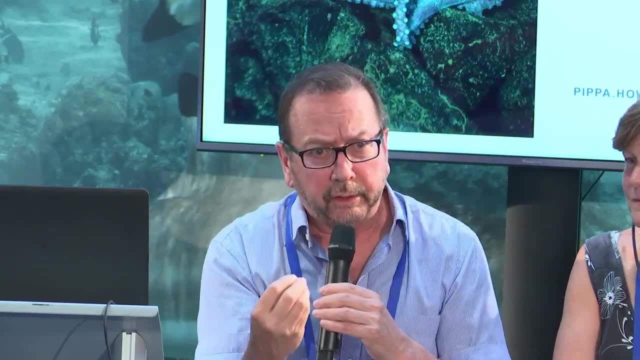 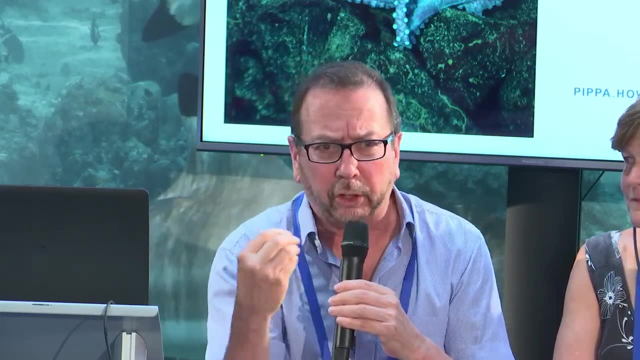 but it's a highly diverse ecosystem, And so one of the debates at the International Seabed Authority is: well, you know, how can we bend the rules so we can get around this Article 145 and say we're just going to go ahead and start mining anyway? 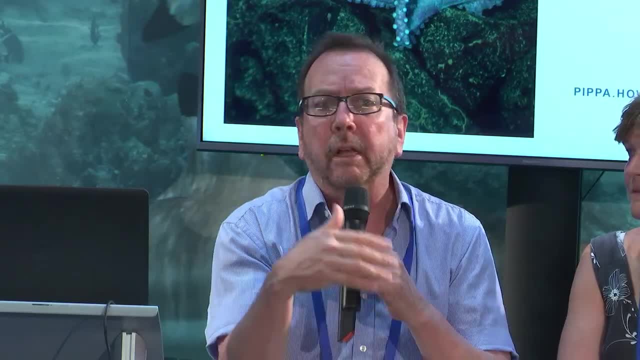 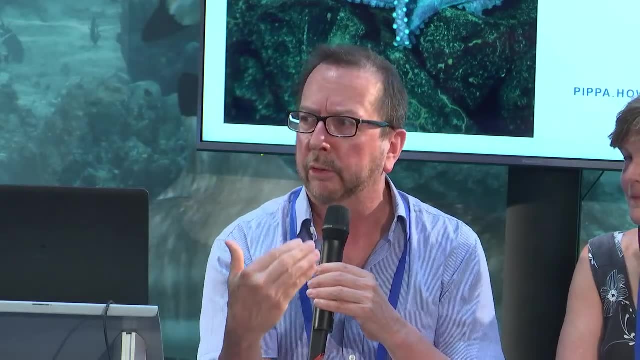 and we'll call the damage to the marine environment and we'll call it acceptable damage or okay damage. And again, when you look at the scale of these operations, you realize it's simply not possible to do so. So we do have tools, legal tools, 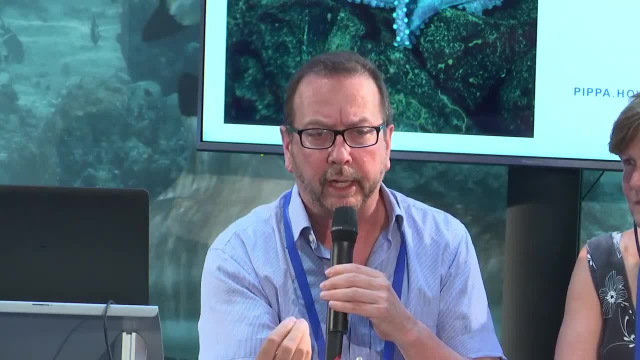 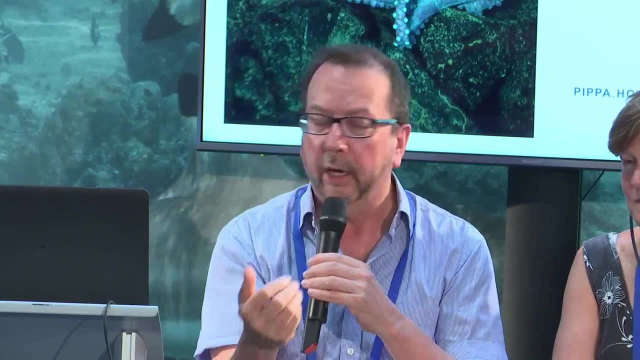 to push back on what governments are trying to negotiate at the ISA, but it's ultimately going to be a political decision And that's where we really need the help from organizations here, and you know through voting yes on Motion 69,. 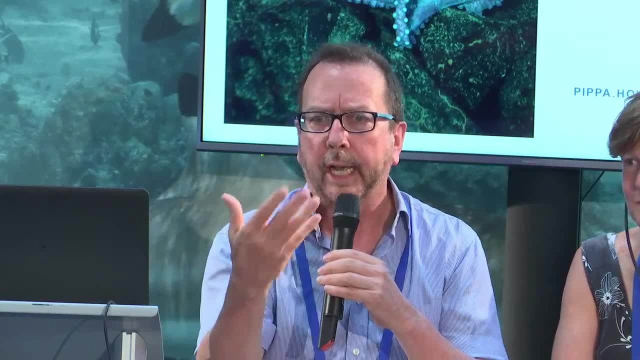 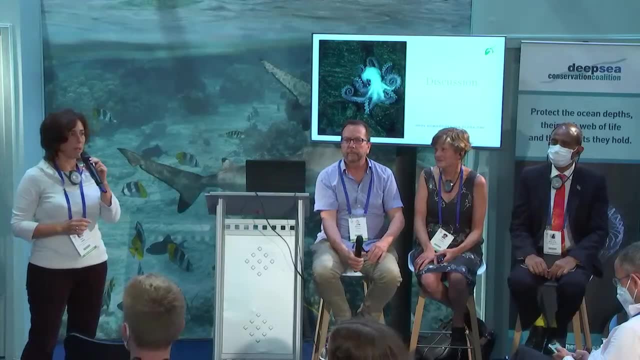 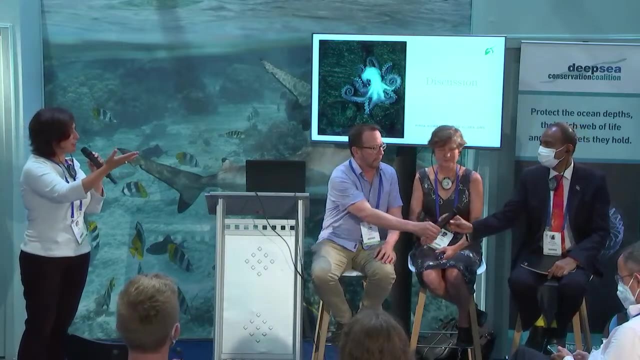 and then pursuing this issue, pushing this ahead with this issue and maybe at another forum. Thank you, Matt. If there are no other questions from the floor, I might pose a question myself to Permanent Secretary Wycliffe. I heard you speak earlier on in a session, earlier at the Nature Business Hub. 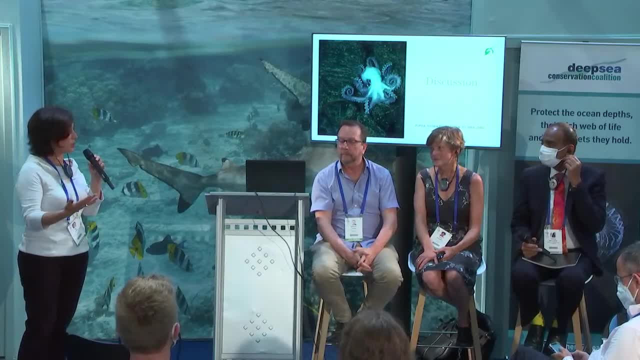 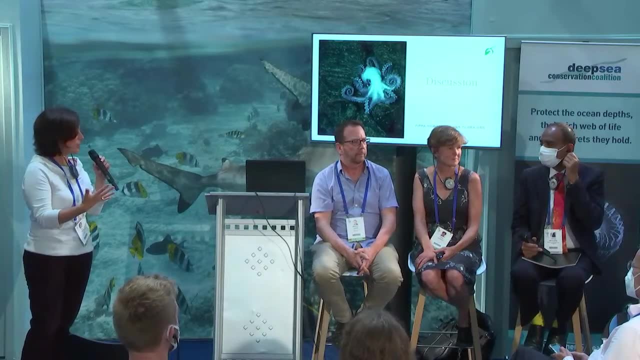 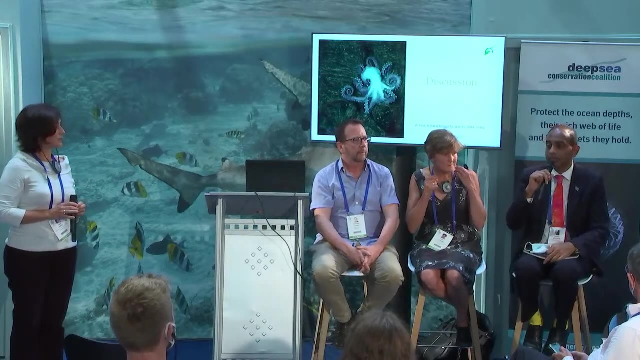 about the importance of working with companies as well on solutions, And I wonder if Fiji has any innovative ideas on that front about how that might look in this context. Thank you, Sean. We've already stepped, taken a couple of steps in that direction. 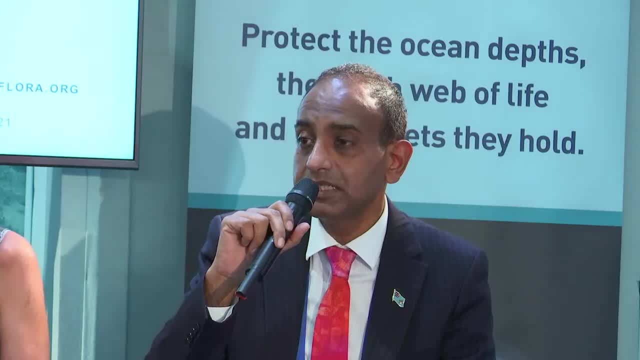 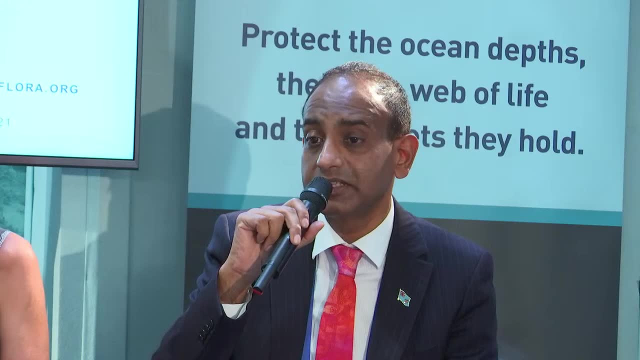 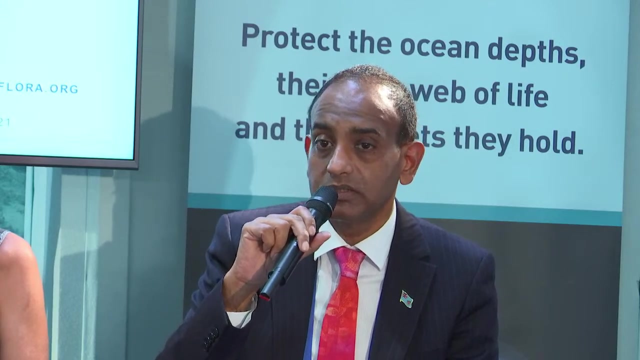 What we've done is not into deep sea yet, but into the within the EZ, a couple of spots where we want to designate them as marine protected areas. Fiji is now forming private sector partnerships with conglomerates and private companies to be able to commercialize those MPAs. 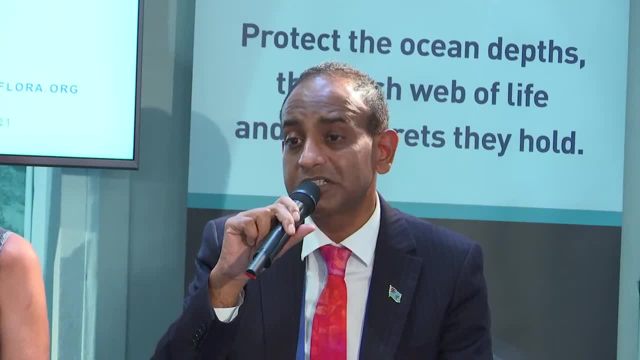 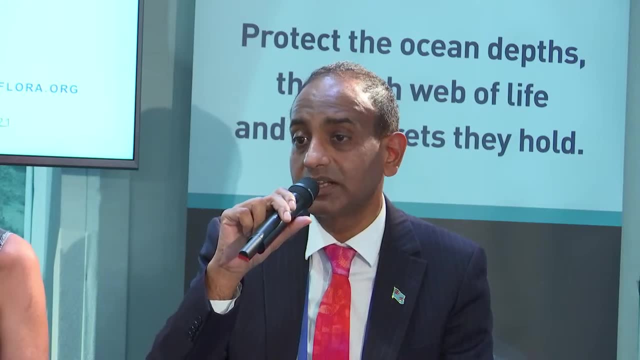 And how we do that is: we all know that marine protected areas have different categories: category 5,, 4,, 3, 2.. So the ones that are not no-go zones, but the ones that are available for entertainment, for diving and things like that, not for fishing. 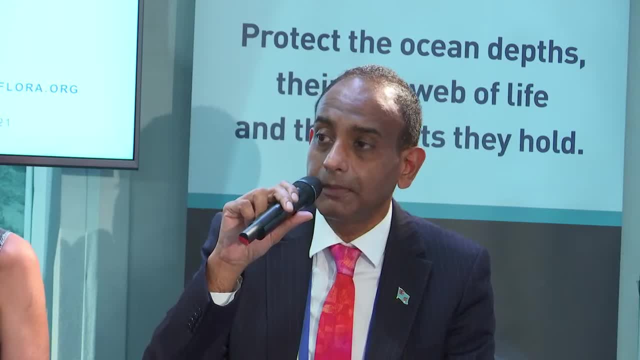 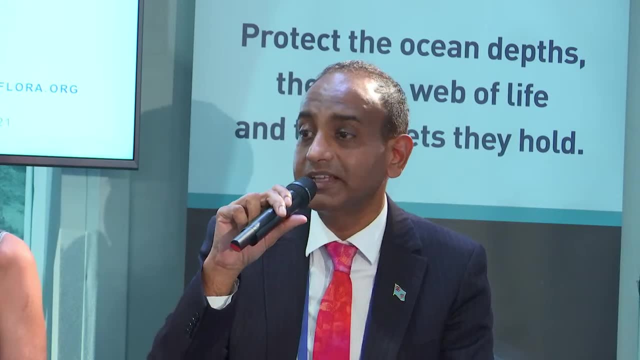 what we've done is we've commercialized them, So these companies would charge a toll for tourists to go and have a look and see them see what's underwater and experience the life underneath for a cost. So that's been a very attractive proposition for companies. 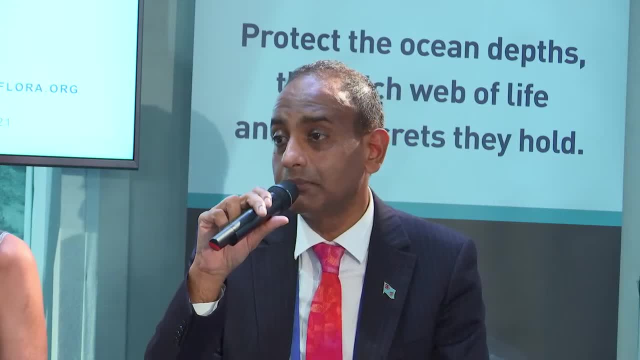 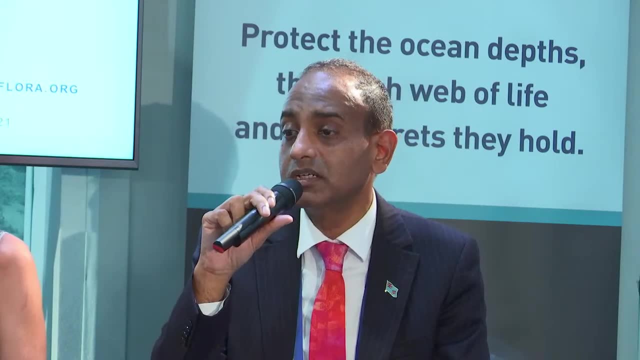 and we've had investors- Asian investors- who put in millions, if not prepared to even do billions, into sea safaris. they call them sea safaris to be able to take underwater experience. I was also thinking when we were talking earlier today. 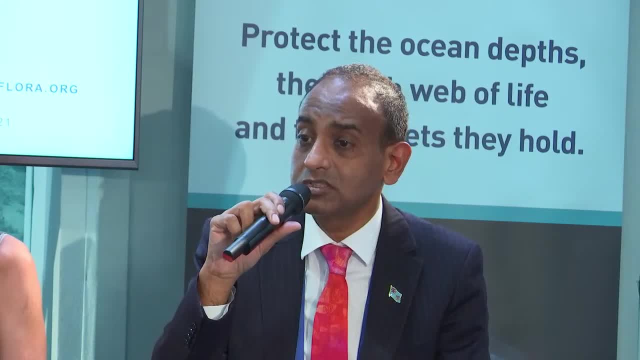 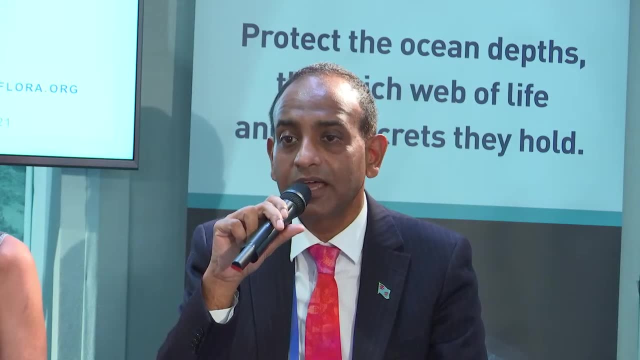 extrapolate that into deep sea as well, not disturbing the ecosystems, but being able to have an opportunity to see what we saw on the video for a few minutes. You know, having an underwater experience and people are prepared to pay costs for that. 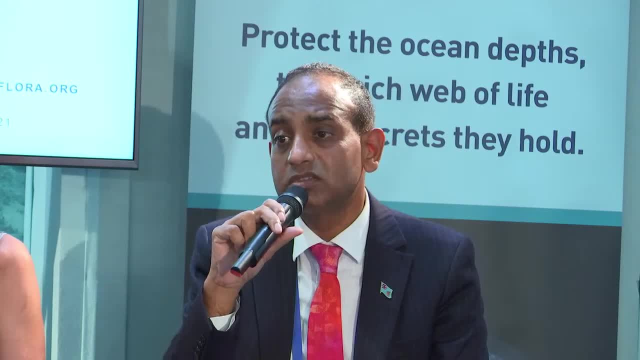 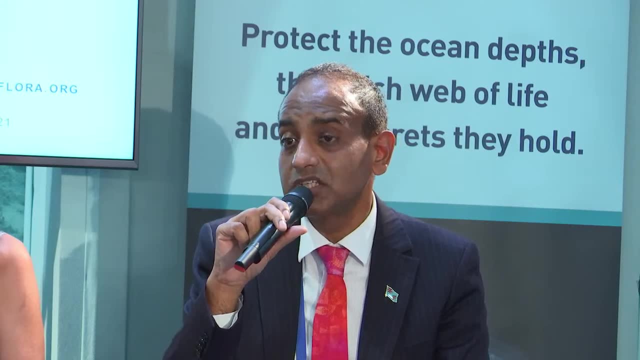 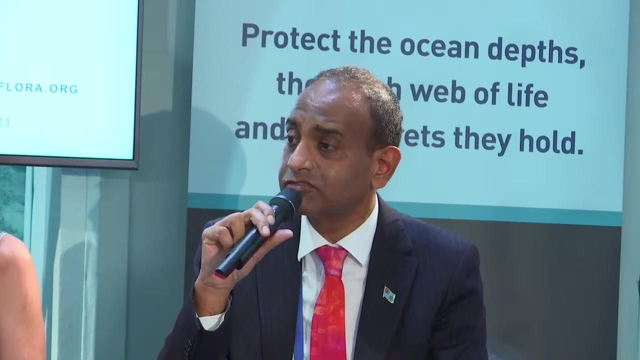 And that raises the awareness and the publicity towards protecting deep sea areas and deep sea spots. So commercialization certainly is an option. There are companies who are prepared to invest. I knew I mean I was discussing in the afternoon with people and they were saying 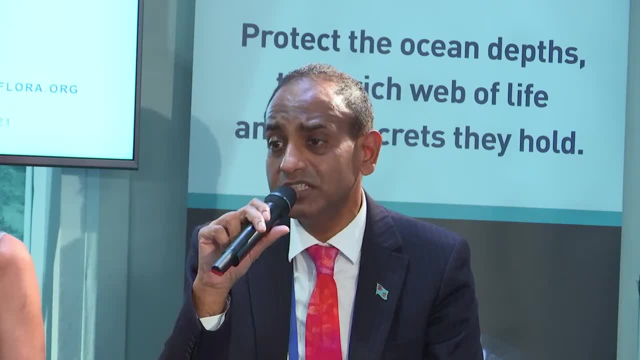 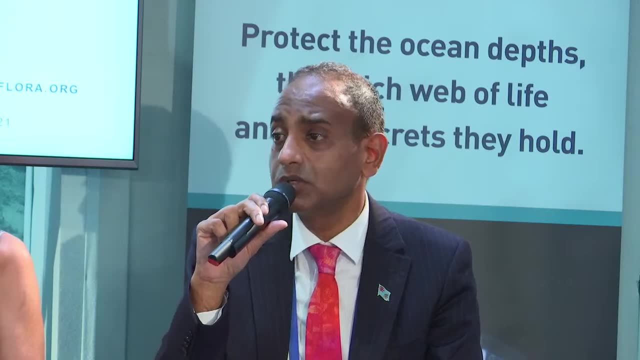 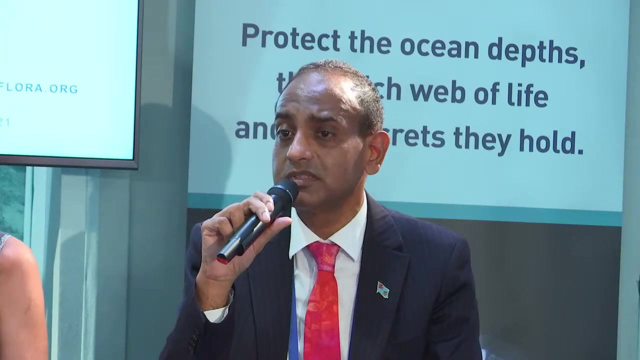 there are efforts underway to be able to reach to private sector groups that are prepared to invest into efforts. So Fiji will continue to do what we're doing: not just commercializing, but also get private sector partnerships being able to build nature-based solutions. 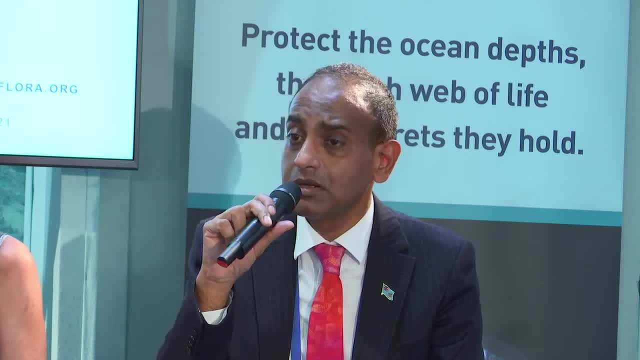 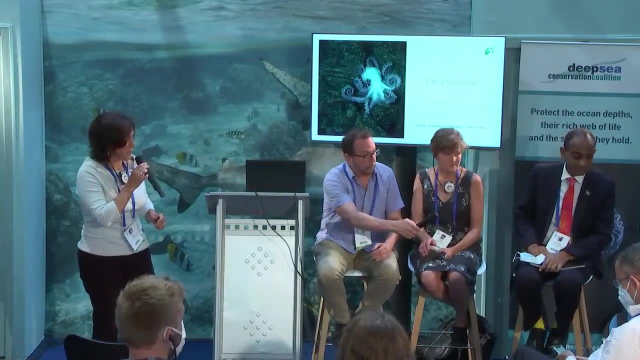 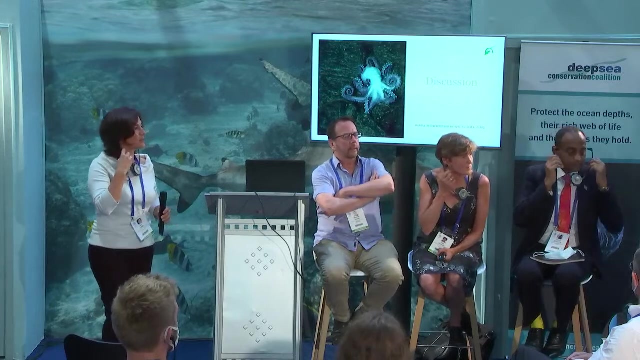 so that these effects are not just put into adaptation but also mitigate in the long term. Thank you, And maybe hand the microphone to Farah, who is also with the DSCC working on this front. Oh, but yeah, so well I. 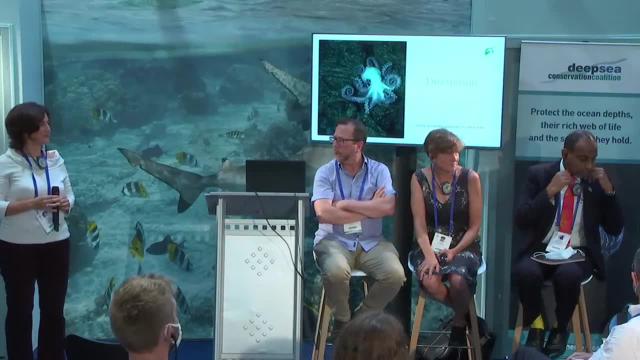 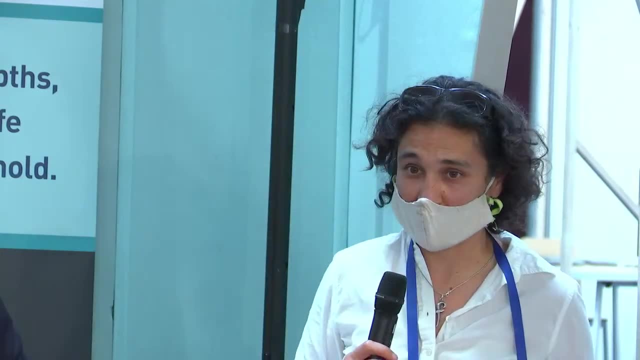 so there's two things that strike me. One is the clock is ticking. Obviously, as we've heard, we know that we have a limited time, less than two years, to stop this industry from starting. And the other thing is we've heard a lot about social license. 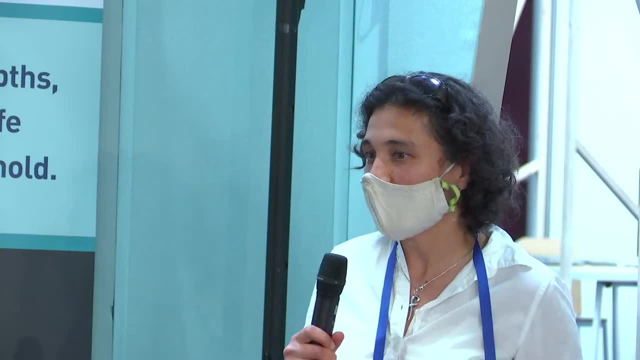 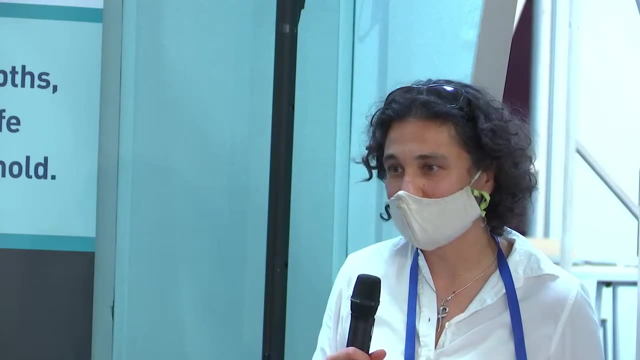 and clearly there is no social license to mine the deep sea. We know that within the Deep Sea Conservation Coalition we have close to 100 members from around the world, all different organizations. We know that the fishing sector, for example. they are expressing opposition to deep sea mining. 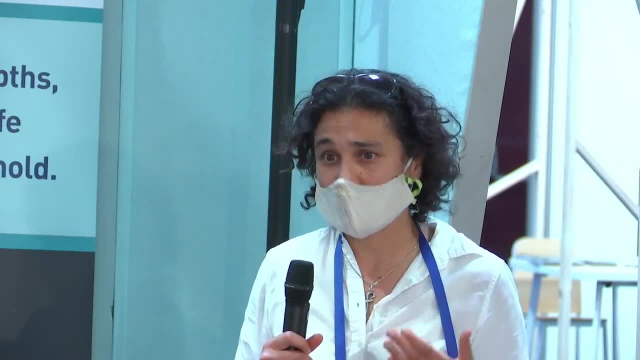 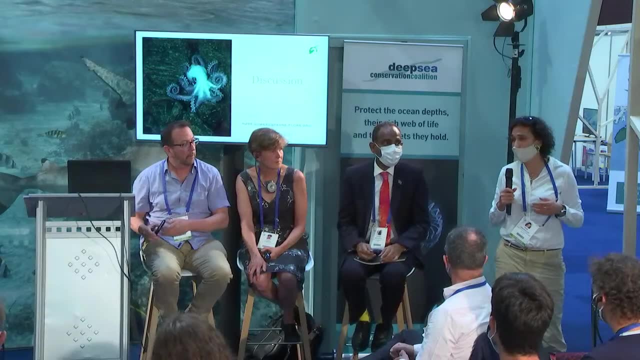 For example, the EU advisory councils have come out and said that they're concerned about deep sea mining and they support a moratorium. And we've heard from the International Poland Line Foundation They support a moratorium on deep sea mining And there's a list. 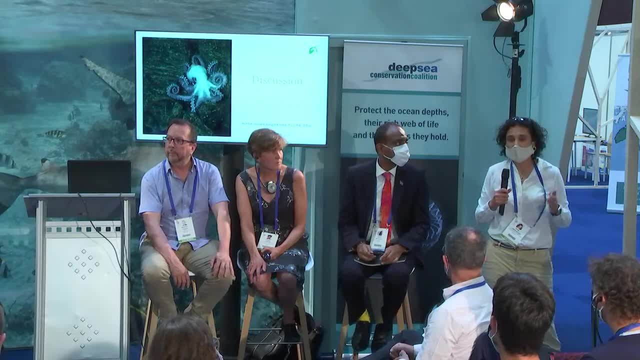 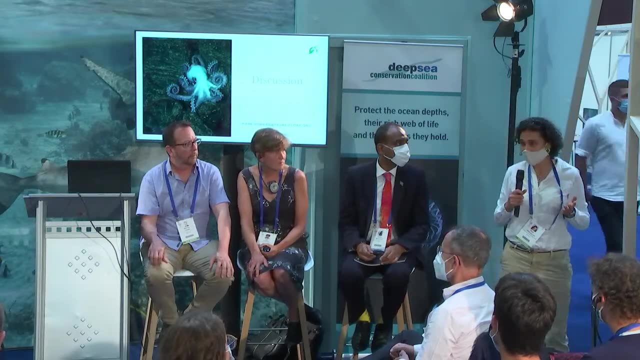 which you can see on our website, savethehighseasorg, of all the entities that are opposed to deep sea mining, But a very important sector- and we heard about it a bit just now- is the business sector right. How does industry feel about deep sea mining? 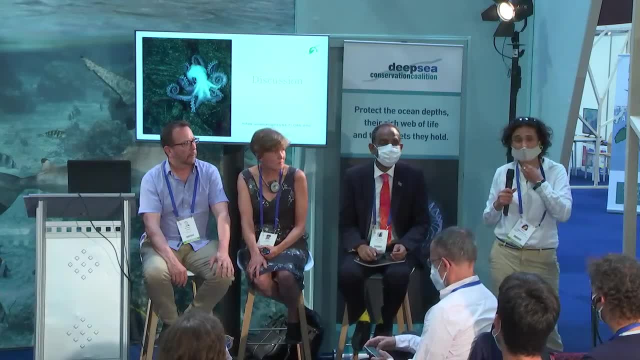 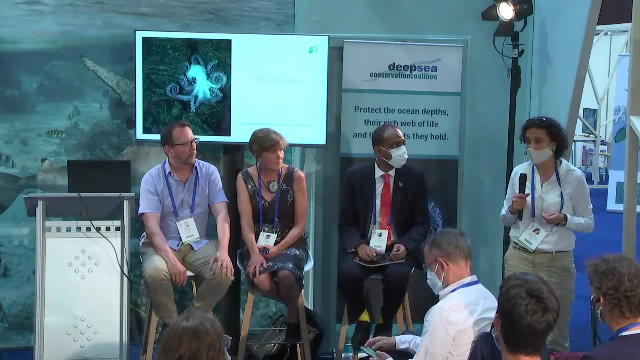 And in fact, there are businesses such as Volvo, BMW, Google, Samsung and, most recently, Philips that have come out and said that they support a moratorium on deep sea mining, recognizing that they- you know that, having the foresight to see, 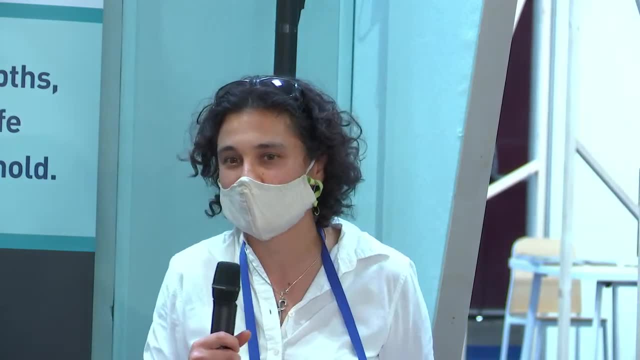 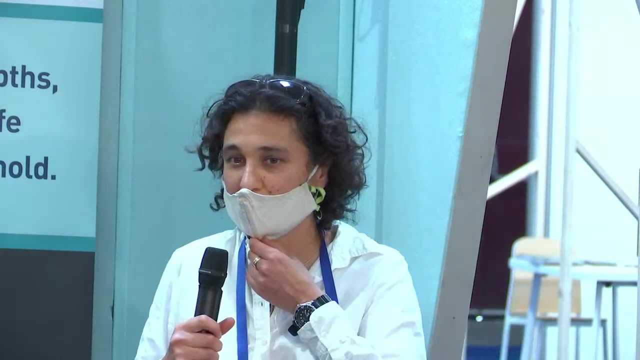 that we don't need those metals going forward in our electric vehicle technology, And they've also pledged not to source minerals from the sea into the deep ocean in their products. So we're seeing that this social license is not there across all sectors, from fisheries to businesses. 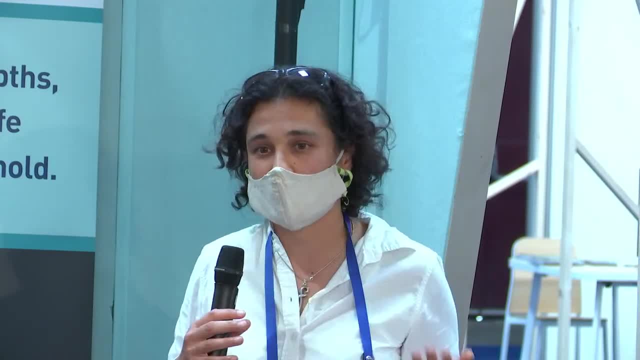 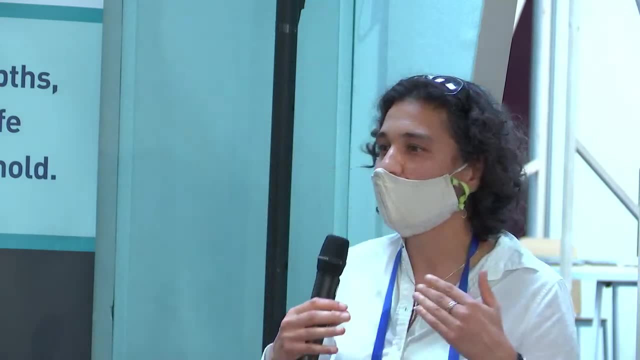 from the civil society and even from the people that represent us, such as the European Parliament in where I live, in Europe, And so the question is: how can we amplify that so that our voices are really heard at the International Seabed Authority? 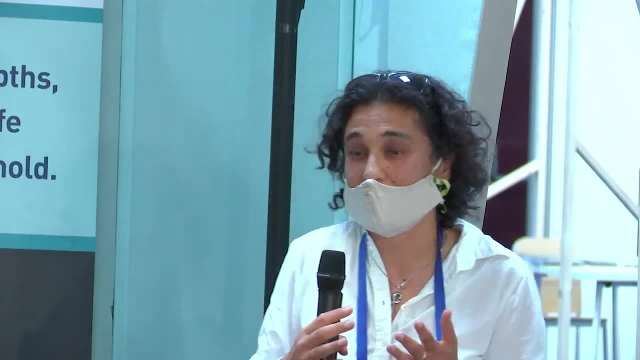 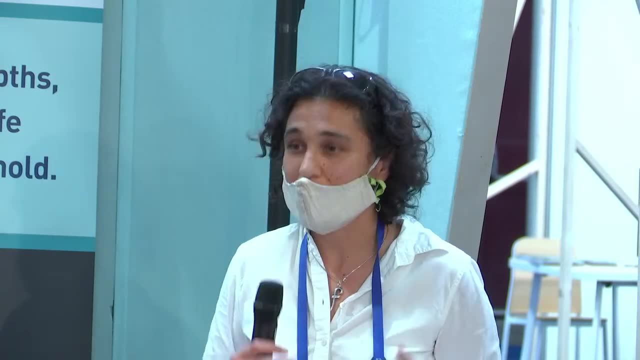 and by our governments, And so one way that I is a suggestion for you perhaps to consider, but it's to join our campaign at defendthedeeporg, and you can also raise your hand in support of a moratorium And also feel free to visit our booth. 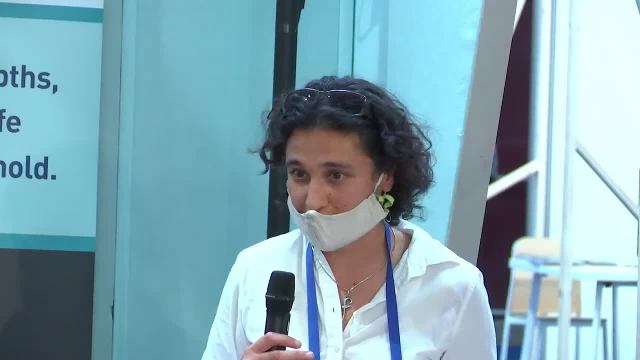 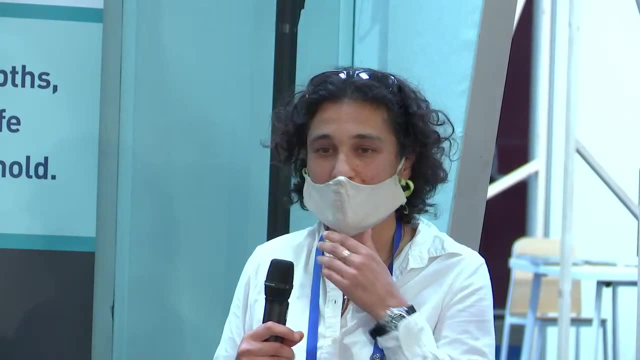 where we have a lot more information also on the ISA, how it's not fit for purpose, on the alternatives to the minerals that they're proposing to mine from the deep sea, and many other information sheets. So I hope we can stop this industry. 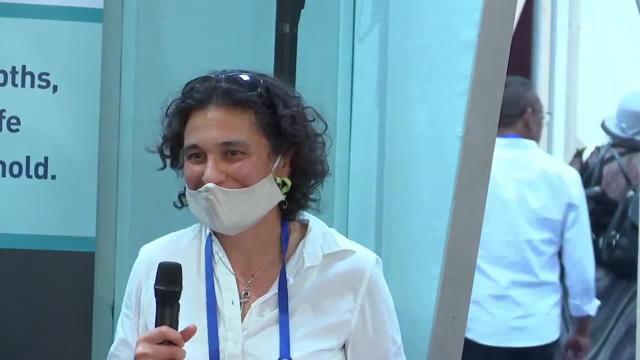 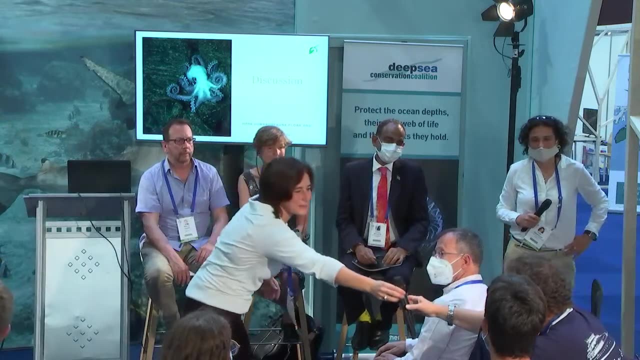 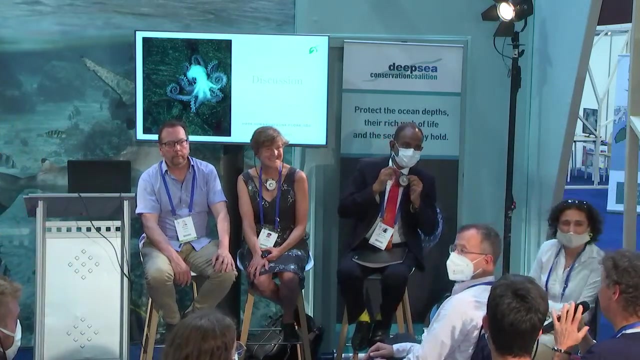 before it starts, And I think that's the good news that we can share here today. So, yes, Thank you, Farah. Yes, a question. I tried this time and I hope I'm not shouting again. Okay, Thank you very much. 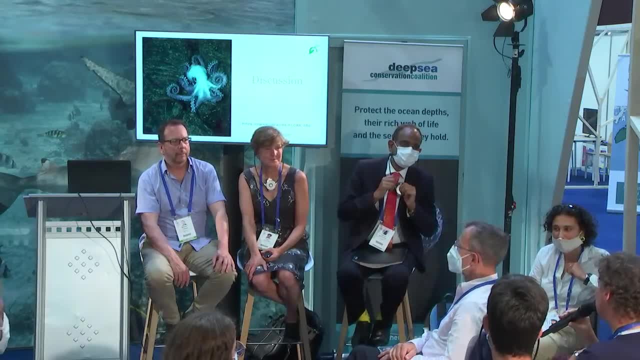 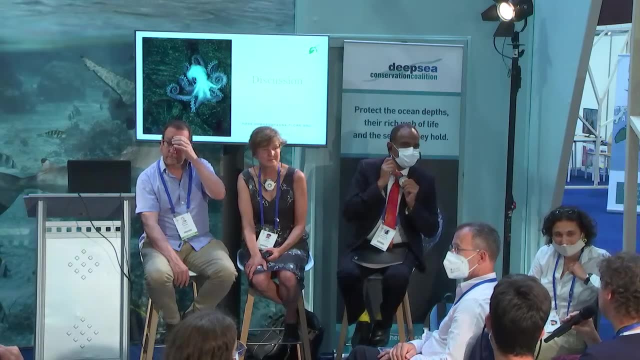 for that interesting presentation. I actually have two questions. My name is Iris Siegler from Shark Project and we'll definitely support that. I wasn't really aware of that moratorium that we have to go forward, but it's definitely something we need to support. 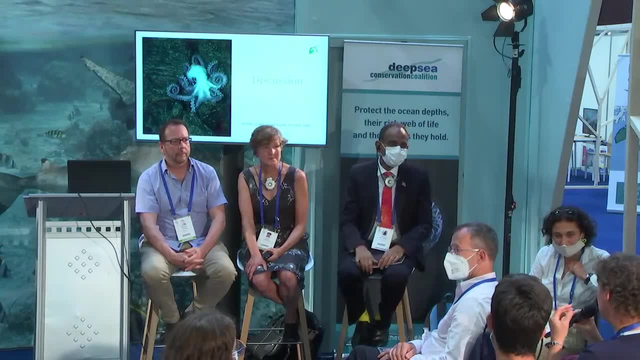 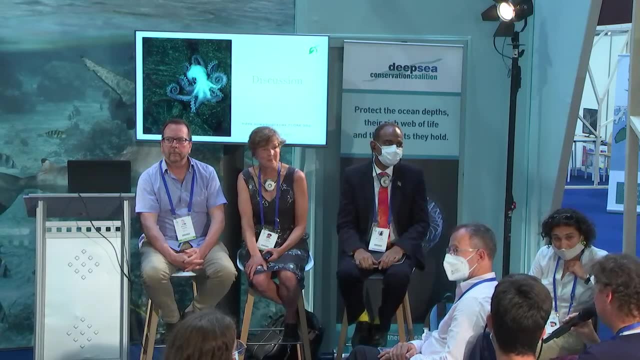 So my question to you would be: do you think that this moratorium, if we have it here at IUCN, vote for 69, is this going to make a difference? Is it going to be powerful enough to really stop it? 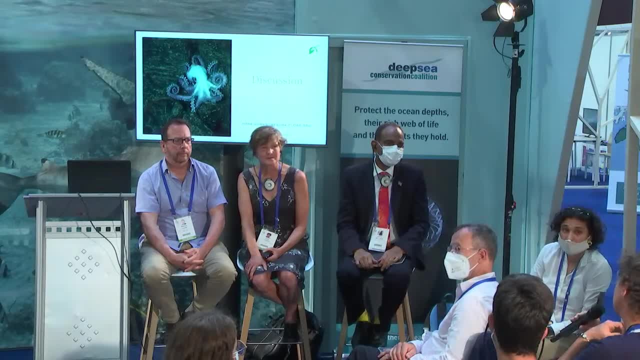 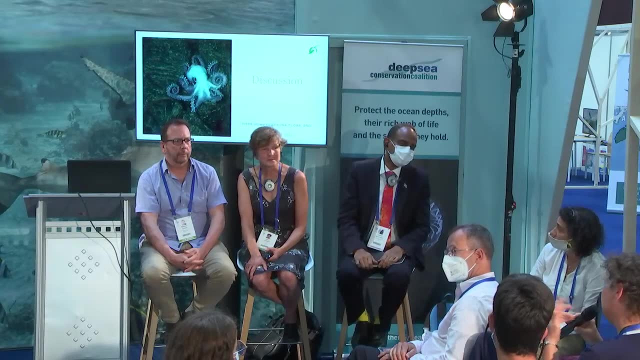 That is the first question, And then I would have a question to Mr Wycliffe. You really impressively showed like Fiji 10, and it's great. I just can't say thank you for that to support that. But would I be interested? 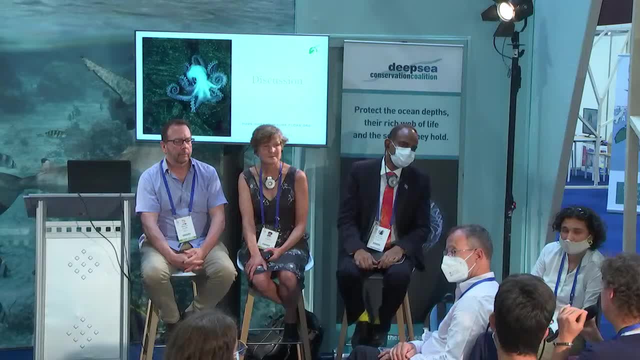 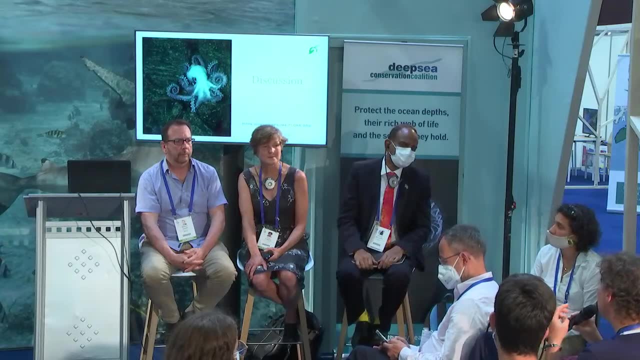 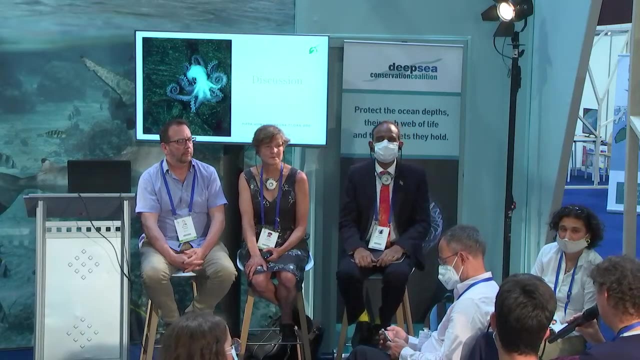 in knowing is, you said, like with marine protected areas, you're also supporting, you're giving away licenses, which is obviously a good way to compensate, But what is your intent of how much of your waters you're going to protect into real no-take zones? 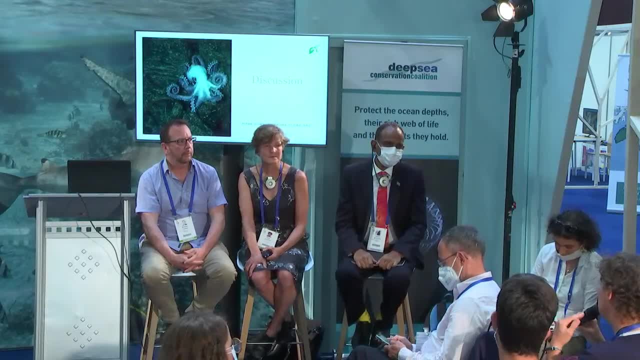 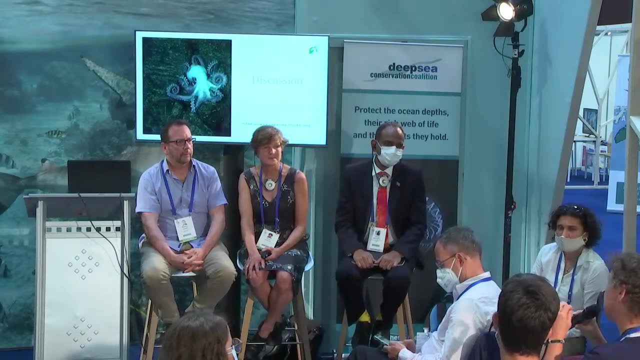 Like no extraction. that's what I mean, because there's a huge debate going on Like: do we talk about 10%? Is it highly protected? Is this strictly protected? Is it no-take? And there's different things circulating. 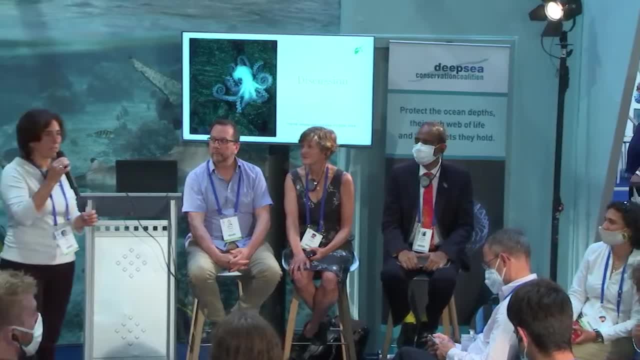 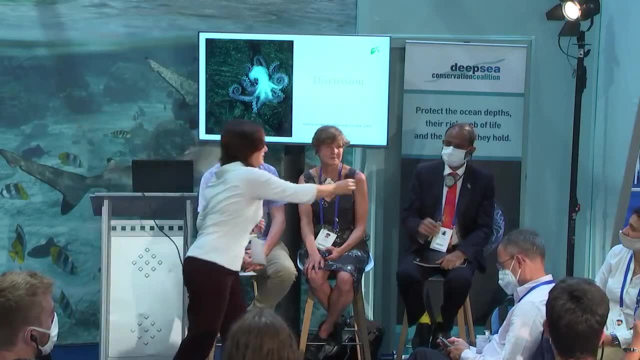 So that sorry for being long Nate. thank you, That's perfect. We'll take the. I'll give the microphone to Mr Wycliffe first to take the second question and we'll come back to the first. Thank you for that question. 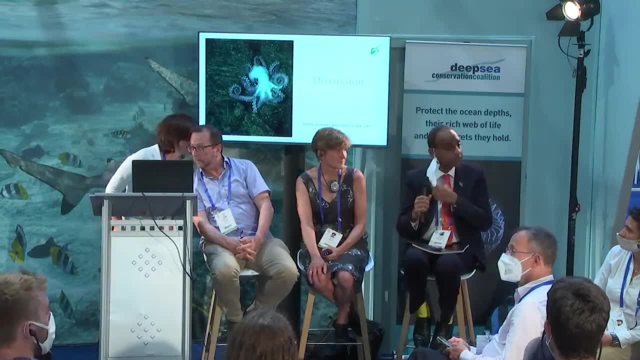 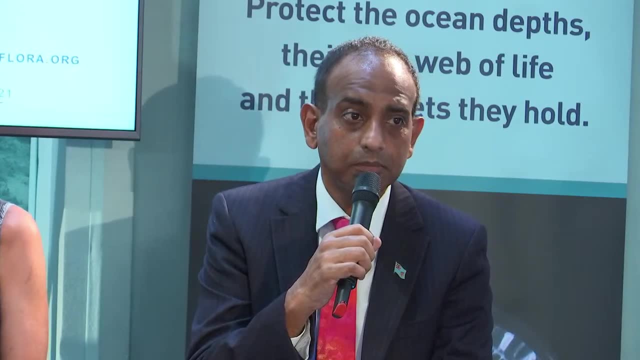 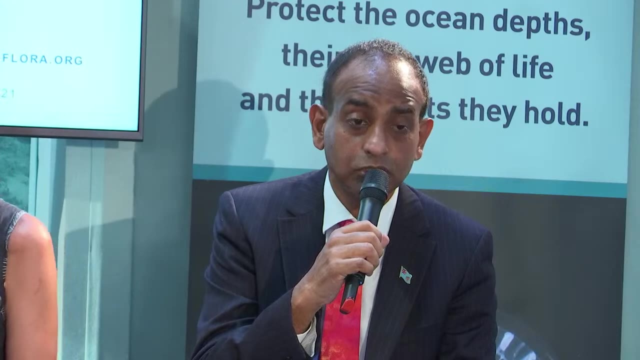 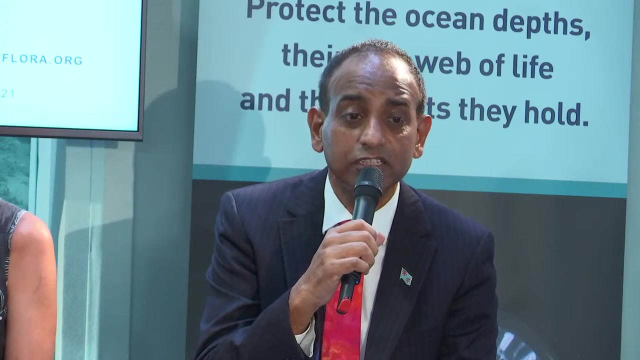 It was a good question too. The way it goes the MPA is being adopted. It's like this: We have taken a stock take of our biodiversity. Our state of the environment report says what's found where, kind of indicatively. 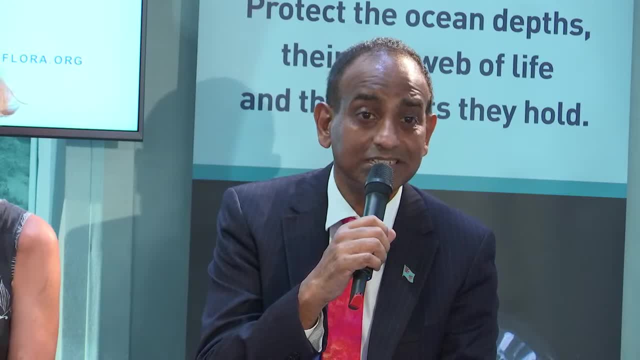 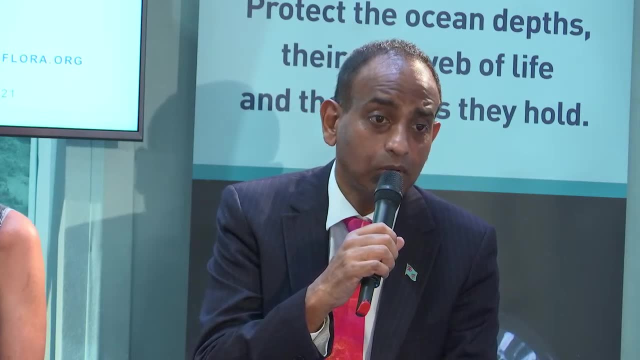 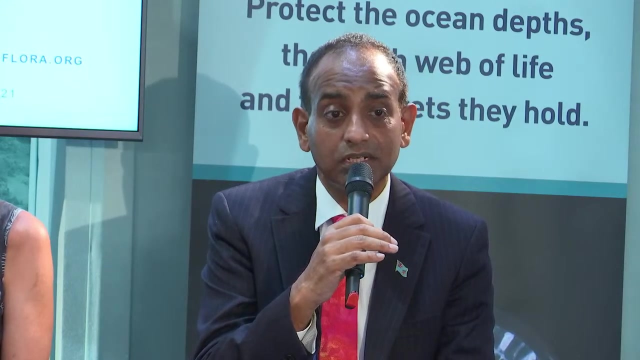 So we don't go by percentage for the sake of it, saying like I put 10% for the warmth is words, and say good, nice things, But we go by how biodiversity is impacted, So the least affected would of course have be categorized accordingly. 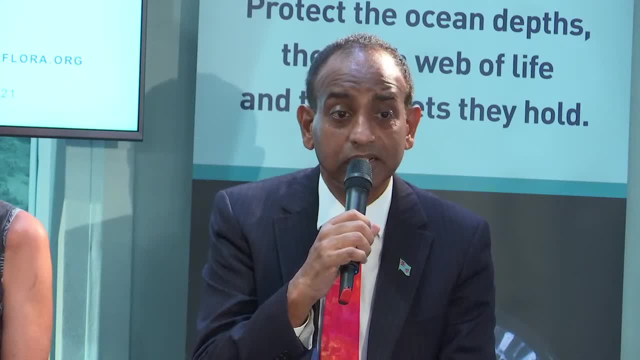 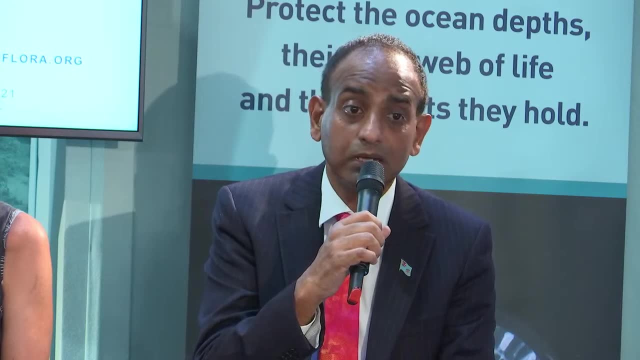 The most affected would be no-take And from what I understand it's not officially done. We have not given licenses yet. The model's just been finalized And it goes through the parliament, And how it goes is about less than 30, 40%. 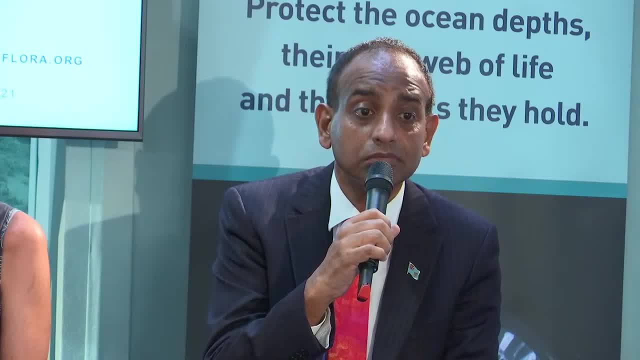 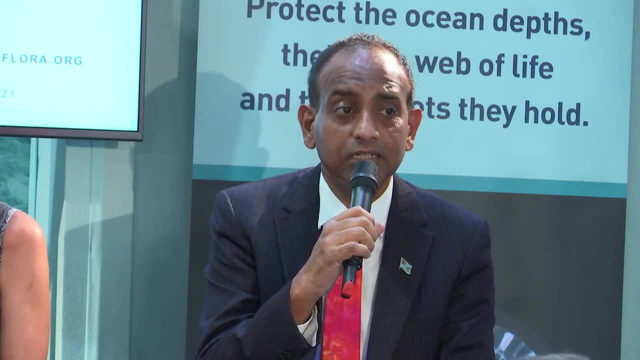 would be a free liberal area to go around doing anything. So the no-take zone is much larger than what you have for leisure, And so we're very conservative in what we do. But for the little spaces that we have we don't give licenses. 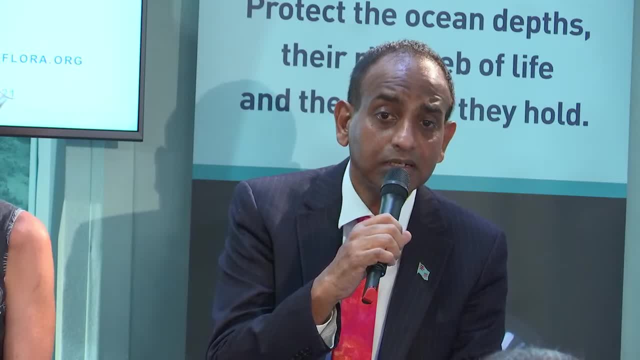 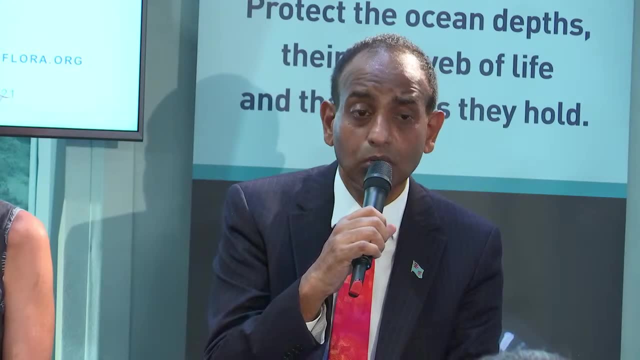 to go do anything inside other than provide studies and education and awareness. So it kind of has several ticks. It provides awareness and education to our local citizenry as well and to the tourists who come, And it boosts ecotourism as a segment. 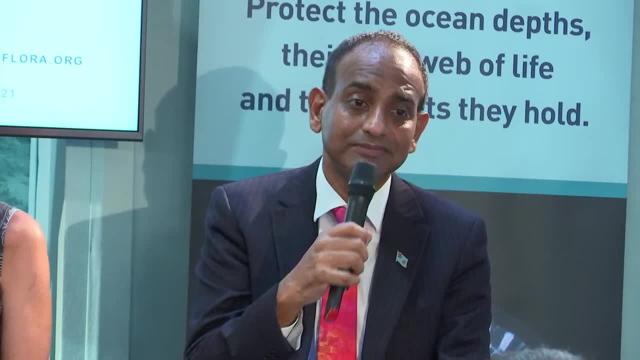 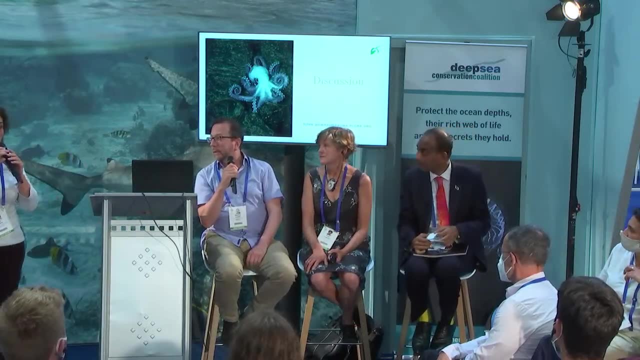 So that's where we stand at the moment. But good question, Thank you. Thank you, And if you would pass the microphone to Matt, The first question was: will this make a difference? Will the yes vote this week make a difference? 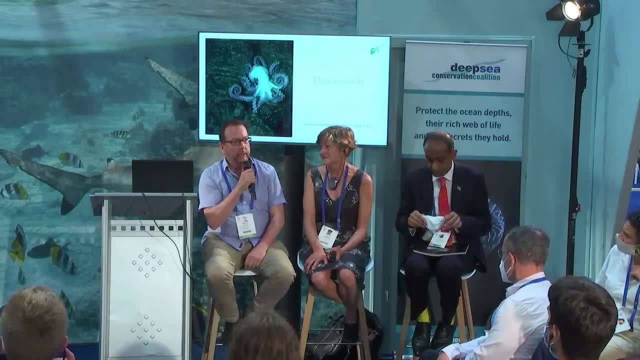 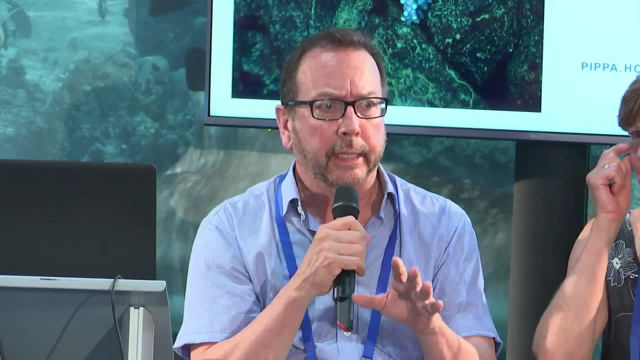 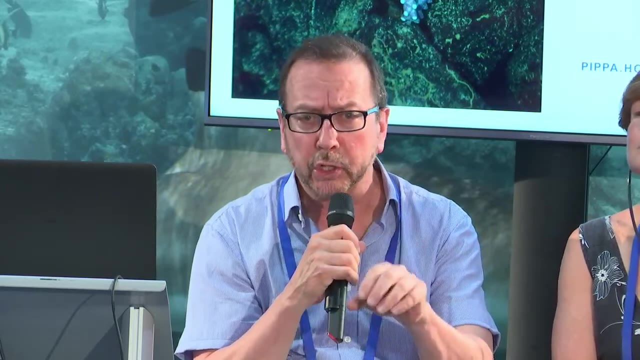 Well, it can, It should And I think it will if we get a strong vote here, Because, again, no country has yet come out and said maybe we need a moratorium at the ISA. There are 167 member nations, And so we've been pushing them. 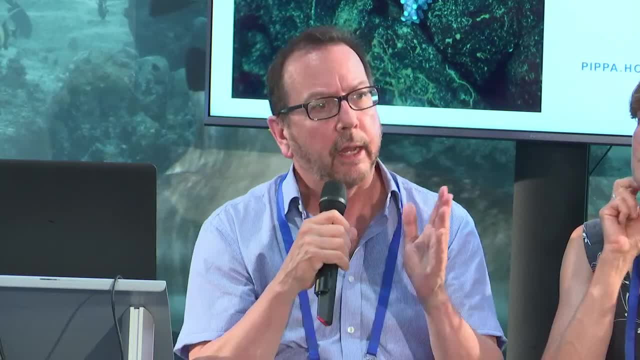 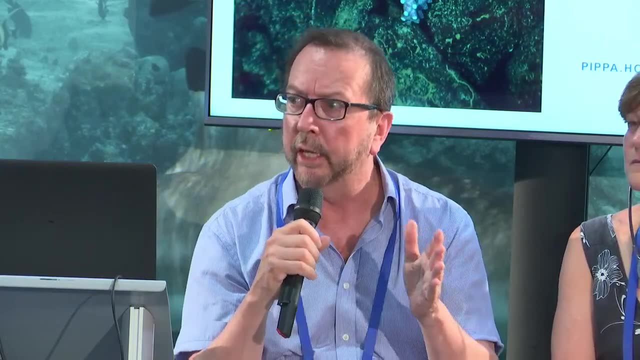 And a lot of them are looking to other countries to go first, And we think that if, for example, some countries come out and vote in support of 69, that already sends a signal to the others that are considering it and may be willing to do so. 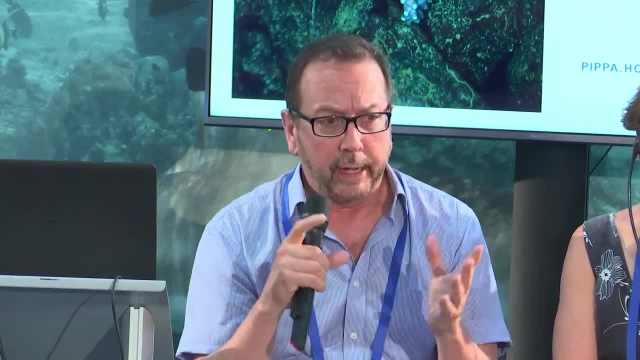 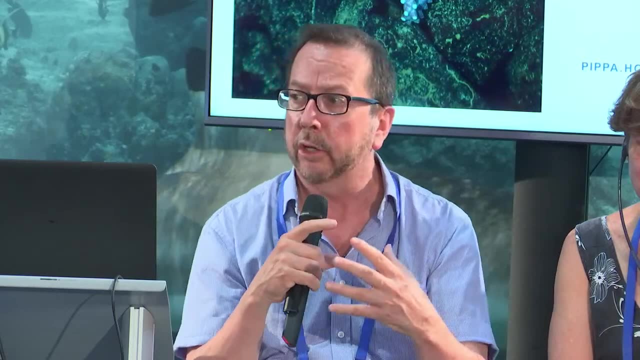 and act as a catalyst to bring together a group of like-minded countries that will then go into the ISA negotiations, as well as the BB&J negotiations and other negotiations, and say, OK, we need to make this happen. But again, the second issue. 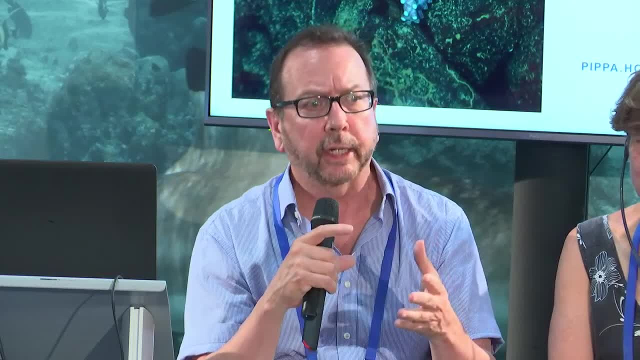 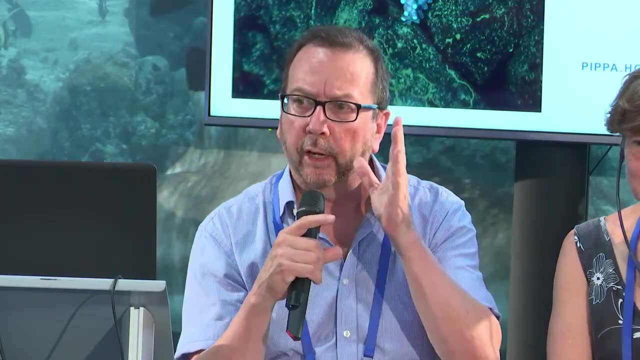 I would emphasize is that, even if this motion loses with the states' parties, if we get a strong vote from civil society, we're going to have to make sure that we're going to have a strong vote from the ISA. So I think that's going to be. 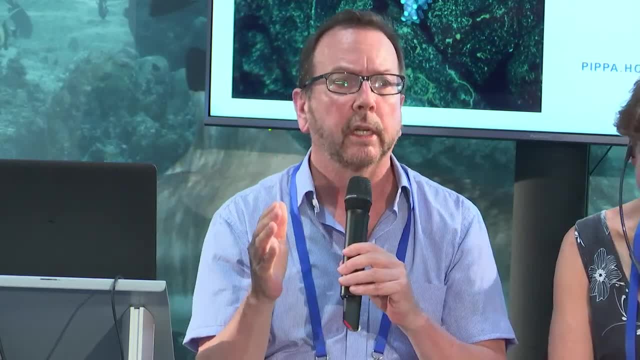 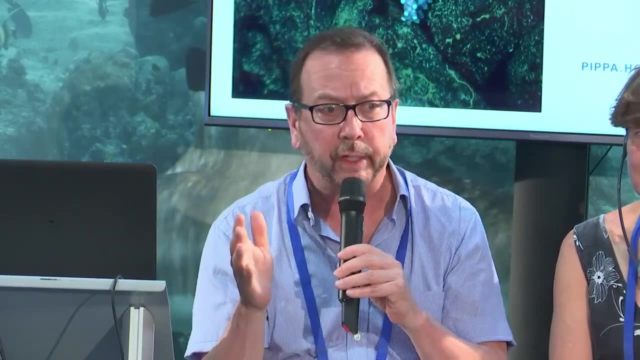 a strong vote from civil society organizations That sends a very strong signal to the member nations of the ISA, individually and collectively, that whoa, wait a minute. it's not just a handful of marine conservation coalitions or even the 91 members. 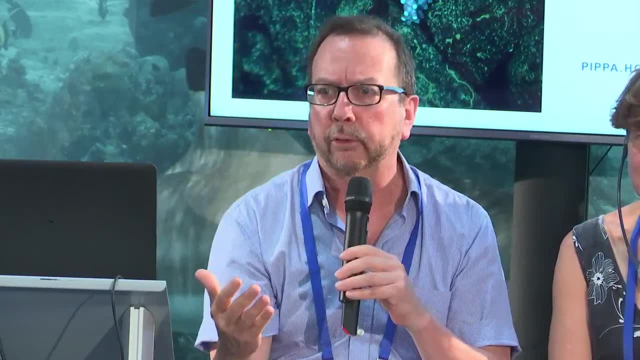 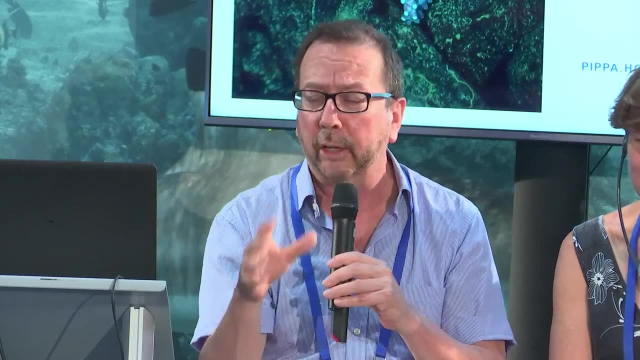 of the SEC, but however many votes we're able to get here at the World Conservation Congress, And that only builds momentum and pressure to put on governments And what we're hearing internally from quite a few governments, in particular EU member states, but also a number. 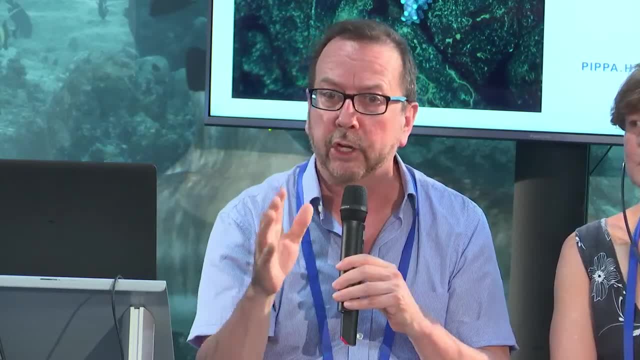 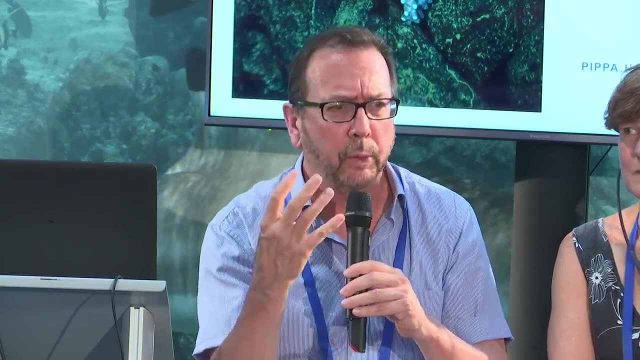 of Latin American states and certainly the 47 states and member nations from Africa that are members of the ISA, that they want to slow this process down. They're starting to grapple with how do we do this, How do we interpret or renegotiate international law? 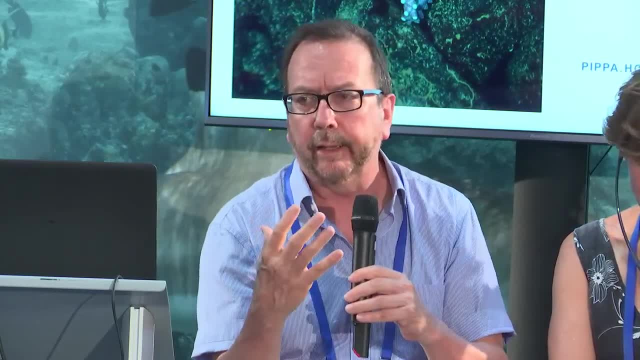 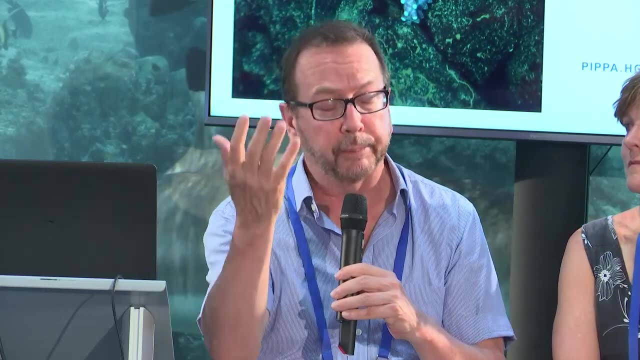 to ensure that we can do this And they can. It's a question of political will And again, I think that the IUCN World Conservation Congress, in adopting 69, could really boost that political will and really bring countries out of the closet. 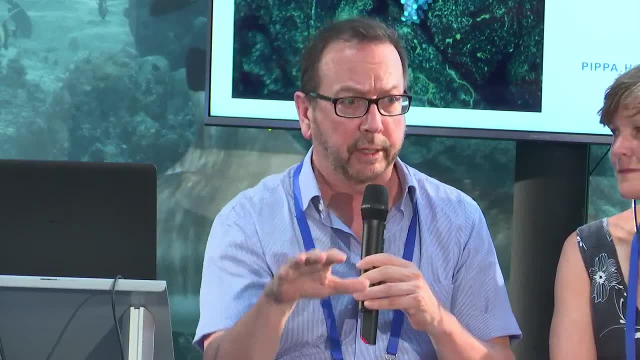 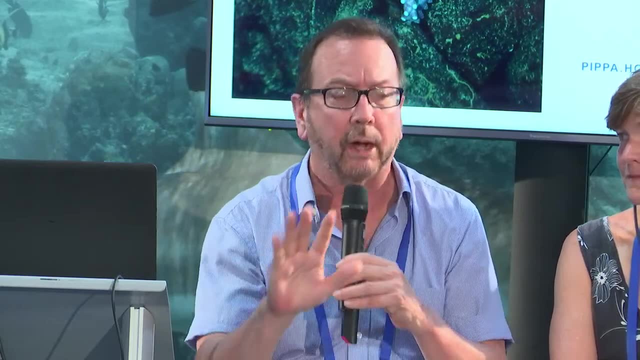 or off the fence on this And be willing to stand up to the countries that do want to mine and say: sorry guys, we're going to have to slow this down. This is a bad move. This is a bad decision. We can't be doing this now. 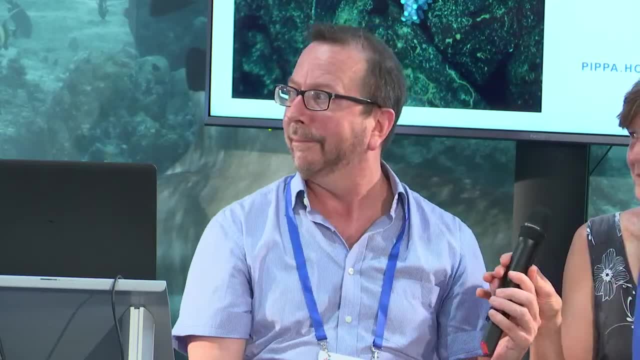 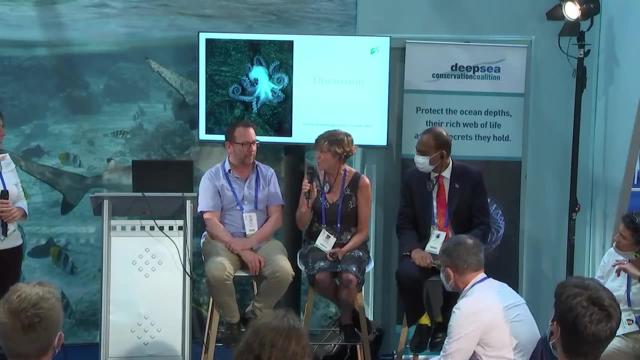 We really need more time to think about what we're doing and reconsider. A very quick final word to Pippa: No, I was just going to say what happens to those who just think it shouldn't happen at all. Should we be delaying this? 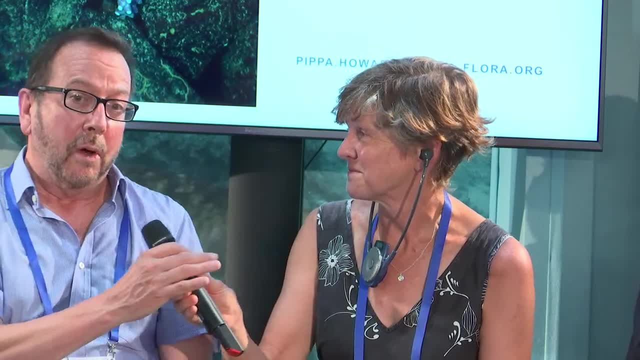 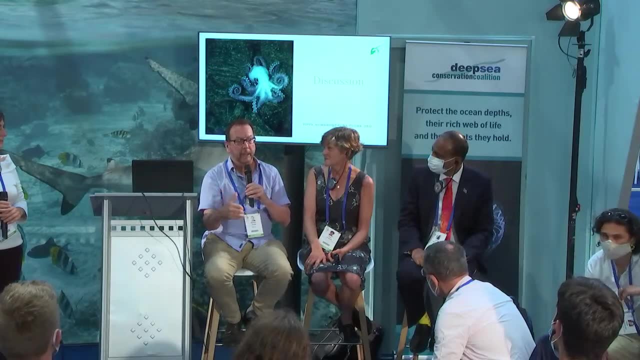 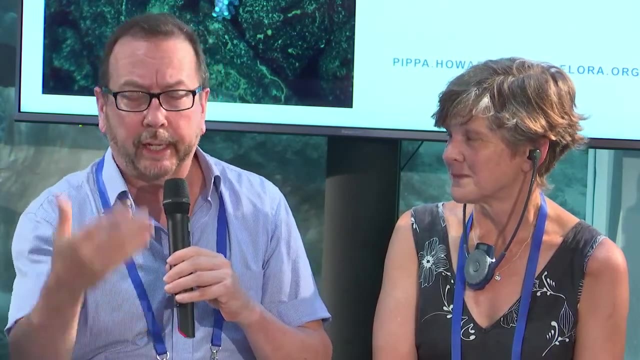 or should it be banned entirely? Well, I would say, if we get a moratorium that gives the space for a serious global conversation about the science, about the regulatory body, about what the world wants to do with its global commons. And I can't help but think. 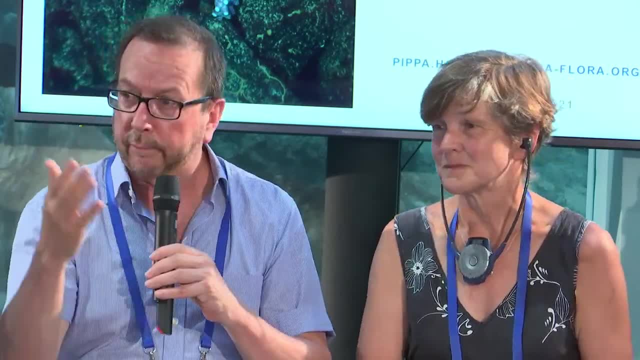 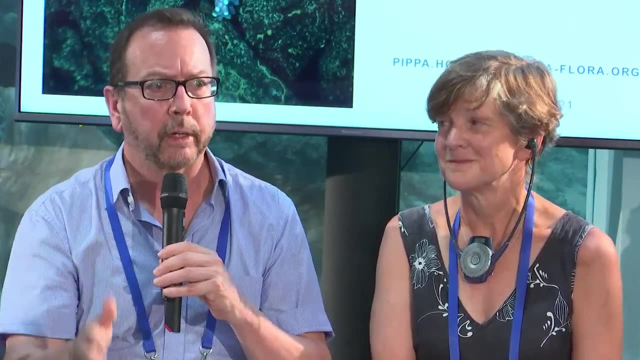 that you know what was it. 30 years ago, France, amongst others, stood up and said during the Antarctic minerals negotiations: no, we're not going to negotiate a regime to open up Antarctica to mining, We're going to set. 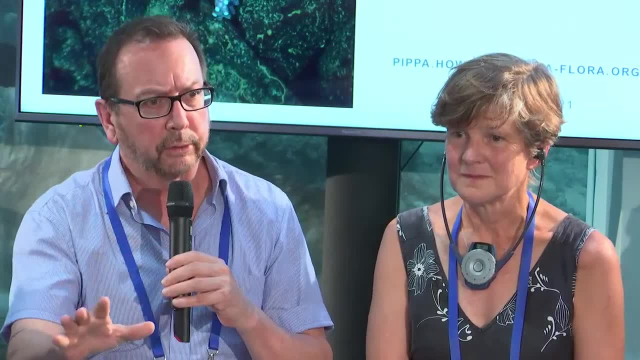 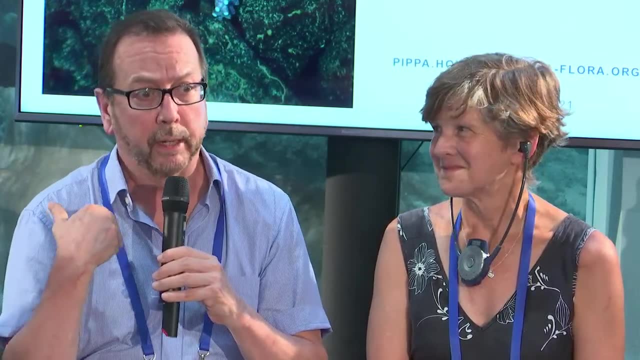 this aside, as a global commons for protection, scientific research, understanding how it influences our planet. The same can be done for the deep sea, And, in fact, from my point of view, that would be a very good outcome of this process. So